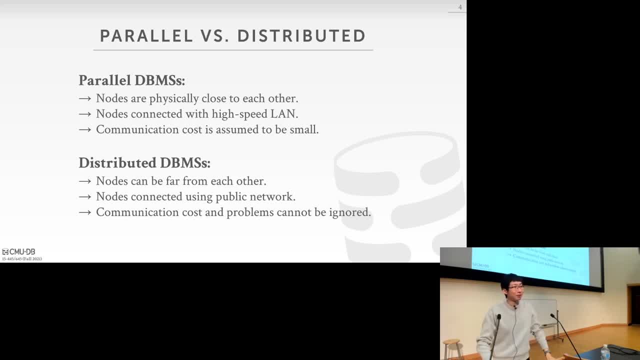 two lectures will actually be the last high level topic of this course. right, it is fast, right? so today and the next two classes we'll be talking about distributed heavy system, all right, so i don't know whether andrew has mentioned this before, but in previous years 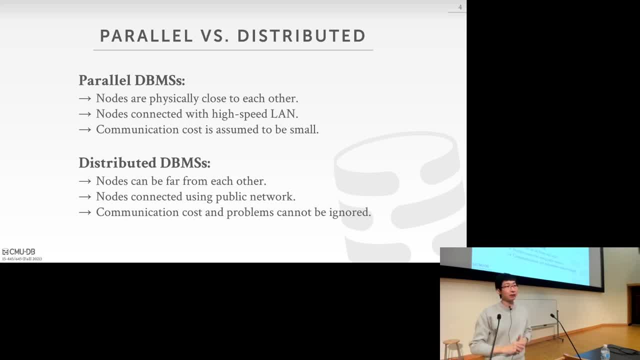 we have. we probably have discussed the concept of a parallel database when we talk about query execution earlier in the semester, so there's actually a difference here, right? so when we talk about parallel databases, we may also partition the database into different portions, and different parts of the system are responsible for different things, but we sort of assume that those nodes in a 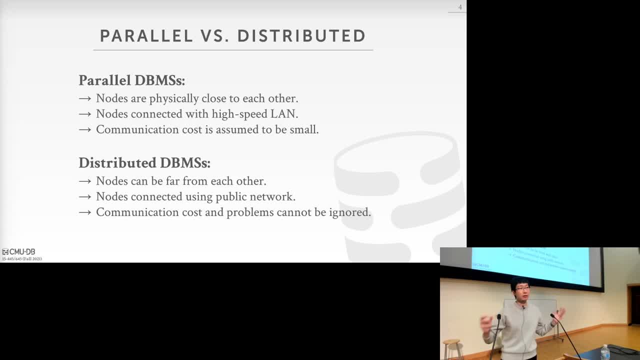 parallel database actually close to each other, and then there's a really fast connection that would coordinate it and all connect those different nodes, and those nodes go together right. so one knows, if it's one node is done, then the entire database is done right. there's no failover kind of stuff. and then 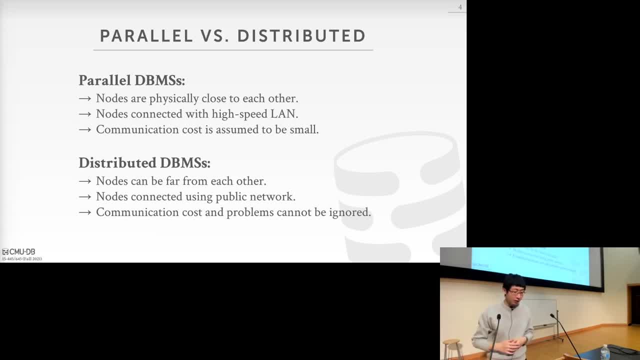 we also assume the communication cost is small, right, but today's lecture we're going to talk about this kind of distributed habits where we actually can arrange different nodes that either in the same machine or could potentially be very, very far away from each other, right, for example. 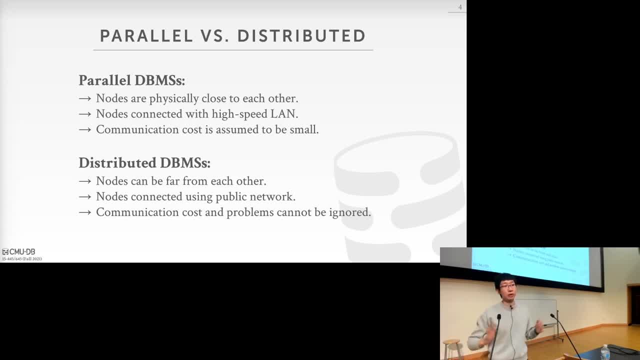 in a distributed database, the nodes or the partitions of data could come from different regions on different, even continents- right in a cloud, for example, and then they would communicate with each other using the public network, which means that the network latency could be really high and then different nodes can actually 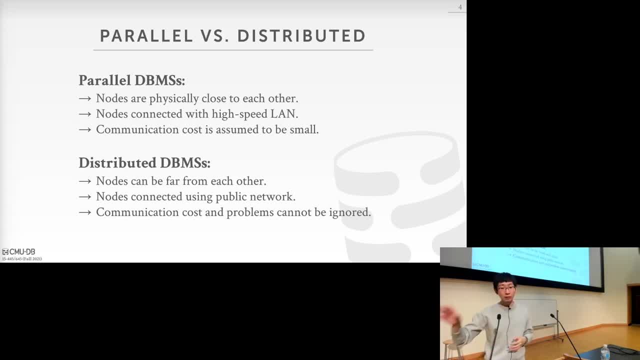 fail, right. so in a distributed setting, if one node is done, we also need to have a mechanism for the whole system to be running well, like handle the case where one node failure and you spin up another node to replace that node, etc. right, and again the communication cost can be high and then 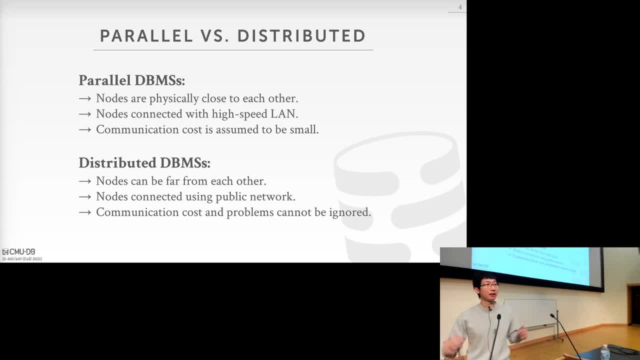 there could be problems of a node failure that we are going to handle in a distributed setting, but you can see that the distributed database would actually be a much more powerful right. you can distribute or even replicate your data across different locations, different data centers or even different continents, right. so if one data center is down, you have another data center. 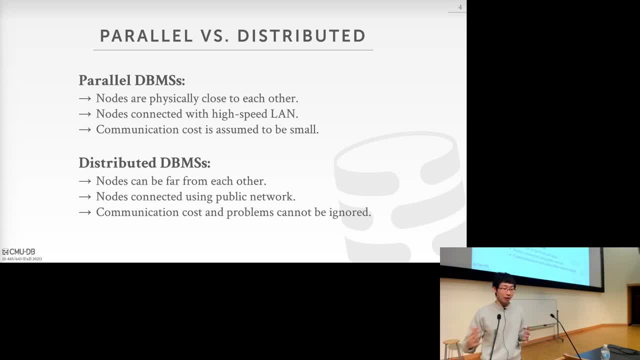 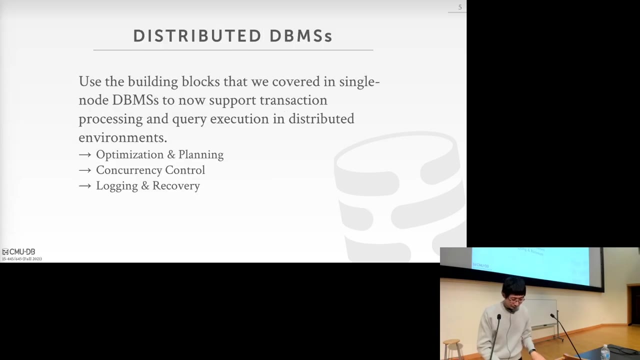 is still up, and then your database system. i mean hopefully, uh, you have a mechanism to let the database system still be running so the system can have much more availability and then give you much more flexibility on to where to partition your data as well. all right, so that's what we're going to talk about today. so one thing to note here is that, for all the topics, 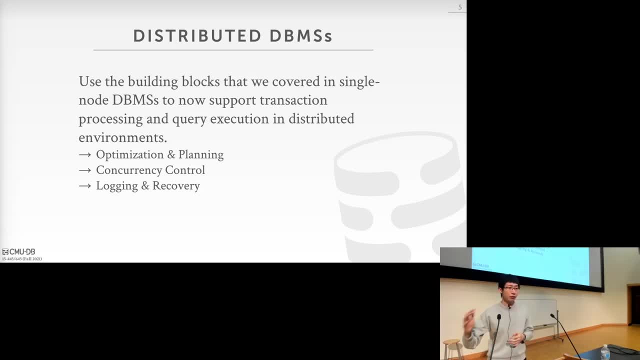 we have so far talked about in this class. i mean all those things would we would still be using them in a distributed system setting right, for example, in a distributed database. we will still be doing concurrency control. we are and we will still be doing login recovery etc. but the only thing is: 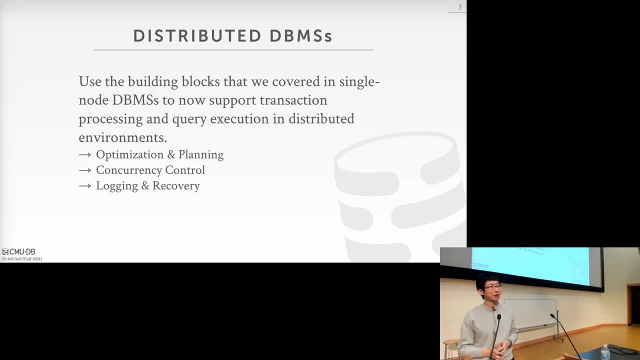 that most of those things will actually become harder, if not a lot harder, right? so, for example, if you want to do it, if you want to do a concurrency control, well, then you not only need to handle the case where a different part of the data may be on different machines that are potentially 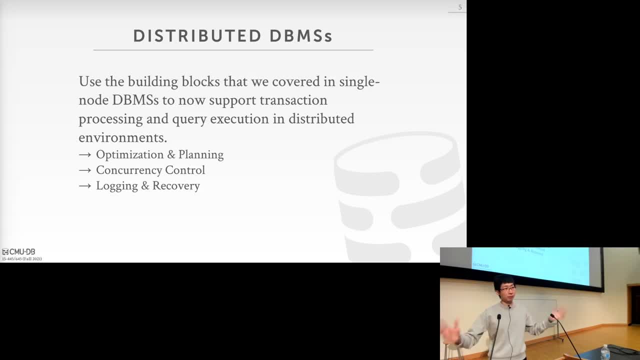 be far away- i mean very high communication cost- and also while transactions are executing. when you lock some data, then that node may go down right, that node may go down right, and so that's what we're going to talk about today, and then, essentially, your log would actually never be. 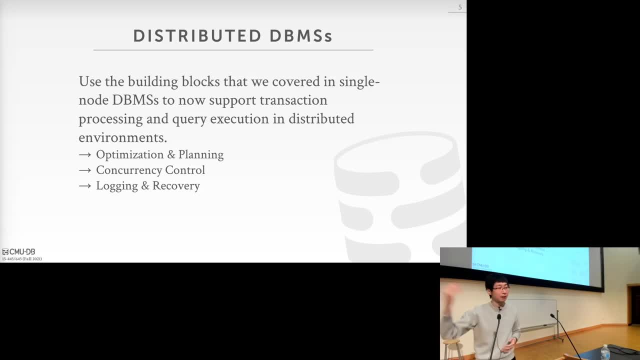 released if you don't have a mechanism to handle that, or resume or like, spawn up another node to replace that node, etc. right, so we'll still be doing most of these things or all of those things, it's just there will be much more challenges in a distributed environment, all right. so today's agenda: 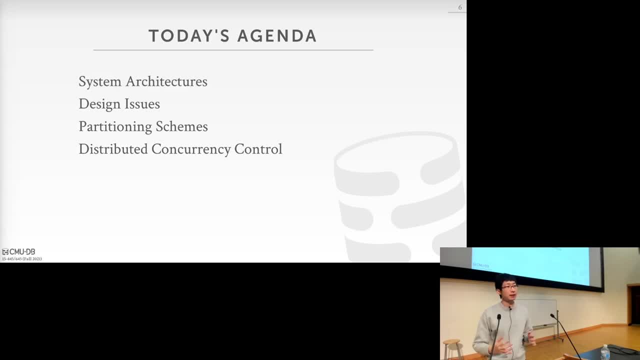 will actually be talking about some of the fund, different foundations or like basic concepts of distributed database scenario, right. so for the class on wednesday as well as next monday, we'll more talk about specific algorithm, right, like more implementation details, but today we are going to because i mean the, the, the whole topic of distributed database could actually very well be. 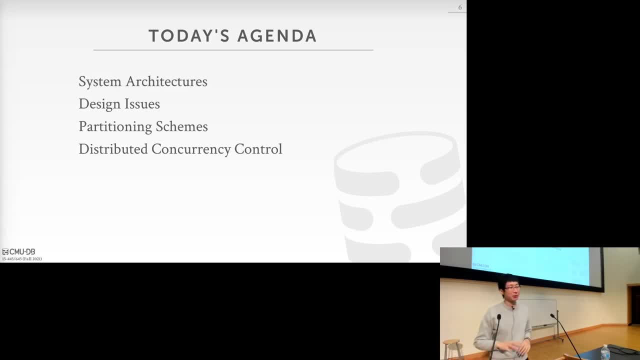 its own like similar strong long course. right? so today we are just only going to kind of scratch the surface and talk about some high level mental model, as well as intuitions and then the next two classes. we'll go into a little bit more details, right? so specifically, 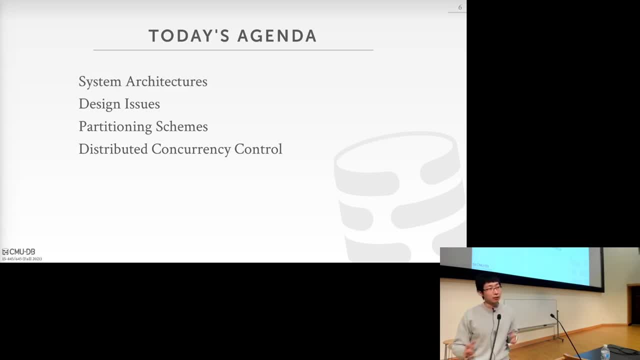 we are going to talk about, there will be the high level architecture that we can choose when we're trying to build a distributed database, and then what about the related design issues? and then we also talk about some methods to partition your data right across these different nodes or machines. 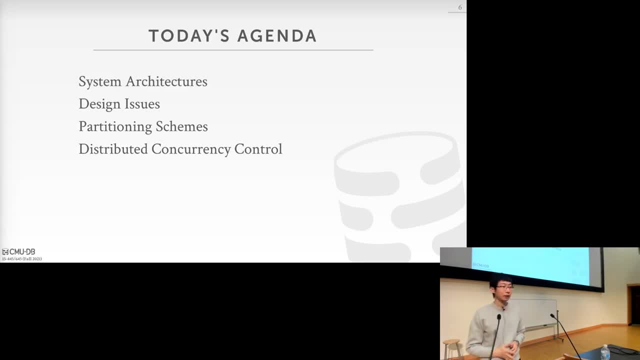 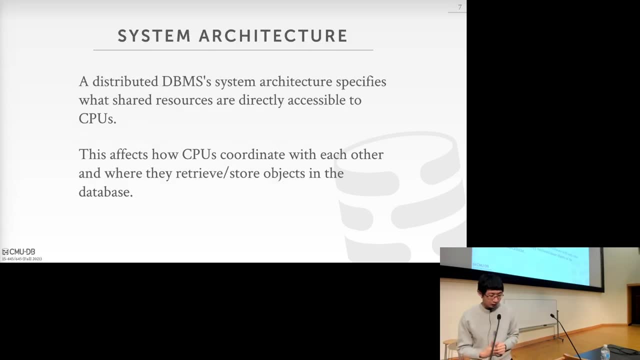 and then, lastly, we'll give. we'll talk a little bit about distributed concrete signature and we'll get more about that next monday. all right, that's today's content. so, first of all, the system architecture. especially when we say distributed database, right, we, we refer to the architecture of a distributed database. 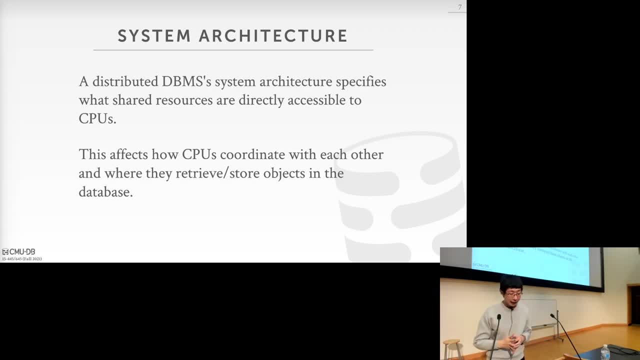 as the mechanism that the system is going to allow or specify what resources can the cpu directly access, right? so i mean every system has architecture right. but in distributed database, the architecture of a distributed database database is specifically referring to how system allow the cpu to directly access different type of resources. say whether the system it allows the cpu to directly access the. 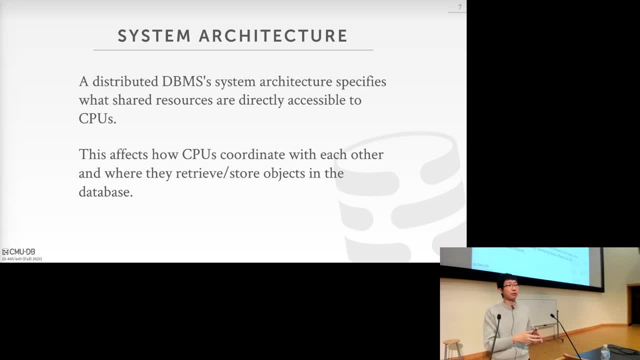 data on the disk. well, if the disk is on single machine then the the system can allow it to access, but you could choose also choose not to allow and then if the disk is on a different machine then obviously i mean the cpu cannot directly access that data on the disk on different machine. 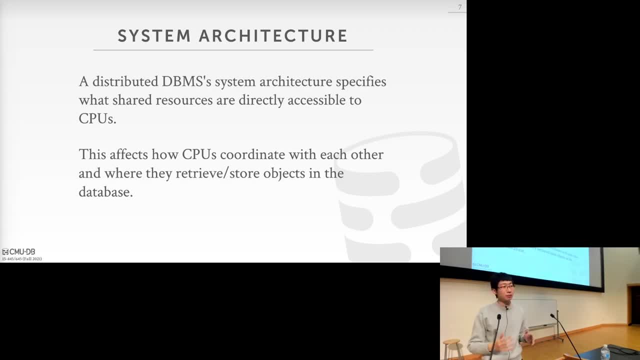 right. so this is kind of like this kind of decisions will be called the architecture choices of a distributed database. then this, actually this choice of architecture, would very well affecting many other implementation details and algorithms that we choose to implement a distributed database. all right, so this sounds a. 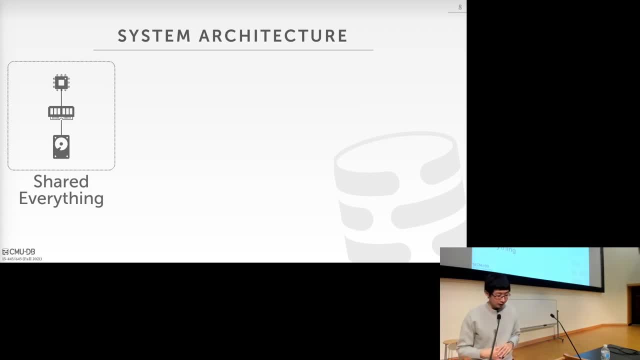 little bit abstract. let me give you some specific examples. so the first type of distributed architecture, first type of distributed database architecture- i need to be specific here- will be called shared everything. so this will actually be exactly the same as the single node database we talked about so far in the semester. essentially, i mean, everything is on the same machine and the 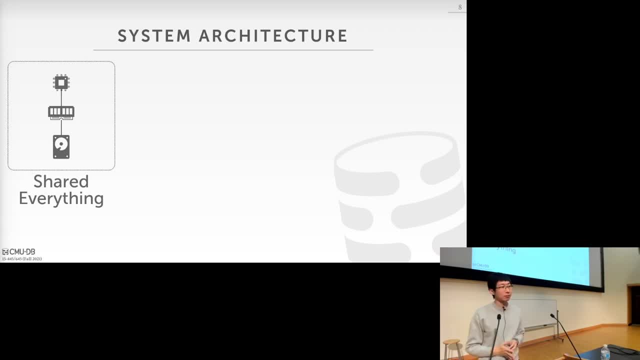 cpu can directly access both the memory and disk on the same machine, right? so i mean it's like a shared everything and then it's the same as a single node database. that all, that's the architecture the the, the single node database system, will be using. uh, if we consider the terminology of a, 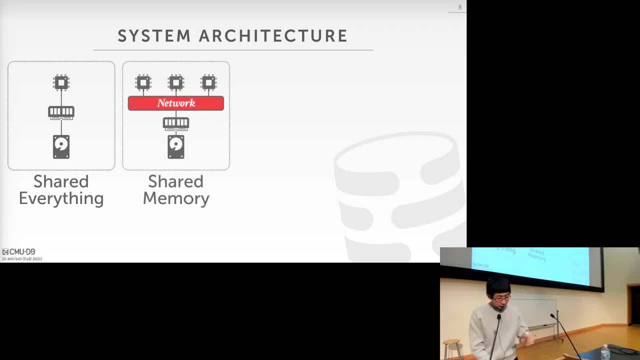 distributed system architecture, all right. so now we got to, uh, we got a scenario where, uh, the resources can be on different machines, right. so the first architecture choice of distributed habits will be called shared memory. so in this architecture, again as this illustrated here, these cpus can be on. 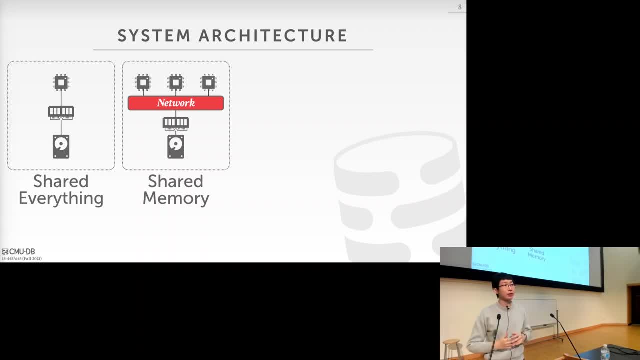 different machines, right? i mean can be very, very far away from each other. but then we are going to assume that there's a central mechanism or unified channel that allows these cpus to access memories like a central place of a big chunk of memory, either on a single machine or on different machines, right? 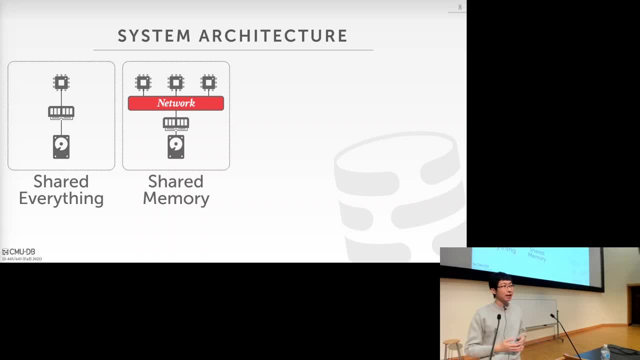 so this mechanism could be um, for example, rdma or infiniband, but the idea is that this, uh, these cpus don't really know which memory chip is on which machine is like local to the cpu or not. right, it always goes through this unified interface that would hide the details of the 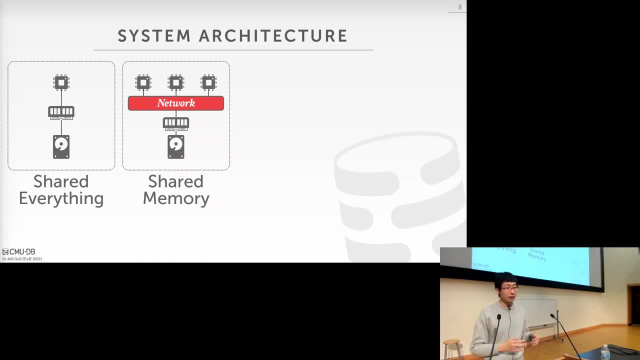 memory and this interface would deal with the memory, uh, consistency or coherency, uh, for this big chunk of memories, either i mean on a single location, or memory distributed on different places, and then each memory would, would have access to the local disk, uh, i mean attached. 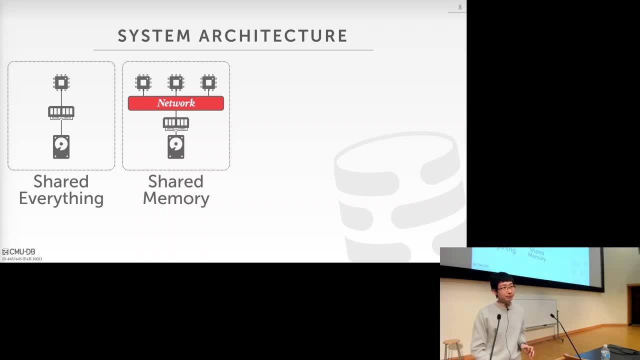 to it all. right, so that's called a shared memory, make sense. so the next architecture, which is actually a little bit more uncommon, will be called shared disk, right? so kind of just move this central memory to a small dimension, to the smaller disk, and you can clearly see from this interesting 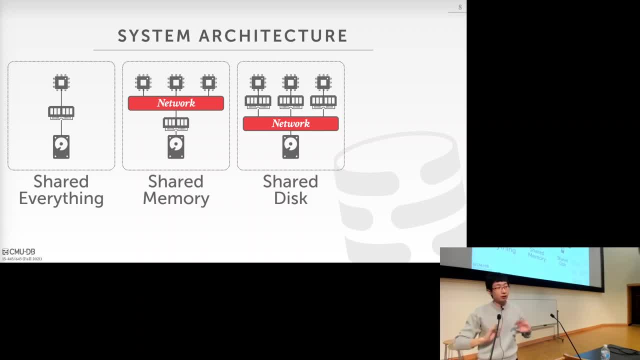 picture this and this. what it does is it allows sharing the different areas in the community right in this particular chip to be able to take in different restrictions, different units and systems, different WWEOK systems of mechanistic functionality. so in a case like this where we have a different memory system, this could be possiblehearted. 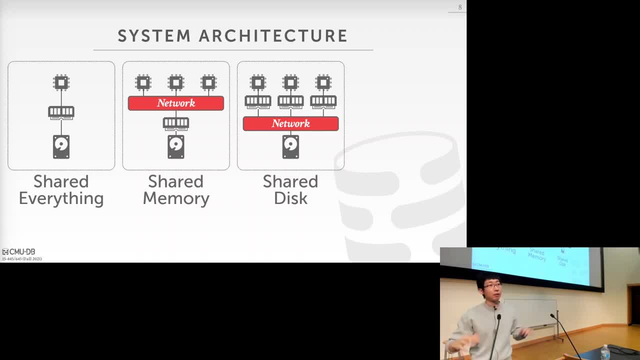 sharing and different teams of the computing systems, a different systems, uh, all in one, could be activated in different parts of the system, right? so, just like by recipe memory, there's a central- again centralized- interface or unified channel that would allow this memory to read data from this like a shared big chunk of disk space, right? either this disk, 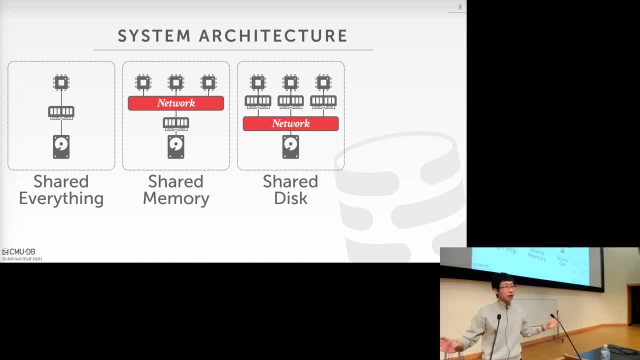 could be on a single machine again or could be distributed on different machines, doesn't matter. but the important thing is that when any time a CPU wants to read some data, it first go to its local memory and then the local memory would actually go through this unified interface. 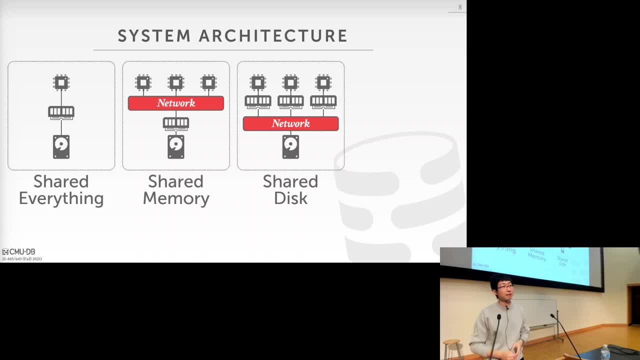 to get data from a shared pool of disk space. all right, make sense. well, this is actually think of this. this is like we'll get to the details. but this is actually much more common these days, and especially in the cloud area. right, this shared disk could be something like. 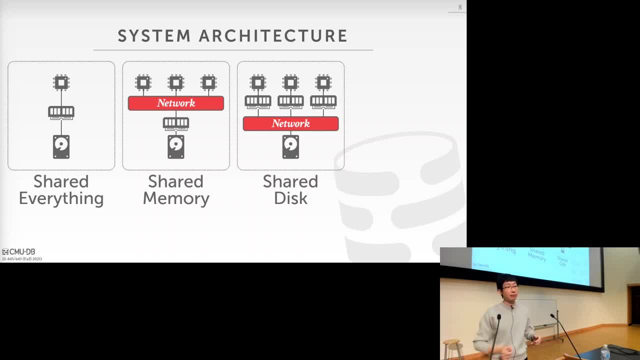 s3 on amazon, for example, right, so you can have a different compute node. but then at the end of the day they all go through this amazon s3 service to get the data, regardless of which machine exactly the data is right. and then the last architecture would be called shared nothing. 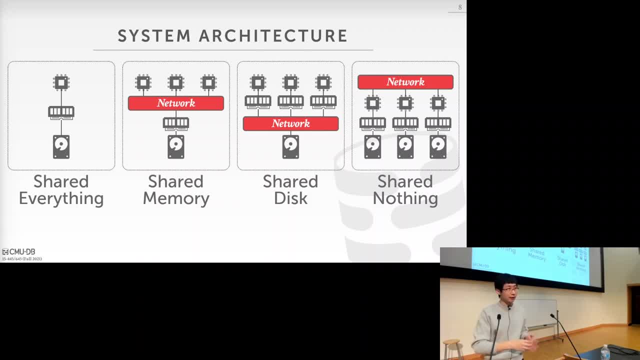 is actually also kind of common, but more common before 2010s, before the cloud time. so essentially in this architecture i mean the CPU had, every CPU would have its own memory and disk directly attached to the local machine, right? so every time the CPU wants to read data go to. 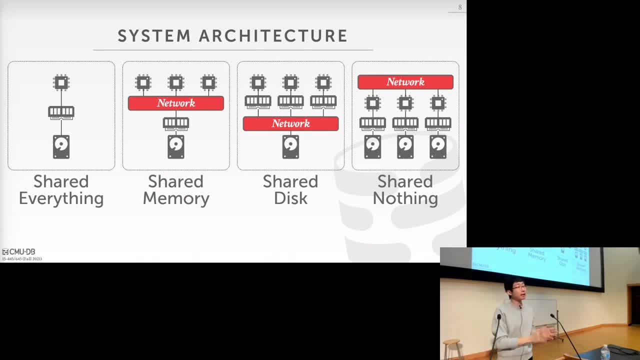 its local memory then go to its local disk. but then any time one machine or one CPU needs to access data on a different disk, they actually need to go to a higher level network protocol. sometimes it just would be a public network, right, they would go to this higher level network. 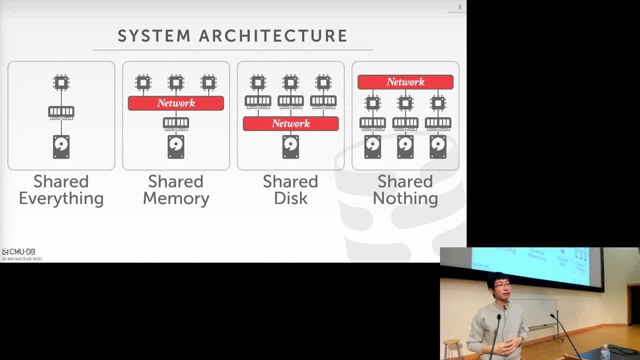 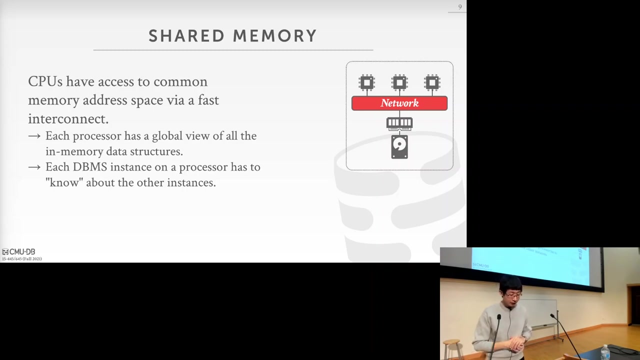 communication channel to coordinate the data reside on different machines and different disks, etc. but the important thing is that every CPU has its own memory and a disk and there's no resource sharing below CPU. all right, make sense, cool. so, uh, let's give you um some more specific about these uh different architectures. so the first i 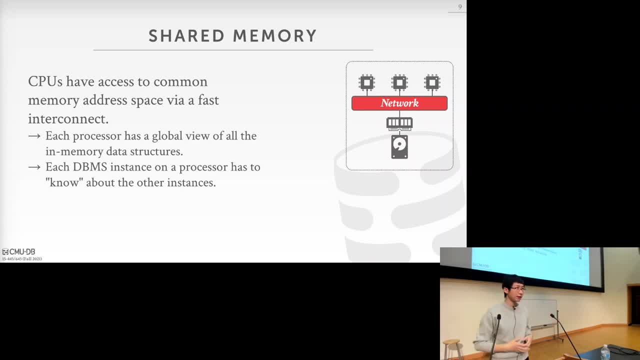 mean the very first would be, uh, shared everything, but that's kind of, there's a single node architecture. they were that we already talked about, right, so in the distributed setting, the first architecture i mentioned would be a shared memory. and again, i mean these CPUs will actually 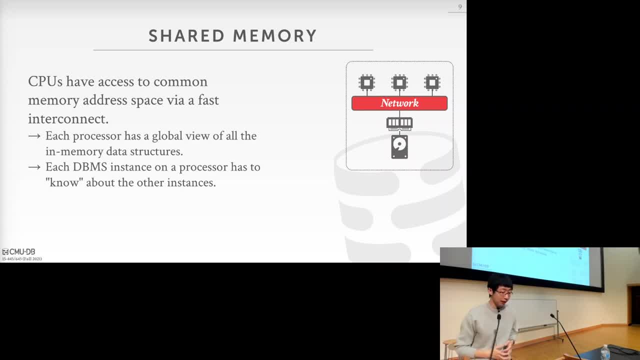 have a uh have access to this common memory address space via a first uh interconnect and oftentimes this could be implemented with RDMA right, remote uh direct memory access or just by. by the name you can tell that that's kind of like an interface that would allow uh different CPUs directly access memory reside on different machines. 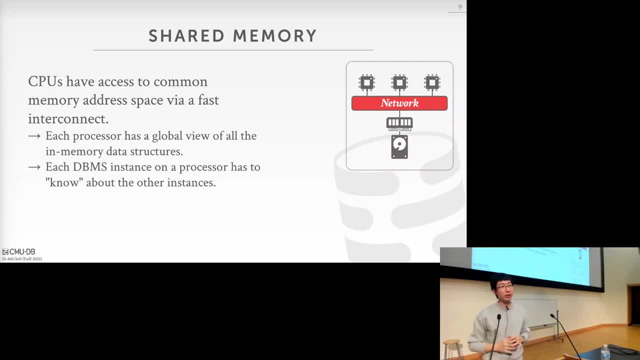 and then, like i mentioned here, uh, every processor would actually have a global view of the entire memory, right? so, no matter where the memory chip resides, every CPU will know what will be the content that the database system has on each location of this entire memory space, and then can. 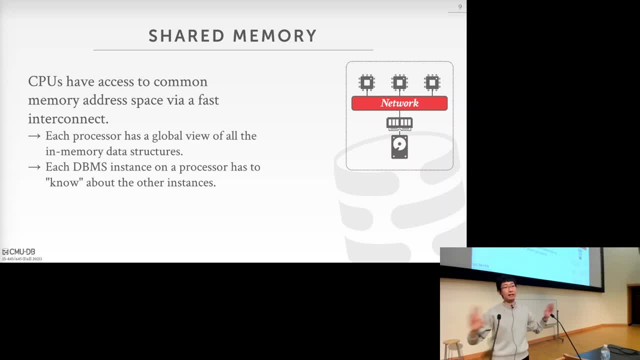 either read data or write data on any location in the entire memory address space. okay and then? yeah, then all the coordination would be happen in this network layer and then this network layer or the centralized interface, will be handling all the cache, coherency and consistency, etc. but one thing to note here is that actually, in practice, almost no database system would 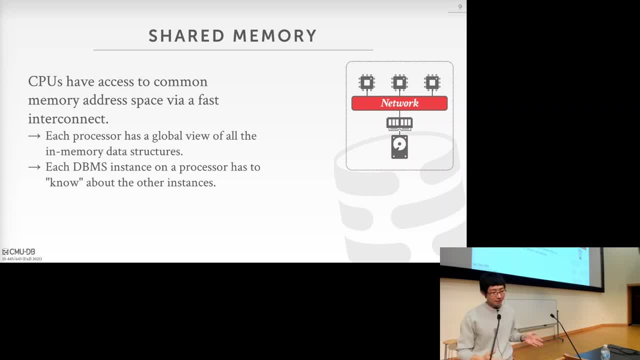 implement a distributed architecture this way and the, the, the, the main reason would be just that, um, in order to coordinate the cache coherency as well as the cache consistency with this, a single network uh interface is actually a pretty uh difficult and the overhead is is often high. right, it's like it's much easier to deal with the issue on onto. 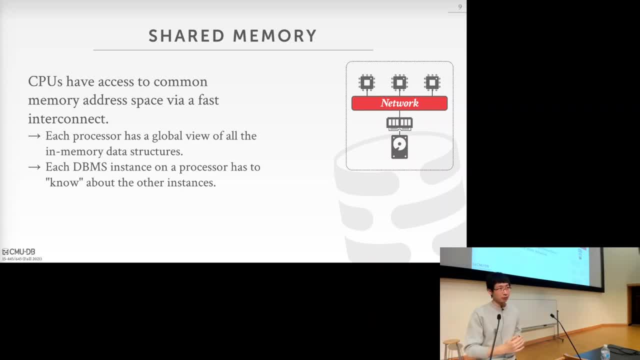 the lower layer, or even just use a shared nothing architecture, right? so in practice, almost nobody used that. so what would be more common? uh, use case of this idea, right? not necessarily in database, but a common, more common use case of this idea would actually be a high performance computing. 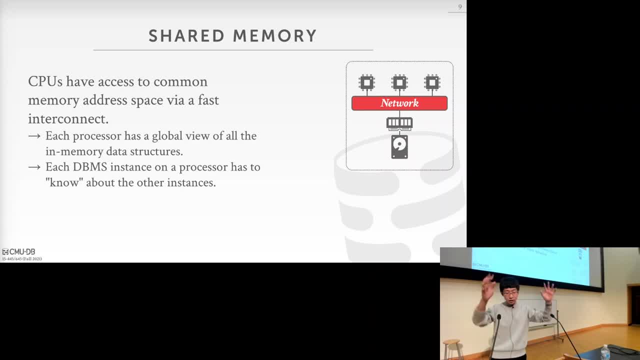 right, because in the in that world you often have this like a giant machine right with lots, of, lots of CPUs and also a centralized location with a giant I mean a chunk of memory like terabytes, etc. so in that uh, in that world, then it's actually a common to have this uh. 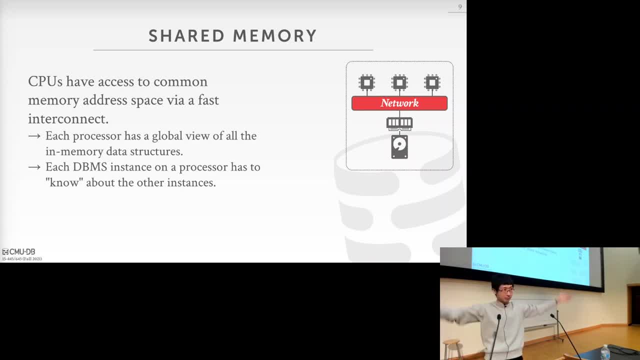 shared memory address of this, like an entire big array of memory in your data center and then using this idea to coordinate uh the uh communication between different computer nodes. right, so it's actually a more common. this idea is more commonly used in the HPC world rather than the distributed 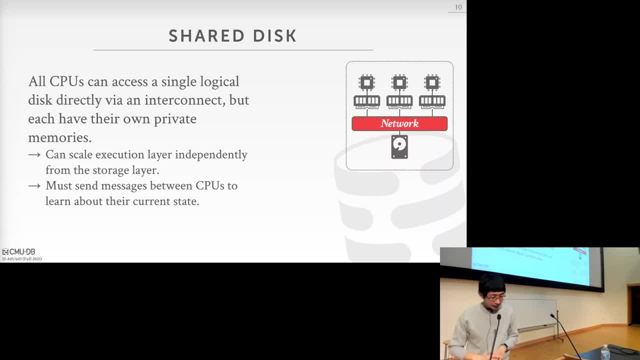 database system world. all right, so next idea would be a shared disk. again, like I mentioned, this is actually a very, very common uh, this disk, especially in the area of cloud, and then the, the, the high level idea would just be that um each, each CPU would have local access to the. 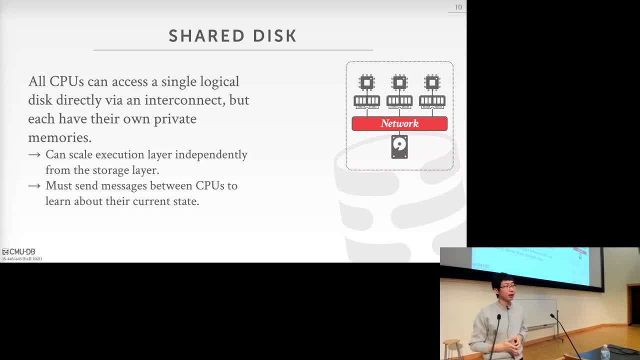 memory by doing all the computation and then do the read, write memory, read and write there or in the reader right, in the buffer pool, in other words. but then when they need data, they would actually go to this centralized location with a unified channel right and then to- uh, I mean to- 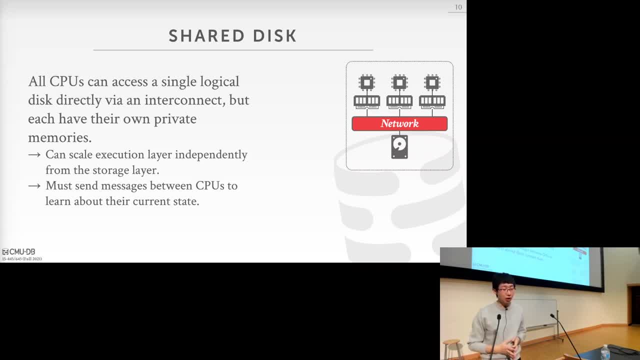 store uh data there. so this is actually more common, especially in the cloud area, because this have this uh appealing property where it can allow you to scale the uh storage and compute independently, independently, right. so? because in this architecture, this um this, all the uh data access is going through this centralized interface and all the details of how many disks are there. 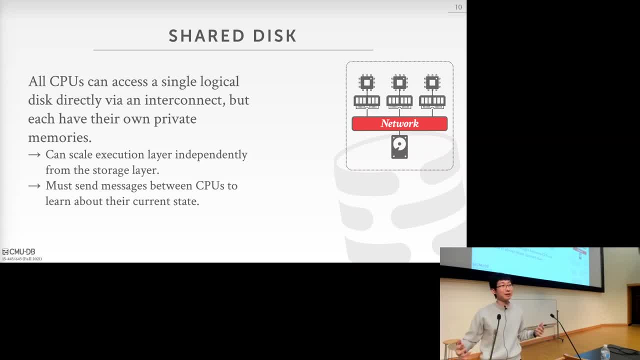 with locations of all those disks etc will actually be hidden, right. so if your storage is not enough, you can add more disk space, I mean below this network interface. then this compute node doesn't need to know right. similarly, if you realize that you don't have enough compute, 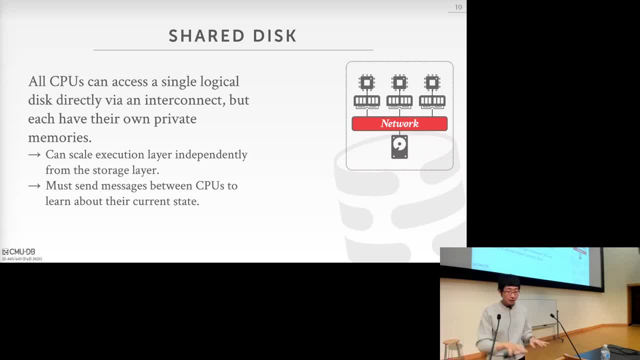 capacity but you have already have enough disk, then you can simply add more compute node and then that doesn't affect your operation on the disk, almost doesn't affect the operation on disk, even in some cases don't handle, handle a few corner cases. so this is actually very appealing property, especially in the cloud. 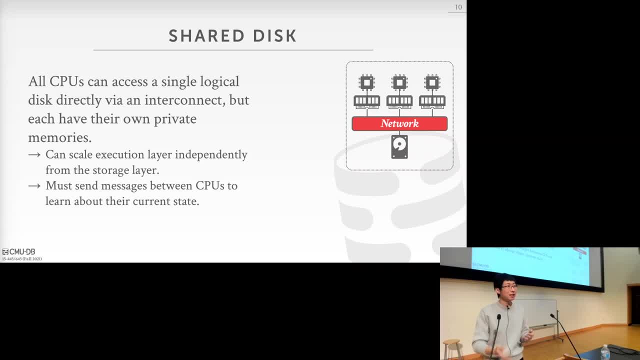 area. people want this um convenience and flexibility to deploy their application applications and scale resource resources up and down in the cloud, right. so having this shared disk architecture would be a very well uh compatible with that goal, right. so another thing to mention here is that even though, uh, we have this separation between 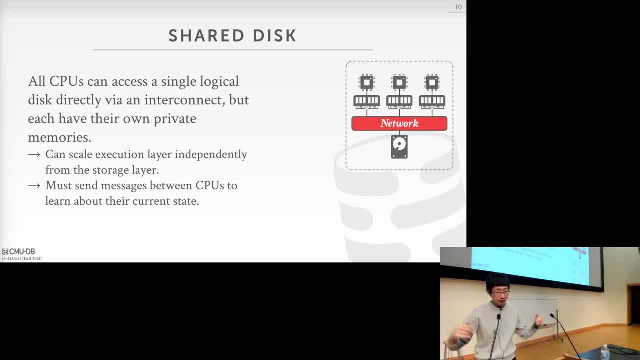 uh memory and disk and all the data access going through this uh network layer. but while we, the database system, are executing queries, especially executing transactions, right, there would also need to be direct messages sent between this computer node or between this cpu and memory, and we'll. we'll know more details later, but essentially, if you want to doing things like 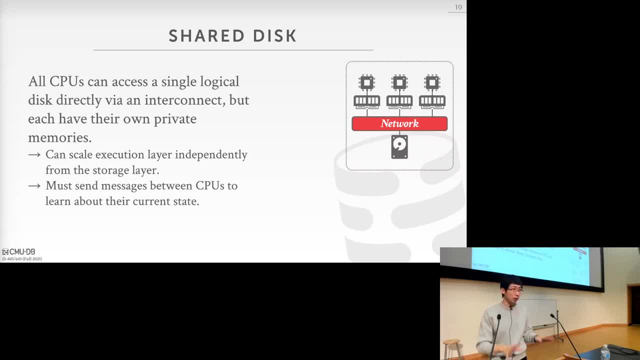 a concurrency control, for example, then you still need to do a little bit of coordination, even though, uh, you read all the data from this centralized location. okay, so again, this like just examples of the system, uh, that would be using this architecture architecture, and most of the systems are after. 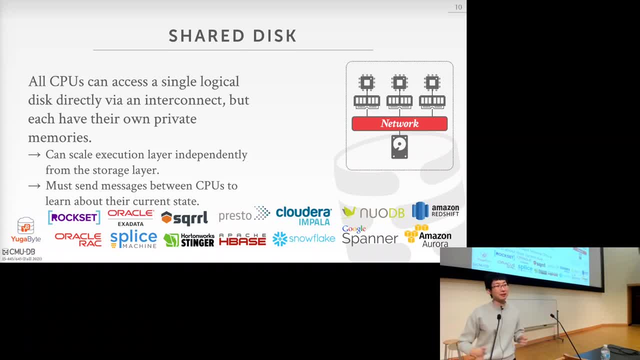 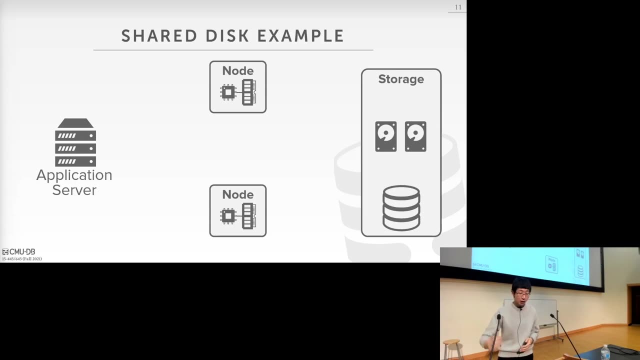 2010 would actually, oh, most of the distributed heavy systems after 2010, especially a system in the cloud, uh, would actually, uh, prefer this architecture, all right, so i'll give you a specific example here. right, say, i have a one digit distributed database with a two a computer node. right, that would? 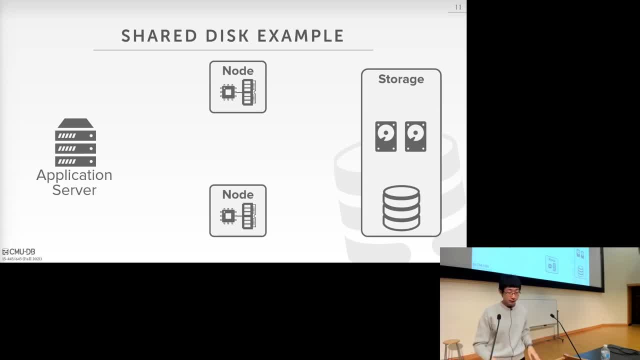 include the memory chip as as the cpu processor, and then we have this centralized location to have all your data, right. think of this centralized equation, for example, as the amazon s3. uh, i mean data interface, data storage interface, right, and then, for this node, think of them as 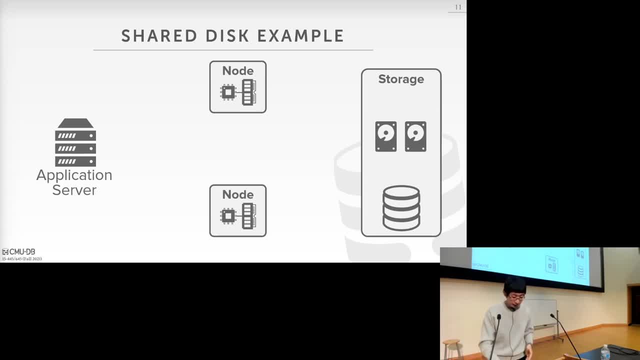 amazon ec2 instance, for example. right then, in this case, say, the application server wants to get data with id 101, then what this node, or computer node with this processor as well as the memory, would do? that it would just go through this unified interface for the storage to find out. 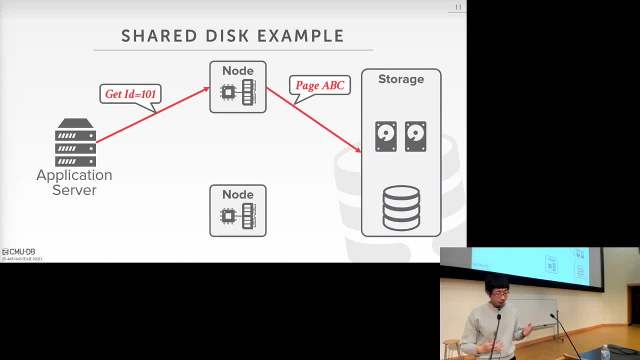 which would pay page that contains the id uh with continuous, contains record with id 101 and then read the data and or put that specific page to the buffer pool in this uh node node up above right. i mean similarly if you have another uh, another uh transaction. 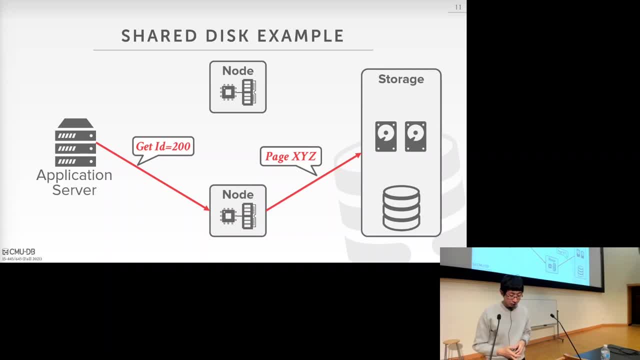 so sorry. another query wants to read: um, i tuple with id 200 and then this node will go to, through this interface, find that uh page on this shared disk space and then get that page back in the buffer pool and read that out. all right, so again, with this you can easily scale the compute and 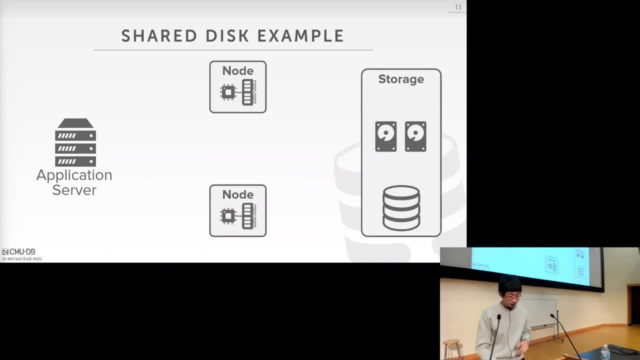 and storage independently, right. so say here, for example, i want a. i realize that i don't have enough compute capacity. right, i want to add a new compute node. then that's very easy, right, you don't need to do. mostly you don't need to deal with anything in the storage space- you just add another compute node. 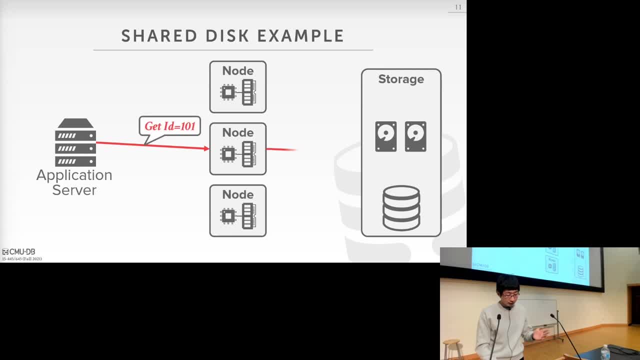 with additional cpu ss memory and then say now you want to, you still want to get a record with id 100. then you can just go to um sdisk and get that page back. all right. so what would be a little bit tricky here is that say, at some point you want to update. 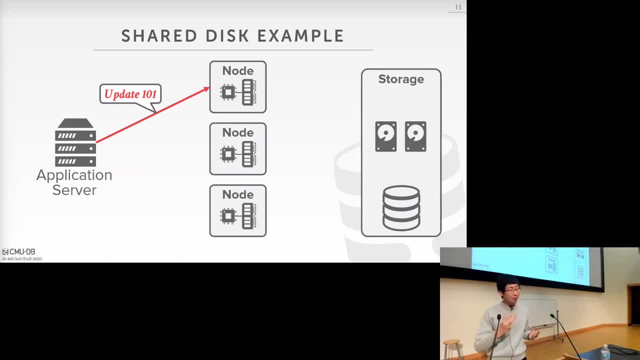 this: add a page or this id: uh, sorry, you want to update this record or tuple with id 101. right then, you could do that. right, you could go through, uh, this computer node and then eventually get to the storage layer and then update that page. but the problem is that, like i mentioned earlier, other 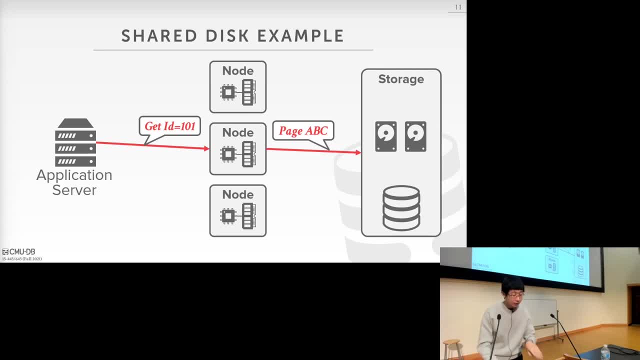 nodes in the system, for example here right. other other nodes in the system may have read this tuple from that page as well, right, and then have some local copy, i mean in the of this page, in the. in this case, if there's an update in this compute node right, also update this record. then there's. 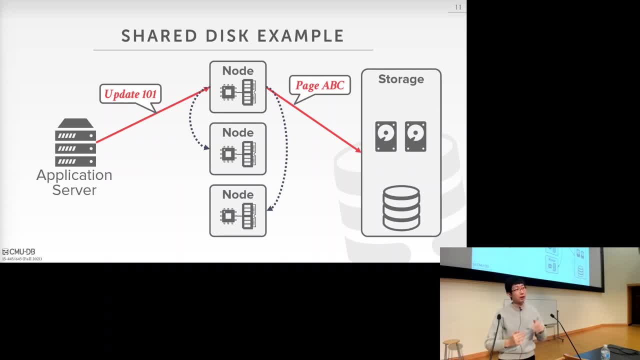 like i mentioned earlier, between these computer nodes. even though it's a shared architecture, there would still be a message passing between this computer node that you coordinate- hey, which node has which copy of which page or which record? and then, when update happen, how do we need to? 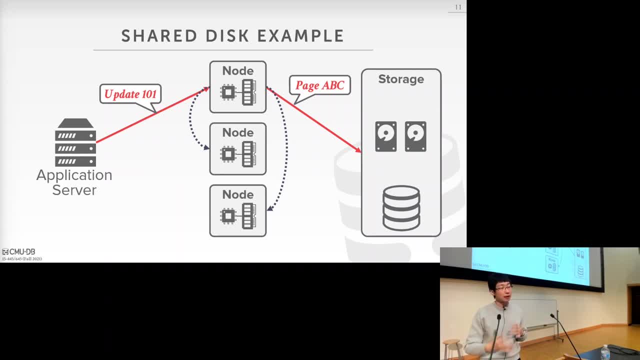 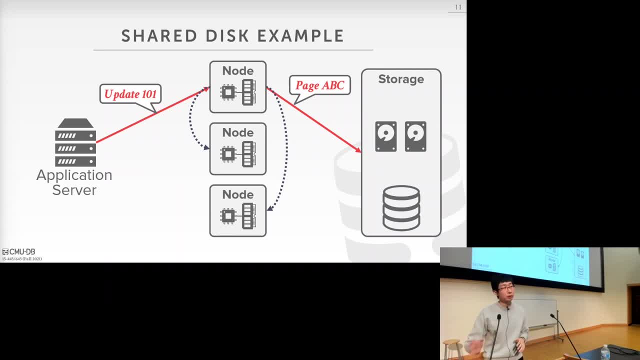 need to be a coordination between the different computers, and we will talk about the detailed concurrency control algorithms later. all right, but this is this illustration of a shared disk, distributed heavy system architecture makes sense. okay, so similarly right. this is the same as you can scale this computer node right, add a new. 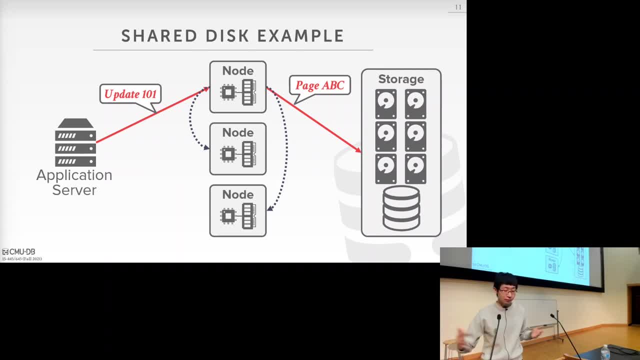 node with a cpu and memory. i mean you can also add, i mean storage node below this shared disk layer, right, and then again, i mean you don't necessarily need to attach most of the stuff in the compute layer because this is always all this storage will be hidden behind this and unify the interface of this shared disk networking layer. 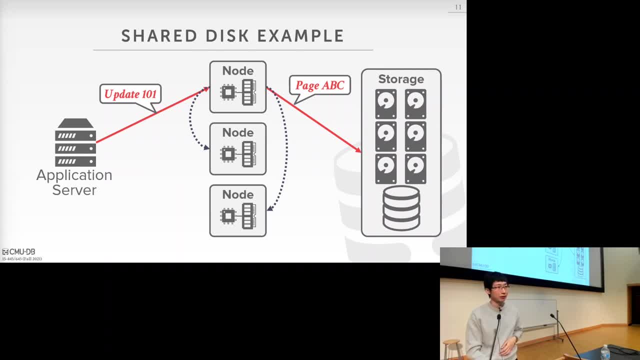 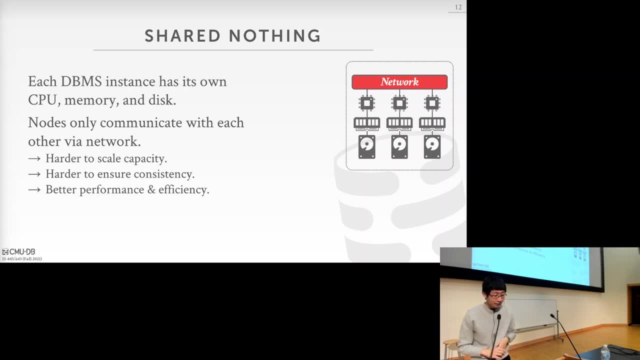 all right because they're very easy to scale resources up and down, especially independently. so the last locator, our last architecture, would be a shared nothing architecture, right? so again, like i mentioned before, every instance in this or every node in this architecture will just have its own cpu, memory and disk and then it will always access the data. 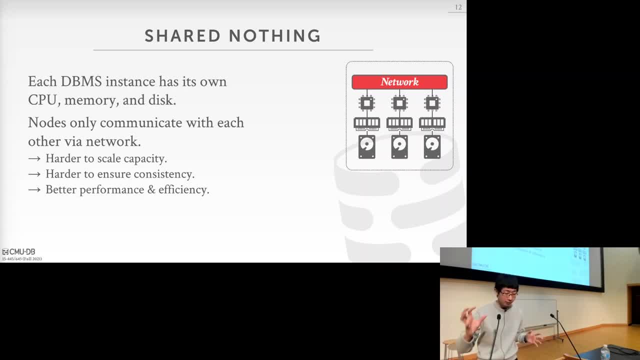 locally right, either memory or disk, and then when a specific node needs to access data on a different machine, it would actually go to this higher level network layer. in many cases it would just be a public network to get the data remotely right. so there are actually well. 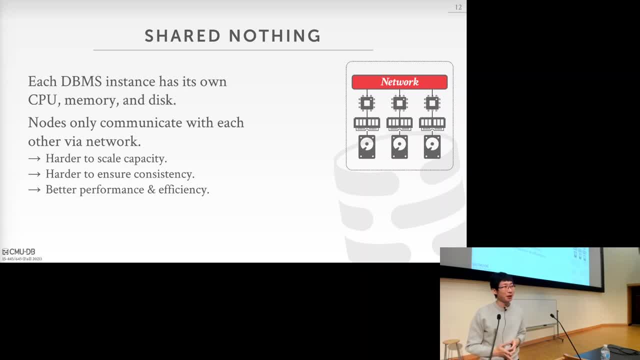 the immediate, uh, the. obviously the advantage of this approach is that if a query or a transaction only needs to access data on its local disk, then it will be very fast. right, because each, every cpu would have local memory and disk attached to it. and then if all the data- this query or transaction- 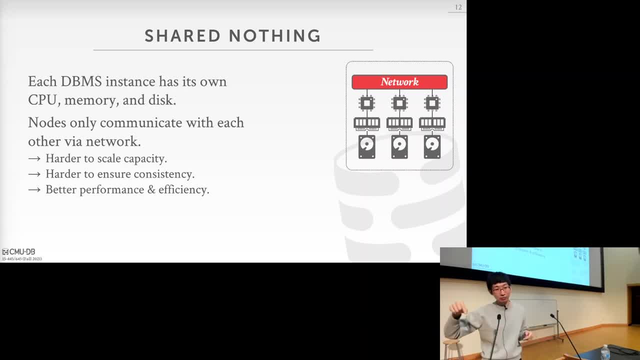 needs to access will be on this local disk. then it can just directly read everything locally, right? it doesn't need to go through the expensive network protocol, right? so that's the obvious advantage for this one. but then there are also a corresponding disadvantage, right? the first would be that 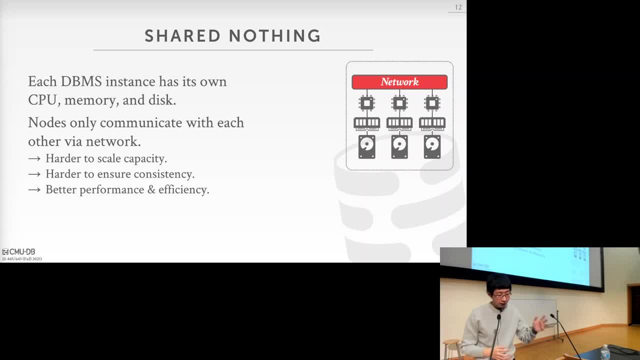 unlike a shared disk architecture, it's difficult to scale compute and storage independently, right, because every node will have a storage and compute and memory attached to it. and also is it also a little bit more difficult to ensure the consistency of data correctness in this shared disk, sorry, in. 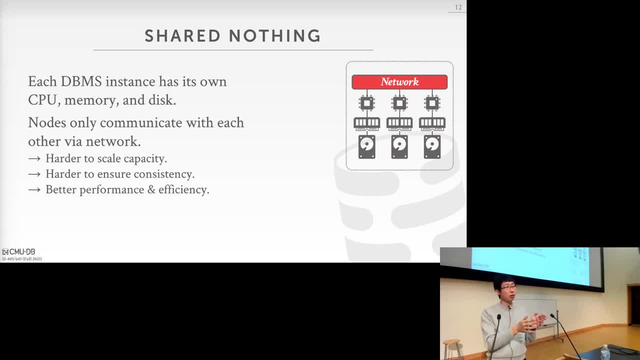 this shared nothing: architecture, because now every node will have its own partition of the data. right, it's not a centralized location of storage anymore. every node would have its own partition of data and every time one node, for example, update a record, then if other nodes needs to read the 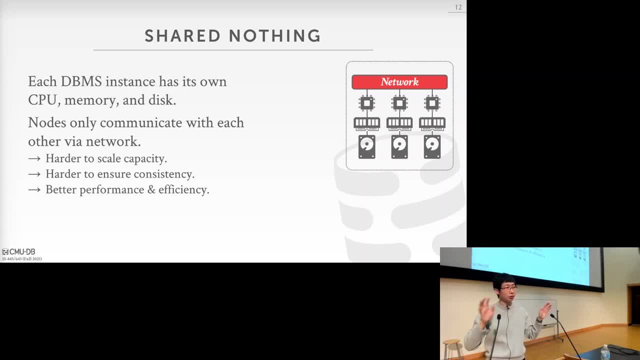 record, you sort of need to coordinate not only between a different competition, but also you need to coordinate the data between different nodes as well. in this share nothing architecture, especially i mean when you want to replicate a portion of the data on multiple nodes for availability reason. right, so could be a little bit uh, that challenges as well. 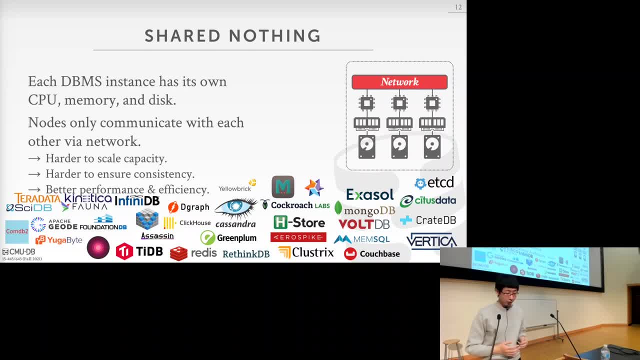 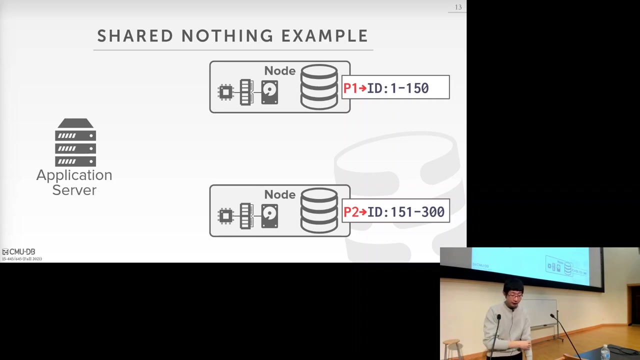 because of its efficiency and performance reason, many of the systems, especially systems before 2010, will actually use this architecture, so this is also very commonly used in distributed database systems. all right, any questions about the shared nothing architecture? okay, so just give you an example here. right, so in this shared nothing architecture, every node again would have a memory. 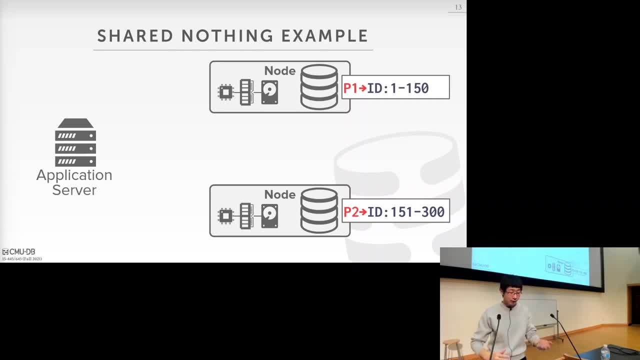 cpu as well as storage. and then, for example, here, let's say, we have two nodes. the first node, as i use it here, or in other words we can call it a partition right, it would have the partition of the data from id 1 to 150. 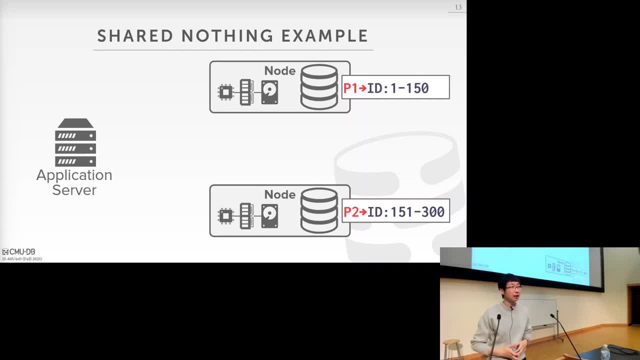 and the second node, for example, could have the partition of the data from id 151 to 300 right and, for example, in this case, if the application server sends a query that wants to access the tuple with id 200 and then this query would just be sent to this shared nothing architecture. 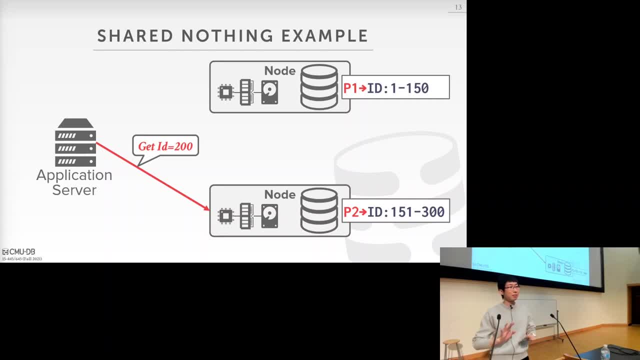 second partition: right. of course there actually needs to be some sort of a mechanism to figure out which query this actually, which partition or which node should the application server send this query to? right? we are ignoring that for now, but we will get to that later in this class. but but again. 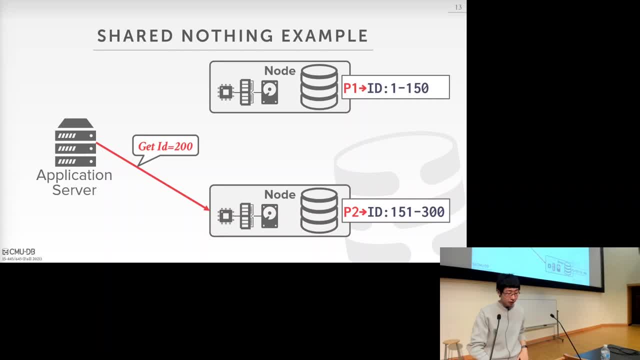 as illustration, this query will go to this second partition or seventh node, and then similarly, oh, in another example. right say now, another query wants to access two records or two tuples, right, the first, second with id 100. then for the tuple or record with id 10, it actually directly access it from. 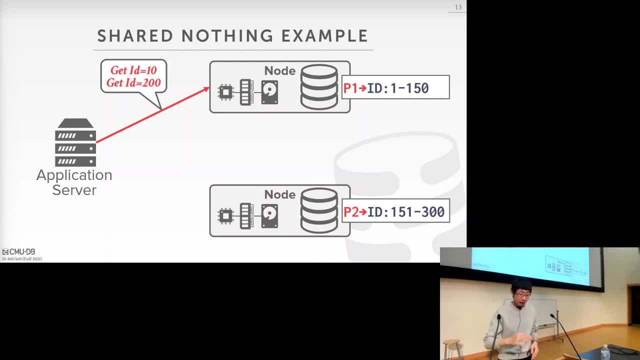 this local disk right because it's just on the first partition. then for the second request: right when this query: if this query needs to access the tuple with id 200, then 200 is not on the first partition. that handles this query right. so what typically would happen is that there would be a 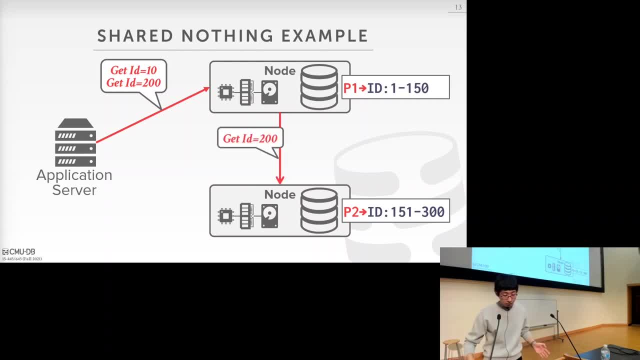 coordination between different partitions. so one common approach would be that this first node would send a request to the second node and then the second node would send a request to the second node and say that, hey, i have a query that needs to access um tuple or the content of. 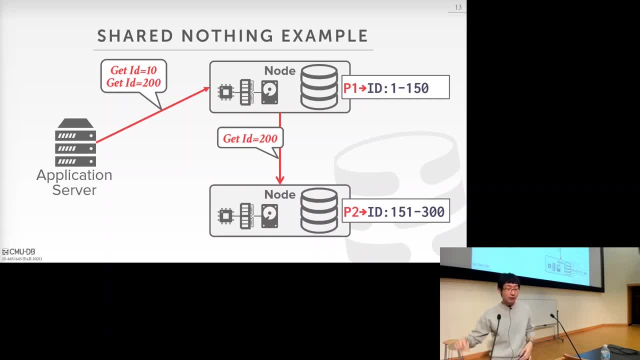 the tuple with id 200 and then it sends that to the second node. second node: read that uh record and then get that back to the first node. so there would be needs to be a coordination happening there in this share nothing architecture. all right. so here say that i want to scale the resources up. 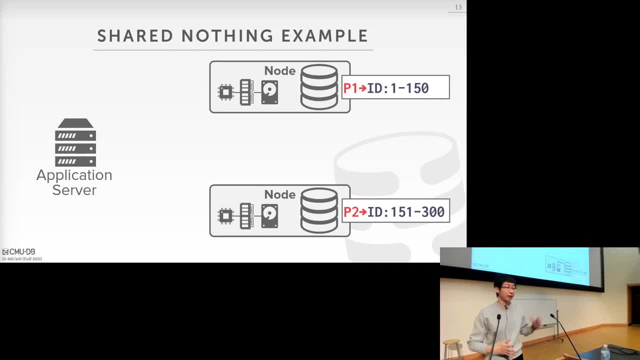 and down. then, unlike this shared this architecture, i can either only add the quark to the query to add more compute node or storage node. here I have to add everything, So every node will have memory storage and compute in it. But then one issue that we have to deal with here is that 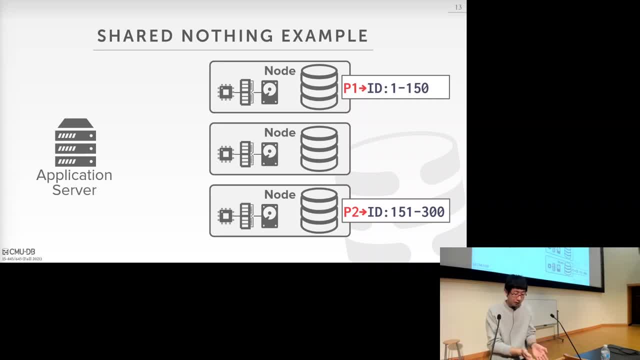 if we just create a new node with this empty disk space, then it's kind of like a waste. So if we still have this data- from ID 1 to 150 on the first node, 151 to 300 on the third node- 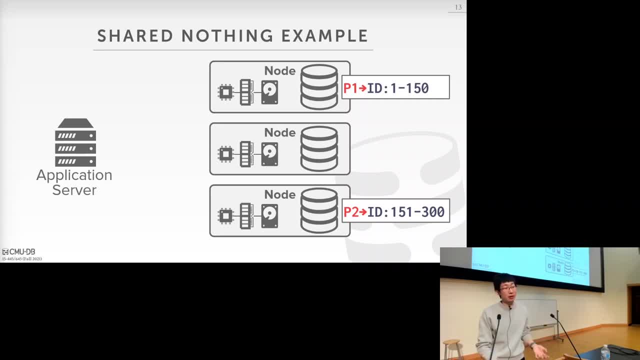 then there will be waste disk space on the second node. So typically what we need to do in a shared, nothing distributed database architecture is that every time when we add a new node we also need to redistribute the data, so move some of the data from the other node. 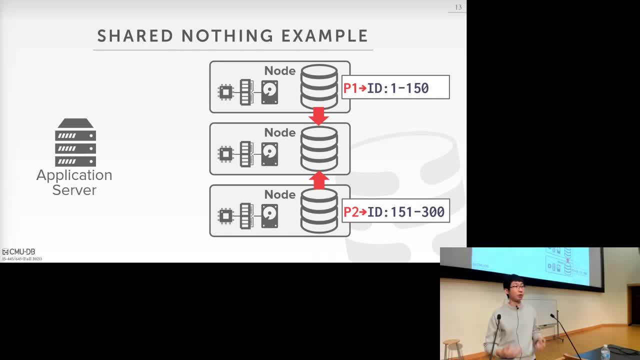 to this new node so that this new node also would handle some of the workload, instead of wasting this compute and storage here. So for example, here what we can do is that we can move 50 record from the first node and the 50 record from the third node. 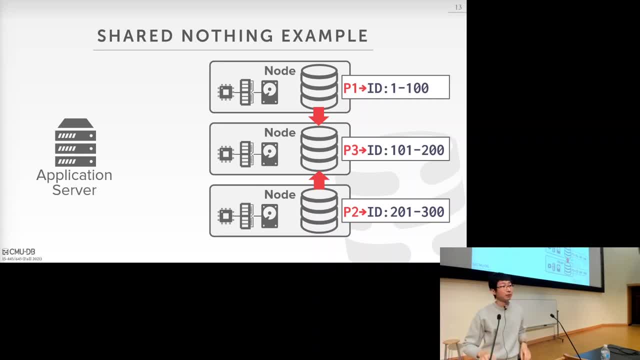 and get to the middle node. But here the illustration may seem simple if I just change the number and I have a few arrows here, But then in actuality this data movement actually can be very expensive and complex Because essentially it's a giant transaction. 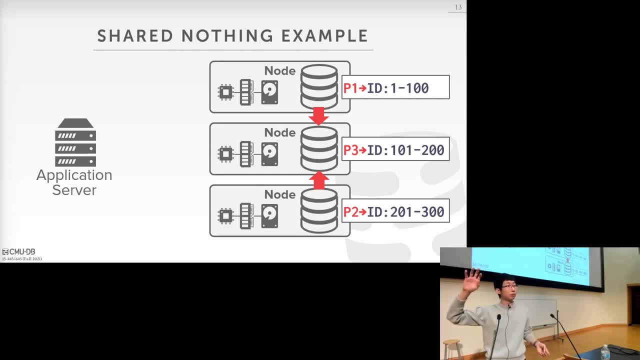 that you need to move one big part of data from, delete one big part of data from some node, or like a few nodes of data, of your entire distributed system, And then, after the deletion, you need to ensure that every single record 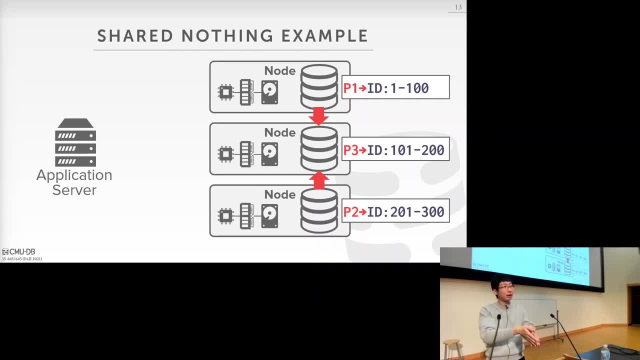 is correctly inserted into a new node And then, while this is happening, you also need to ensure that every system are also handling the other transactions or queries executing at the same time either reading or updating this record correctly. So this data movement is actually. 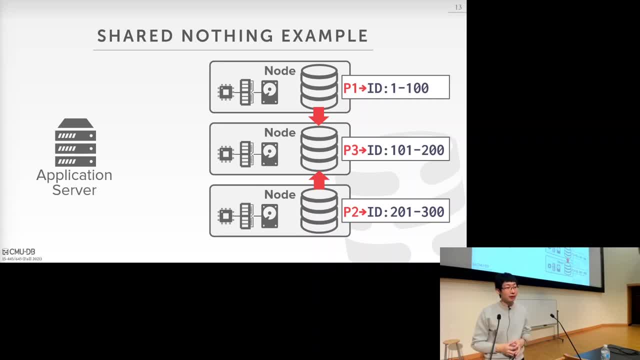 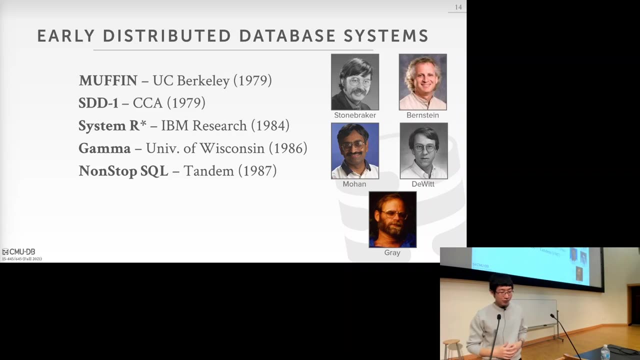 pretty expensive and complex, And then this also limit the flexibility of the system. All right, Any questions so far about these high-level architectures? Okay, So let's talk about a few specific, especially specific- design issues that involve when we're trying to build a distributed database. 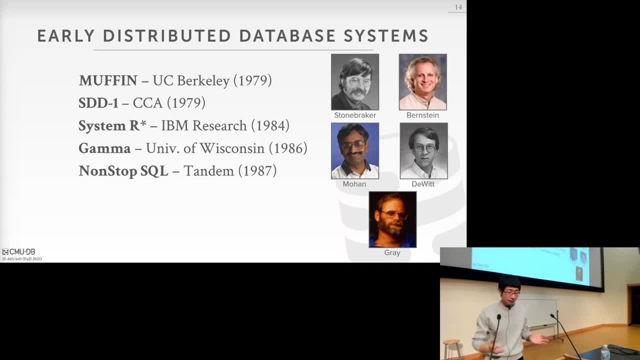 So a little bit of history here. right, The very- I mean like many other concepts in the database system world, I mean most. the distributed system is obviously not a new concept either. Right, So the very first few implementation. 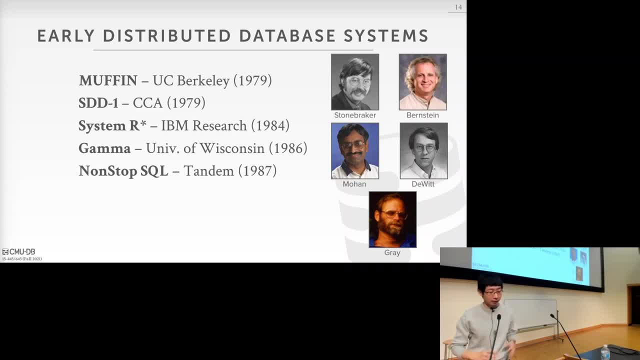 of distributed database system could date back to 1979. And there are actually two kind of like well-known concepts or proof of concept provide came up during that era. The one is called Muffin. I'd call some multi-node like a field. 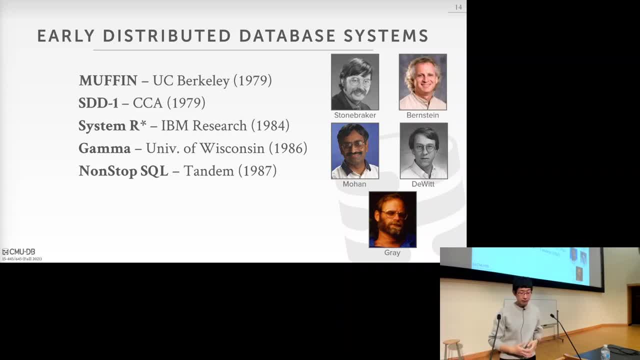 fast ingress, something like that, right. So it came from UC Berkeley, actually from my advisor's advisor, Michael Stoombricker. And then there's another kind of- it's actually not a real system, more like a proof of concept- called SDD1, right. 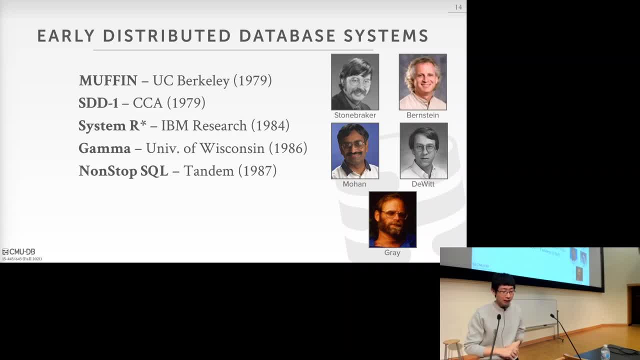 That came from again also came from 1979, but from this second person called Phil Bernstein, which actually is the inventor of many of the concurrency control algorithms for distributed database system right. So he also has a kind of like a famous concept. 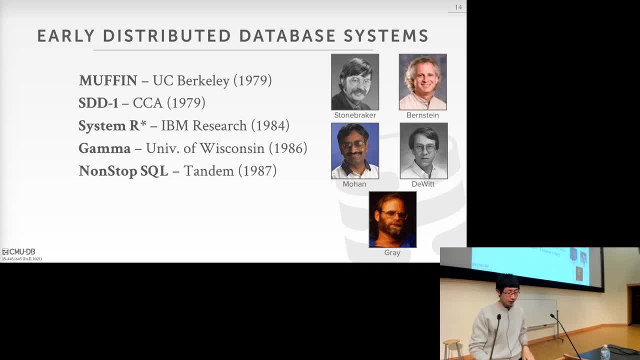 or proof of concept of distributed system in that era. But then of course, like we mentioned many times in this class, system R has the original implementation and algorithms for many of the current implementations and design of database system today Here. similarly, system R in 1984 also has a different 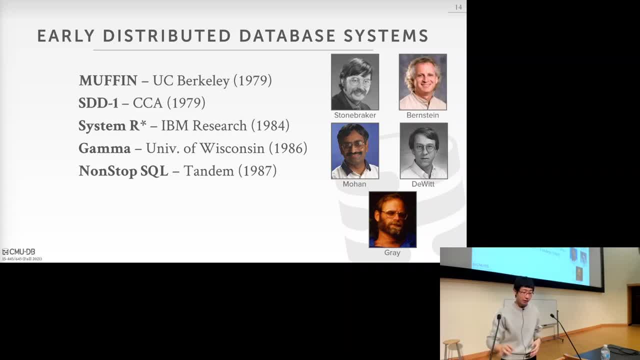 version, or like a new version of the system called system R star. have this distributed database system capability right. And then there are also another academic version of distributed system from University of Wisconsin. it's called Gamma. that's mostly led by a famous professor there called David DeWitt. 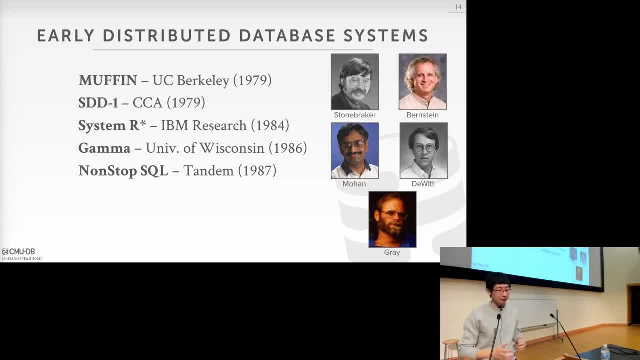 By the way, for in system R, many of the distributed database system work was also led by this person called Mohan right, Which would be the author of the ARIES paper that we talked about last class, And lastly, the Turing Award winner, right Jim Gray. 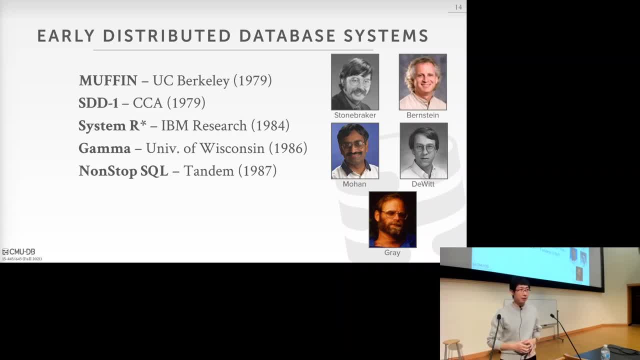 he also was, like, very involved in the development of an early distribution system, right, This distributed database system called non-stop CQ, and it came from a company called Tandem. I think right now Tandem is already through multiple acquisitions. 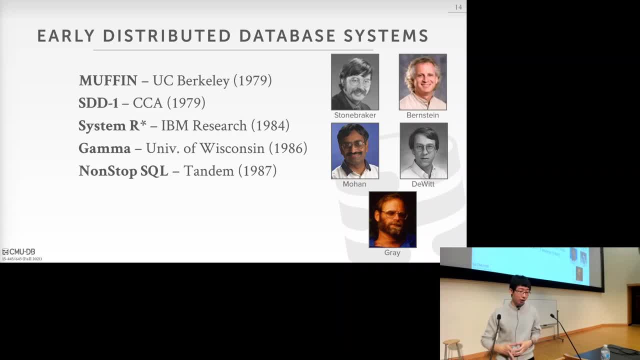 right now, Tandem belongs to HP, but he also has a version of distributed database system that is actually still running today, right, This non-stop CQ, I mean, invented by this Tandem company. Right now, of course, there's not really new features. 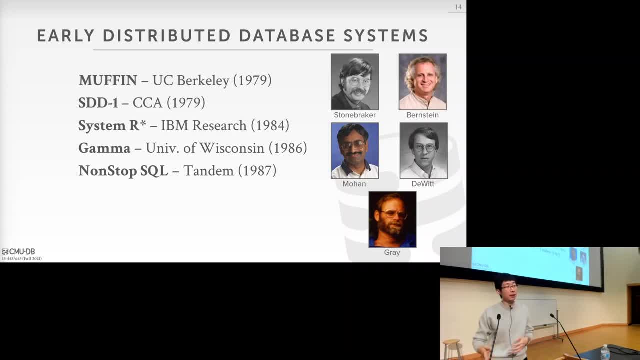 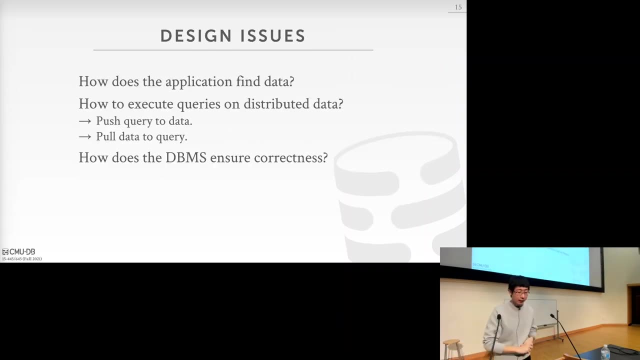 added to non-stop CQ, but the system is actually still used by some applications today, but mostly in maintenance mode. already. all right, So that's the history of many of the early implementations of distributed databases. So for today's class right we are going to talk about. 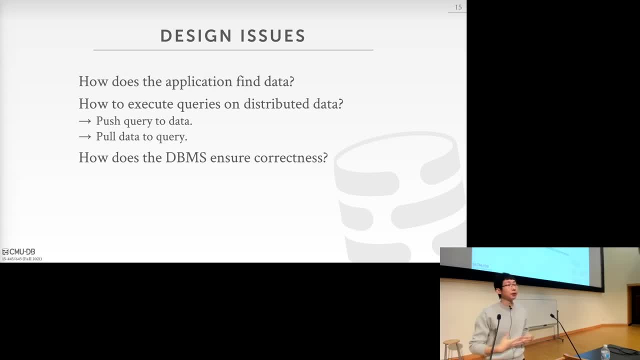 now we are going to talk about a few design issues when we want to build a distributed database. So at high level, right, we are going to first talk about three questions. The first would be how the applications, how do the applications find the data right? 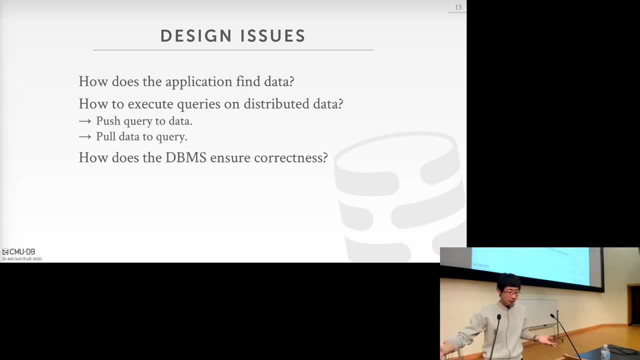 How does the application know which node or which location the data is on? and then how do the queries execute if it finds that the data it needs to access is not on the same machine, right, Either shared nothing or shared disk, how does the query going to get data remotely? 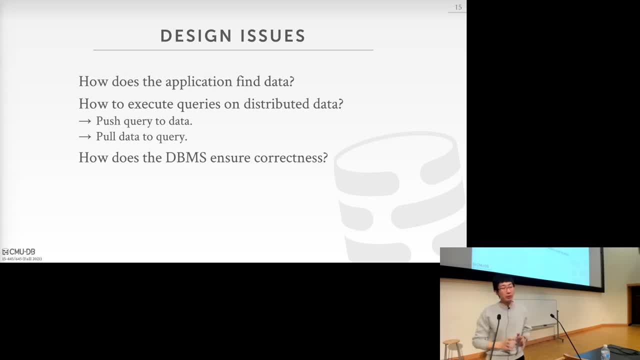 And lastly, I mean how does the database system is going to ensure that, when executing queries, especially transactions across different machines, to ensure the correctness of the data right? And then also beyond these basic no like, beyond these specific topics, 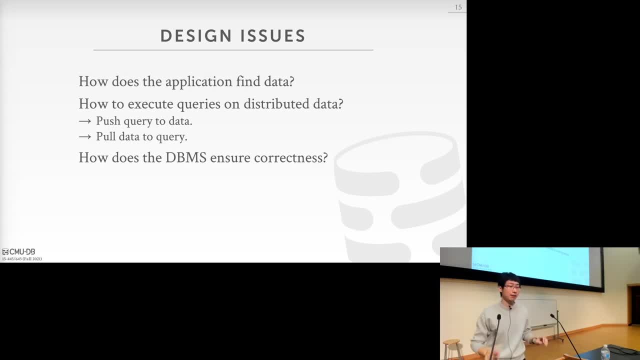 one central thing we have to deal with in distributed database system world is that I mean nodes can have failure right. So beyond this specific issue here, we also need to keep in mind that when a failure happen, one node goes down, or if we 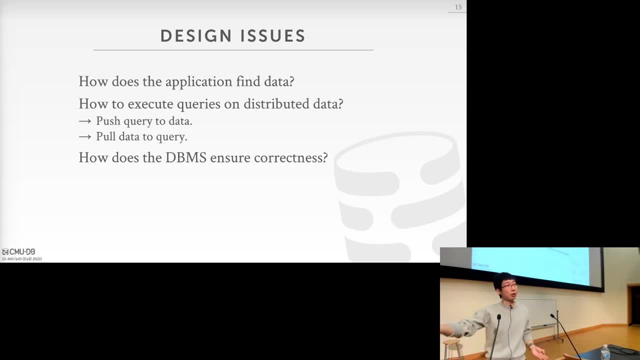 or in other cases we may need to add a node right. So when node go down, we want to replace node or we want to add new node. how do we need to deal with those decisions, as well as the execution of the entire system? 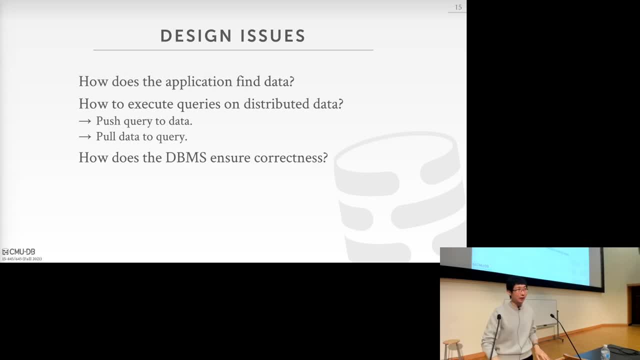 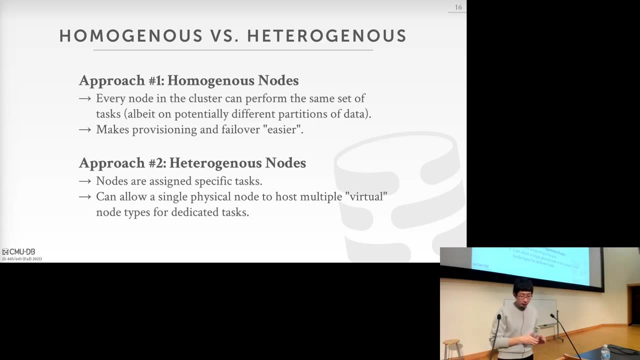 All right, that's kind of the the challenges or the scenarios that we have to think about when we're trying to build a distributed database. So okay, so the first topic I want to discuss is that there could actually be a choice among how you organize or assign roles. 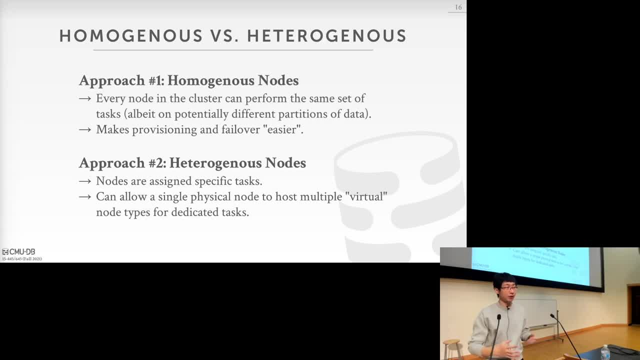 to different machines in your entire cluster of machines in the distributed database system. So at high level there will be two different choices. The first would be called homogenous node, which would mean that every node in your clusters of machines in your distributed database system. 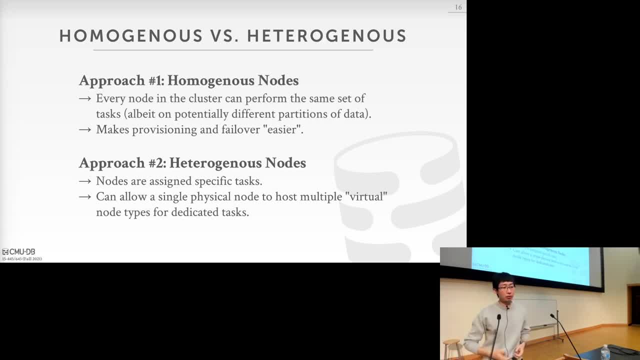 will actually have the same responsibility, right? So every node will be: handle reads, handle, writes, handle the transactions, et cetera. I mean every node goes down. I mean you can create or spin up a new node. 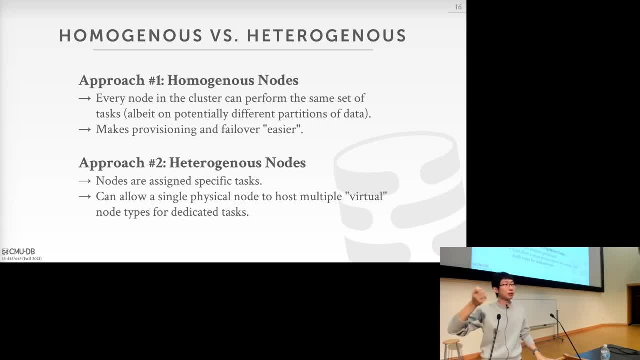 and this would be exactly the same. or has exactly the same responsibility as other node and this would be exactly the same responsibility as other nodes. ]. has exactly the same responsibility as other nodes. at that point or at the same time, the system right. 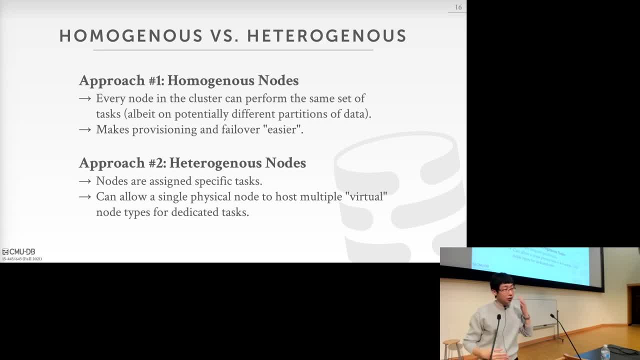 So, obviously, one advantage of this is that it's easier to provision new node as to resolve the scenario from a failure, right? Because, like I mentioned, if you add a new node, well this new node from a functionality perspective, 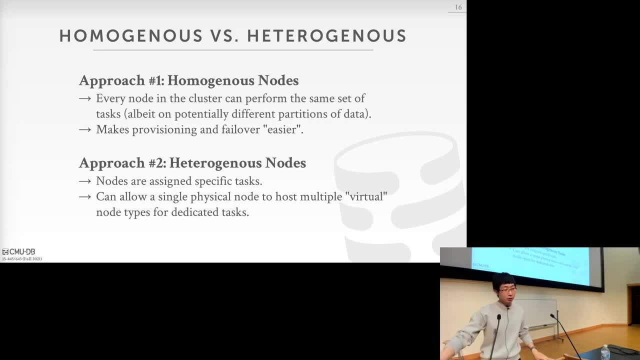 would be exactly the same as other nodes, right? If one node fail, you create a new node, then I mean this new node would exactly be able to take up the responsibility of the node that failed. So, in contrary, a different approach. 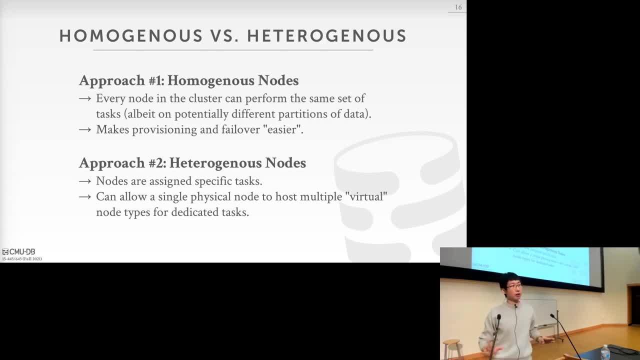 would be called heterogeneous node, which means that different nodes in your cluster of distributed database system may actually have different roles, right? For example, some nodes may have read-intensive queries. Some node may be able to handle write-intensive queries, For example, for those that write-intensive 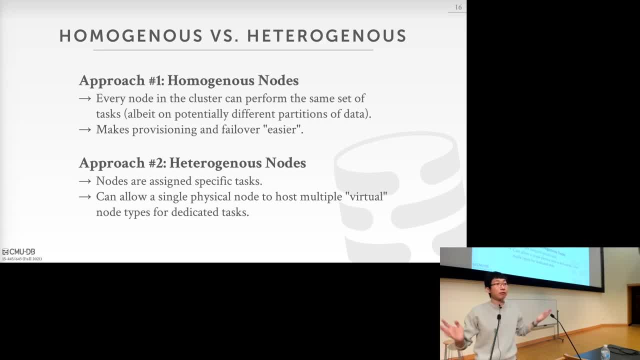 for the nodes that handle write-intensive queries. it may even have a faster disk, right. And then some of the node may even just be responsible for handle concurrency control et cetera, right. So in this heterogeneous, in this heterogeneous scenario, 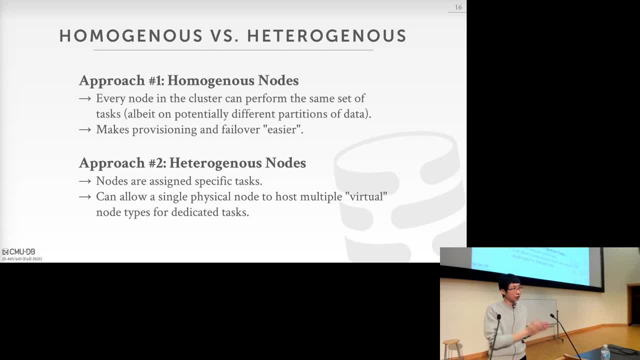 then the advantage is that you can kind of specialize different nodes for different purposes, right? So potentially have a better efficiency of different nodes based on the task you need to do. But then the obvious problem or challenge of this heterogeneous approach will be that 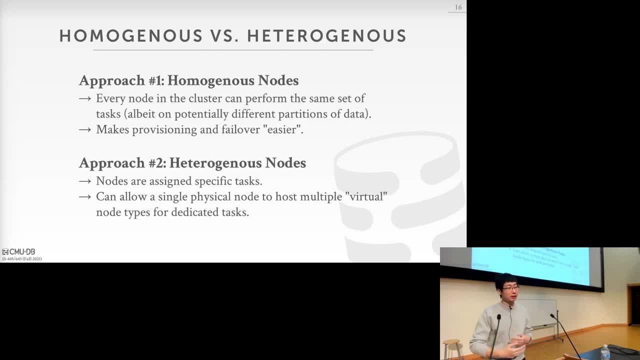 depending on what kind of a responsibility a node is taking. then when a node fail, it may be difficult to recover from that and then create a new node that exactly takes over the responsibility- right If the responsibility that this particular node that failed. 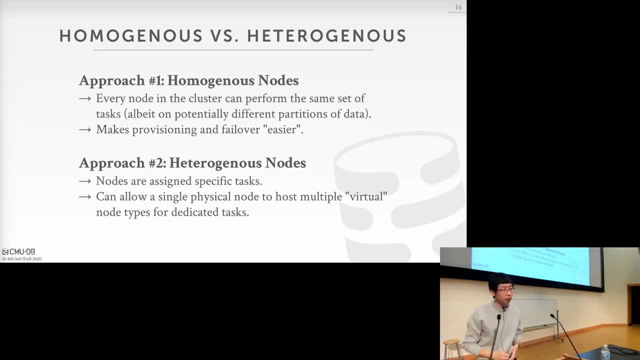 taking is like a challenge or difficult right. And then another thing to note in this second heterogeneous scenario would be that one physical machine may actually be responsible for a different or a number of virtual nodes as well. right, For example, if one physical machine is very, very powerful. 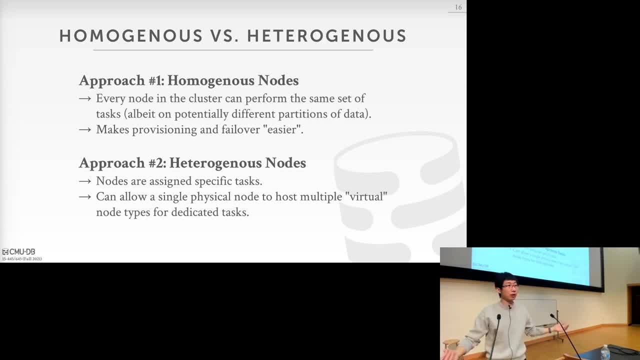 it can be responsible for both read and write. So it can have- there could be- two virtual nodes on that physical machine, one responsible for, for example, read-only queries and the other responsible for write queries. I mean you can assign the task of different nodes. 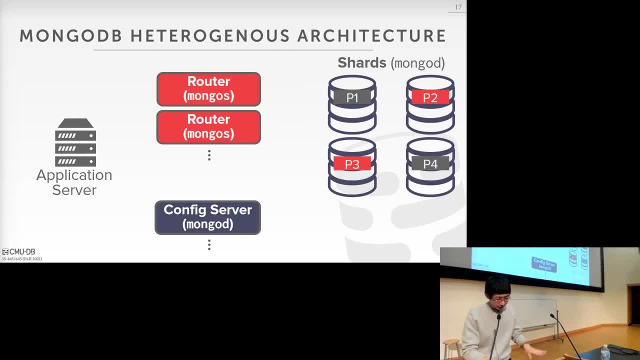 to the same machine as well. all right, So let me give you a more specific example with this heterogeneous architecture. So the example here I'm showing you is actually a NoSQL system, right? Not really a traditional relational database system. 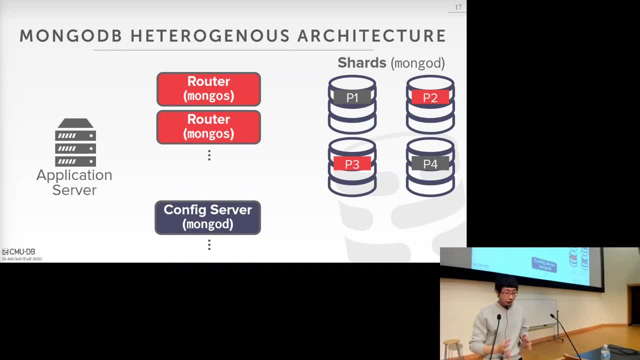 So this is actually an example of a MongoDB. all right, So MongoDB would be a heterogeneous architecture, but by the way, it's actually a shared nothing architecture. So this is kind of like orthogonal right, Whether you design a system to be heterogeneous. 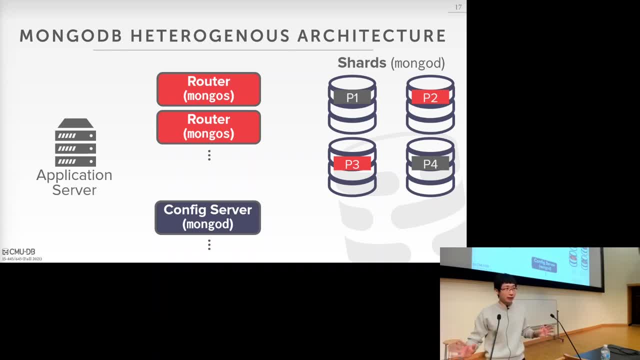 or homogeneous. the architecture would either be a shared nothing or shared disk right, So that kind of like a orthogonal design choices. So in this case, as I'm showing you on the right, I mean in the MongoDB architecture. 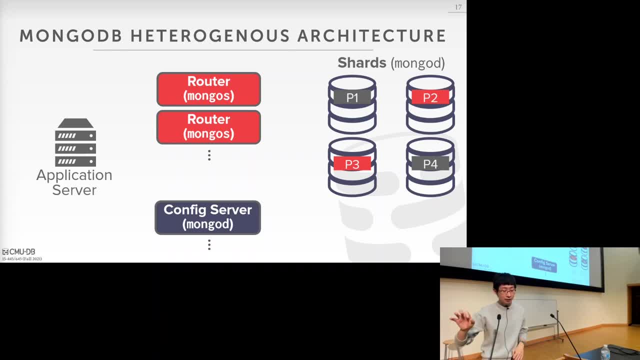 the data and the CPU and as well as the memory, would be on these different nodes called shards. I mean you can think of them as the partitions of the data, all just like a node, as I mentioned in the earlier example. 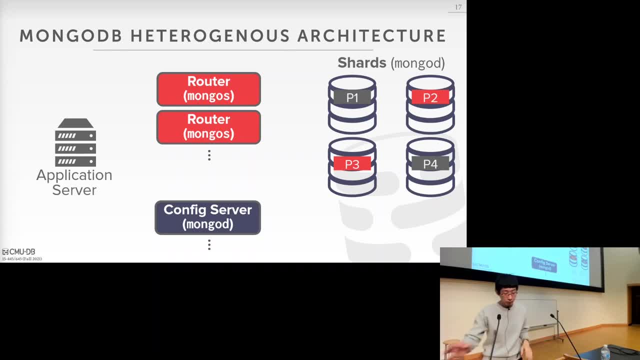 right same meaning. So in MongoDB part end they call them shards, and then we have four shards or four partitions. But then beyond these shards they actually have two different type of heterogeneous nodes, right? One type would be called router node. 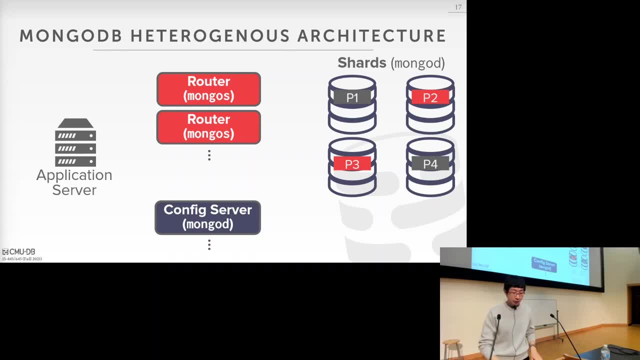 The other would be called config server node right. So what would be the result for them? See that one query is trying to read a tuple with ID 101. Then in this MongoDB architecture all the queries would actually be sent to this specific router, nodes first, right. 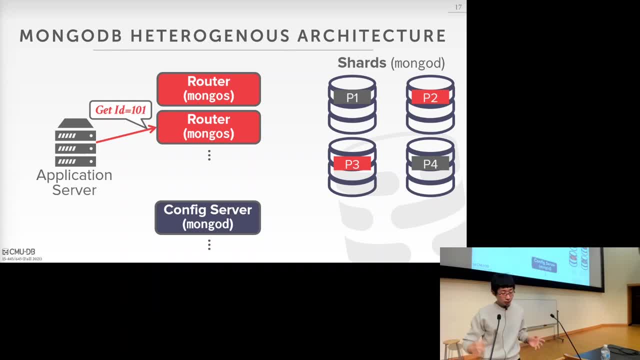 And then the router would only be responsible to figure out, or to not actually to figure out yet, but be responsible to route the queries sent by the application server to the corresponding shards or partitions that would contain that data. all right, But then, when the router tries to do that, 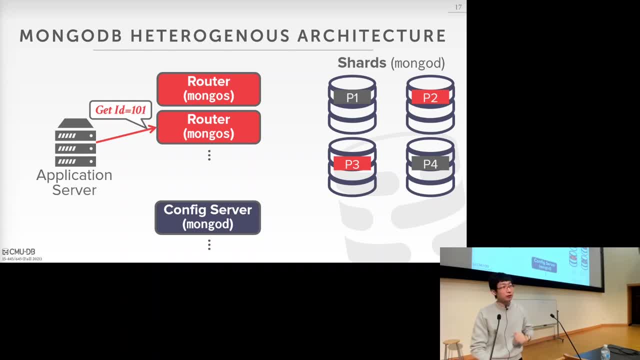 it actually needs to consolidate the locations of different records, different data, with a centralized config server right. With a config server, we'll have the information of the state about which record or which page will be on which partition, and the router would be all go to this config server right. 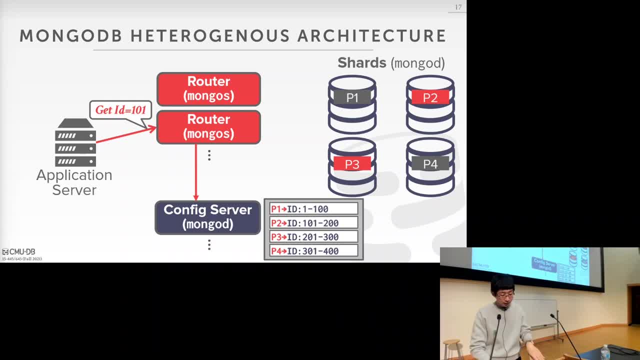 Read the state table from a config server. say that we have four partitions and different tuples on different partitions and then, after config server figure it out, it will send this information about which partition or shard the router should route this query to. I mean back to those routers. 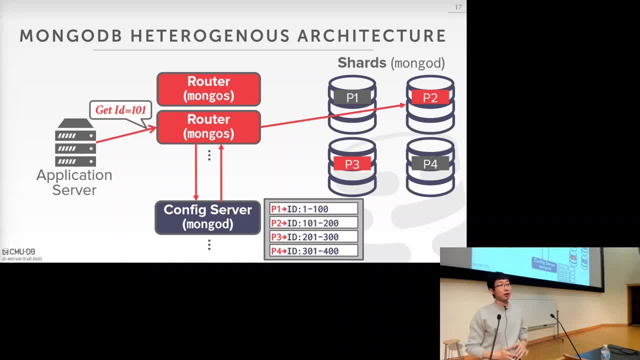 and finally, I mean route to the correct place, right? Well, the router is only responsible for directing the location or directing the direction of queries, and the config server would store all the states of the locations of data on which shards and the shards would finally be responsible. 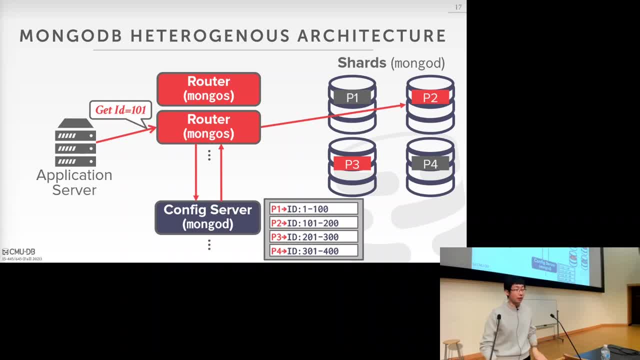 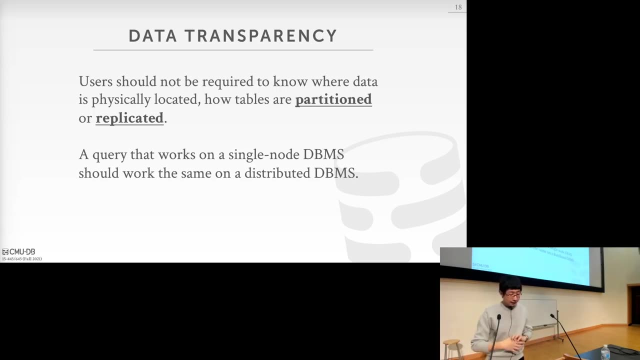 to read the data and executing the query right. So this is an example of the MongoDB architecture, and different nodes would have different responsibilities. all right, Make sense, Nice, Okay. so that's the first design decision and the second design decision. 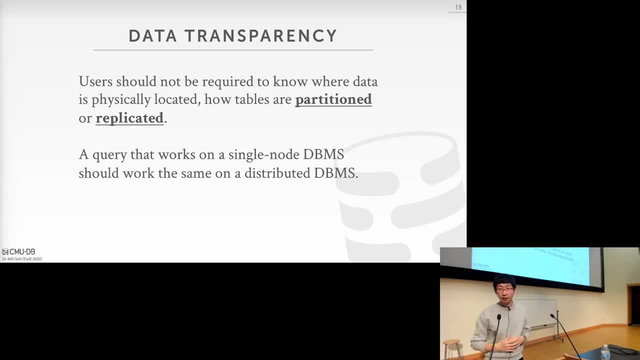 or actually not really before, not exactly before we talk about the second design decision. a important concept here we want to achieve with distributed database system is that the users of the distributed database system should actually not know any data right. They should not know any data right. 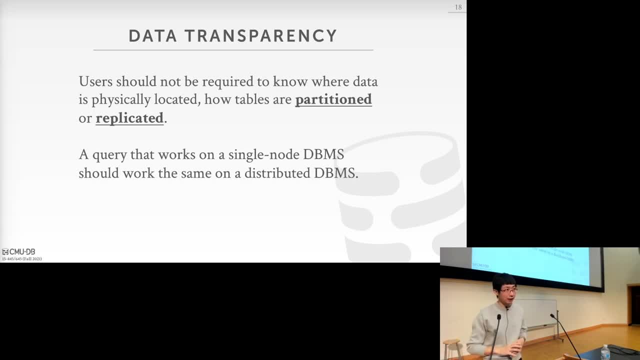 where the data is physically located, right. I mean similar to the when we talk about concurrency control. well, similar to the concept when we talk about concurrency control where we say we want the database system to handle all the scenarios where there's a dirty write. 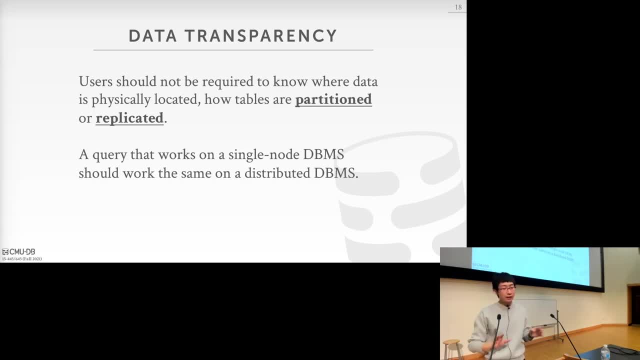 some system failure et cetera, where the users don't need to worry about locking the data and only need to focus on the core logic of the application. Similar here in a distributed database system scenario we don't really want the users to be worried about. 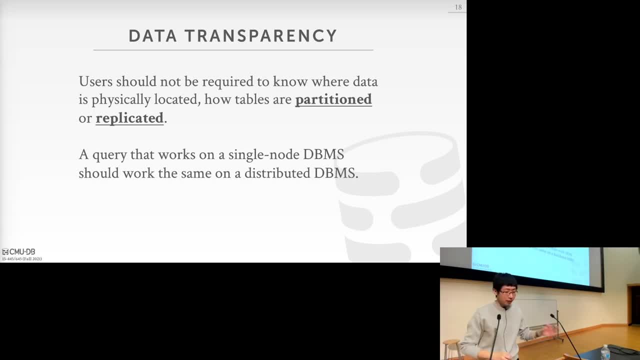 hey, which part of the data is on which machine, or whether the data is partitioned in different machines or even replicated on different machines. We don't want the user to worry about any of those things. We want to handle all those things for the users automatically. 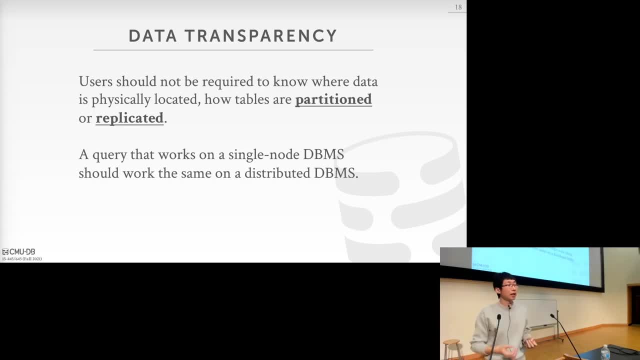 so that when users write a query, users doesn't really need to know- hey, I'm writing this query to a single node database or a distributed database. The system will actually hide all those implementation details from the user, so that the users again. 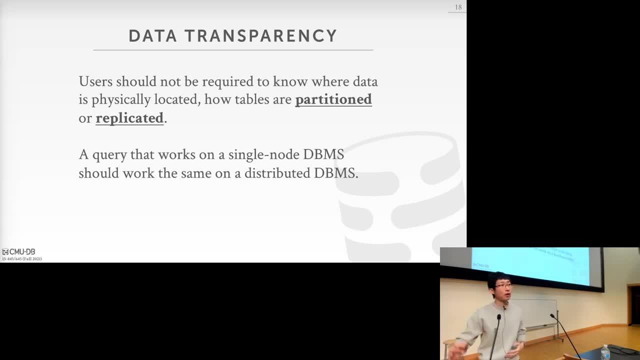 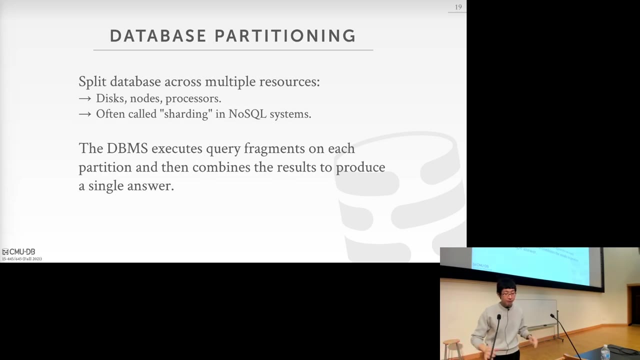 can conveniently store and access their data and then focus on the core logic of their application. So one important notion related to this that the distributed database system need to deal with is that, like I mentioned, it needs to be able to automatically figure out. 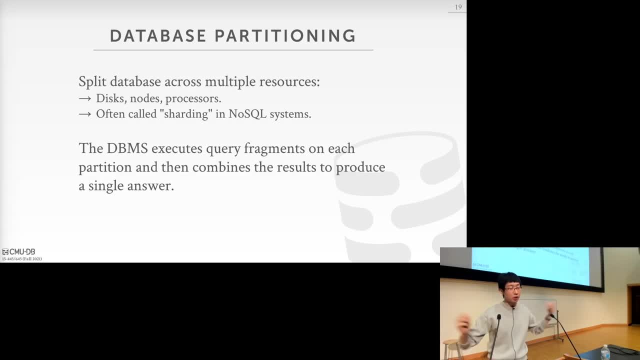 how to partition your data to different machines in the cluster of a distributed database system, as well as automatically figure out how to read and write data from those partitions. all right, So when I say a distributed database partitioning, that's actually a term more often used. 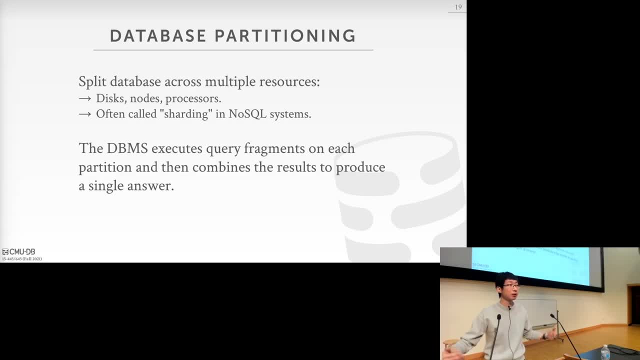 in a traditional relational database world, So in the newer called NoSQL database system, especially with the example of MongoDB, this partitioning would actually be called sharding, For some reason- I actually don't know why, but for some reason that's a term. 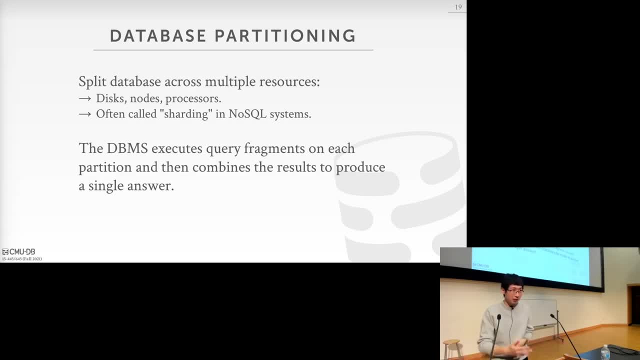 that's more often used for NoSQL system, but essentially that's the same thing: Sharding, partitioning, same meaning, And then essentially the database system needs to be able to partition the data onto different places, and you need to be able to figure out. 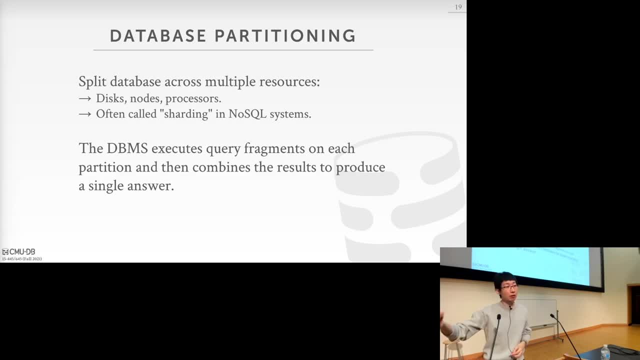 where to access data and then fetch the data from the correct sharding or partitioning appropriately and then finally aggregate the results and send back to the user right. So the users would be similar to the scenario to write into a query to a single-node database system. 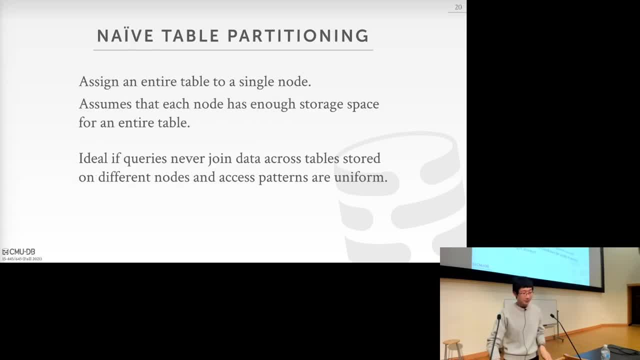 You shouldn't know that the data is distributed. Okay, So the first partitioning approach to do this- or, as I wrote here, we can call it naive table partitioning- would be that the database system could choose to put all the data related to one specific table. 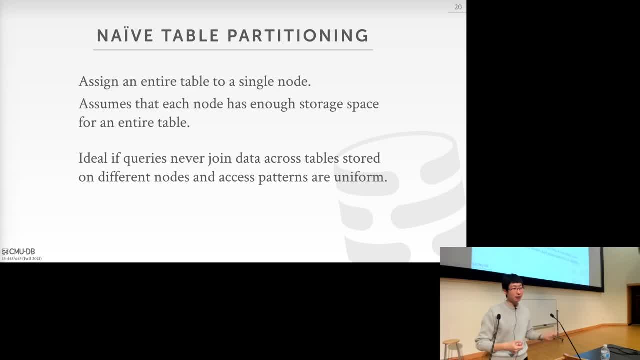 on a partition right, Just like one machine is responsible for one table and the other machine could be responsible for the other table, And of course this would be under the assumption that every machine will have enough disk space that handle all the data from a particular table right. 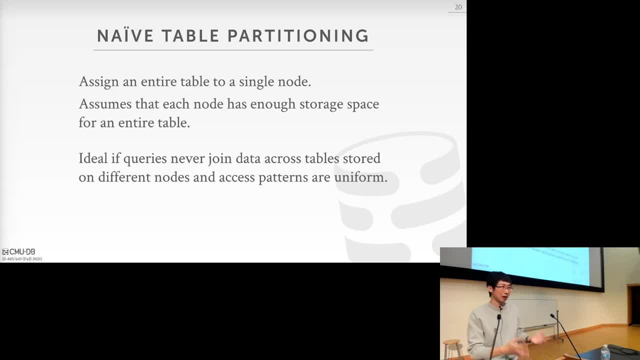 If a table is bigger than the maximum of disk space allowed on a machine, then this simple approach doesn't work. And another thing is that the scenario where this approach works the best would be the scenario where you don't really have a drawing query across different tables. 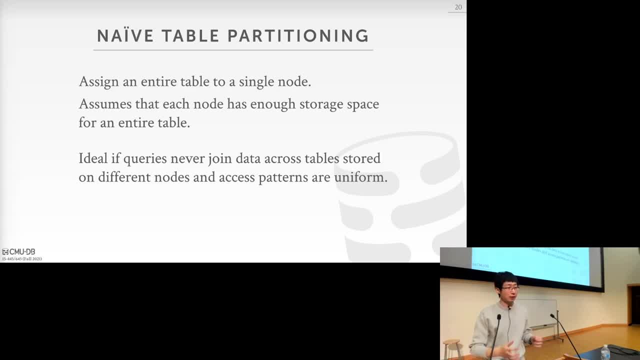 or you don't have too many drawing query across different tables, right, As well? as if the distribution of this right distribution of these queries against each table are kind of homogeneous or uniform, then this approach would actually probably work well, right? 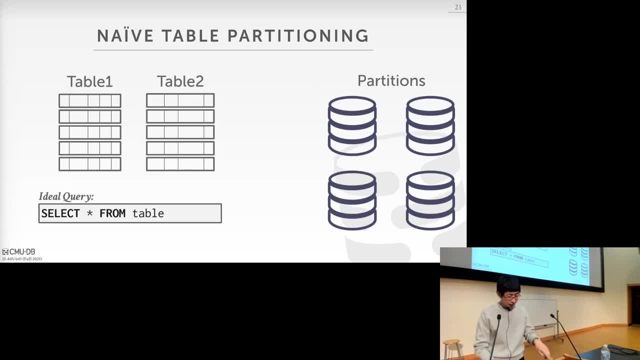 So I'll give you an example of this. right, Say, I have two tables, table one and table two. then with this naive table partitioning approach, right, you could just put, for example, table one, all the data onto this first partition. 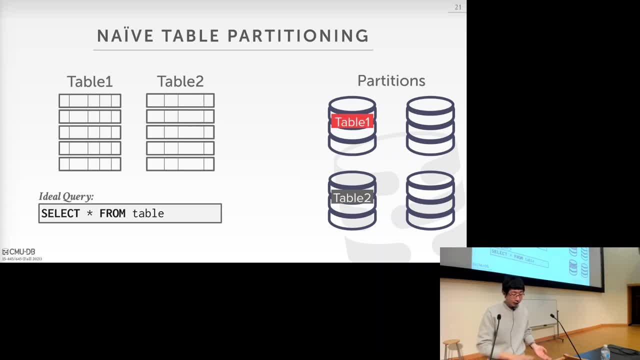 and then table two, all the data on the second partition, And then the ideal query for this would be that you always, always only looking at data from a particular table at a time right, You don't really have too many drawing queries. 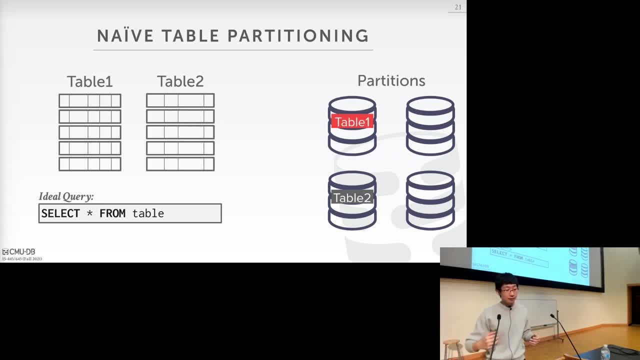 So, because of this limitation that every table must be able to fit the storage space of a specific node, as well as this scenario where I mean if you have drawing queries or if you have queries that don't really have a uniform distribution against different tables, 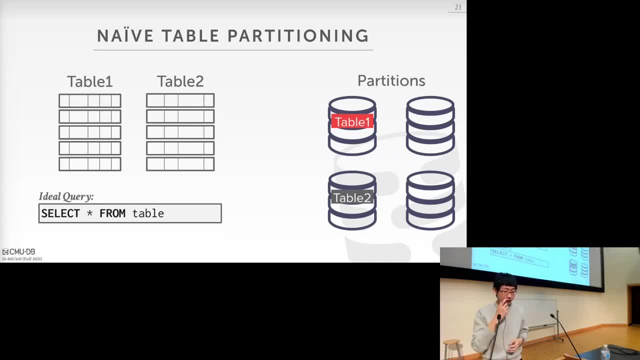 I mean the performance may not be very good. Actually, in practice, most of the system would actually not, as you can imagine. sorry, most of the system would actually not use this naive table partitioning approach. But then there's one system actually: MongoDB. 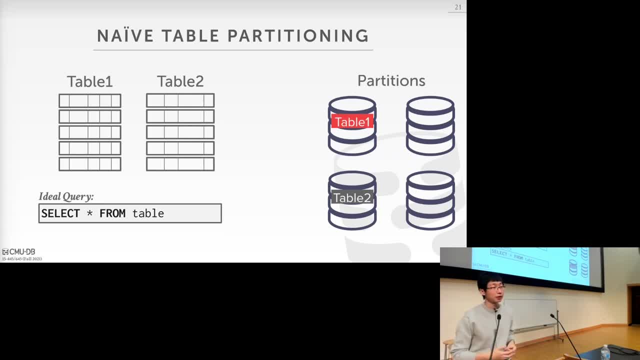 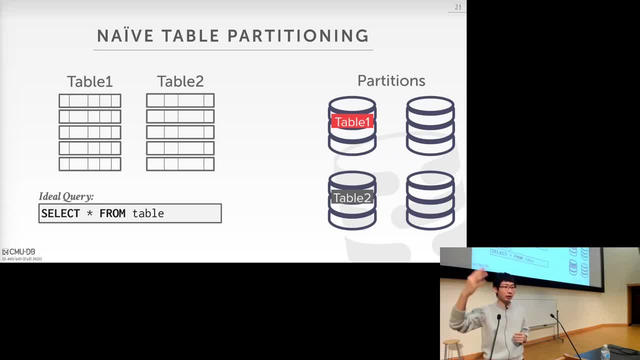 to a specific table, right, so we can think of this as a matrix or a logging store, right? Then, if there's a workload, there are a bunch of queries only appending logs to the end of the one table and they never, or rarely, read any data out. 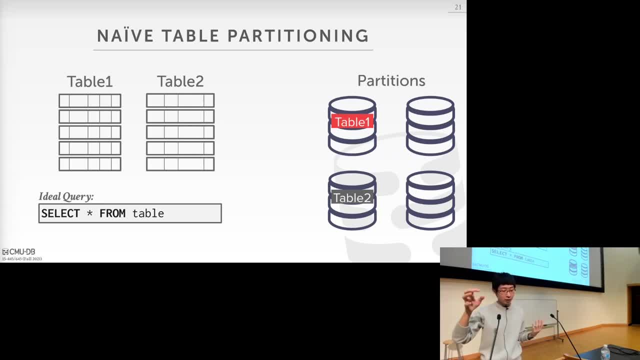 then you can think of, you can imagine a system where they have a designated sharding or partition for that specific table, with a better disk right, a faster write speed And then if you only write to the disk and never and rarely read back again. 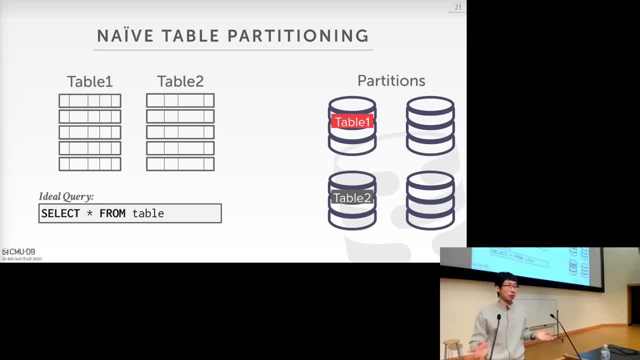 then a faster disk would probably- or at least a disk that is faster on write would probably help you on that scenario, right, And then other transactions or queries can use other nodes in the system and don't really be affected by the write operation here. 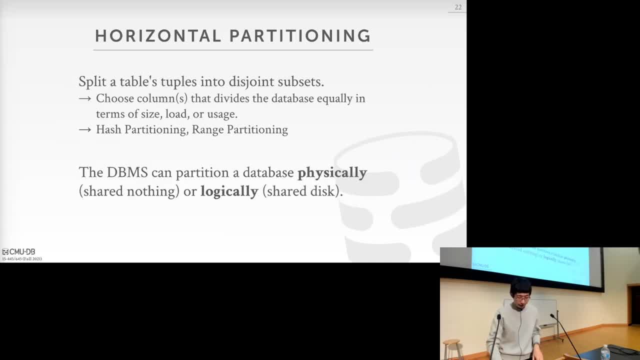 right. so that could be one example of use case. Okay, so what would be a more common approach, Again probably suitable for more general scenario- would be called a horizontal partitioning right. So in this case, instead of putting each of the entire table on a specific node, 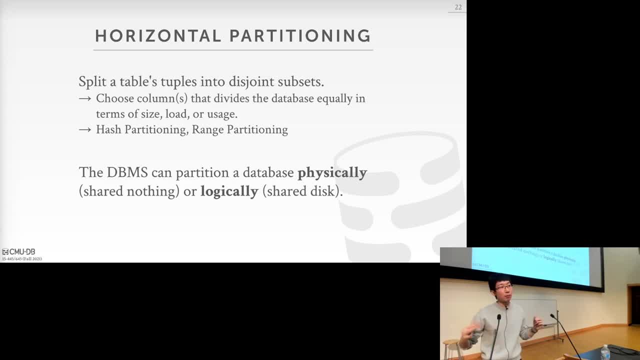 what you would do here is that you are going to split the tuples from every single table across different nodes, right? And then, of course, you want to be a little bit intelligent about how you are going to split these tuples, right, For example, you could try to balance the size. 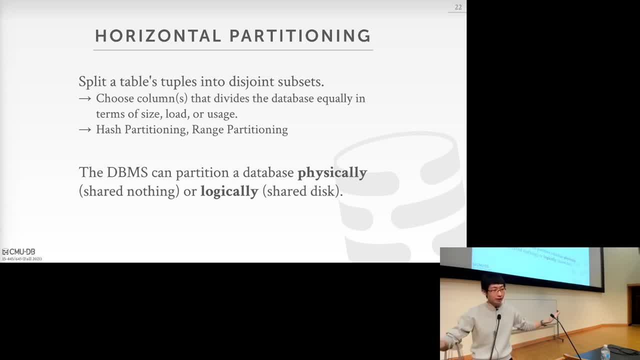 of the partitions of the table among different partitioning or shardings to be like a equal, or you can also try to balance the load of the queries that are going to- I mean access data against different partitions of a particular tuple to be roughly uniform or balanced right. 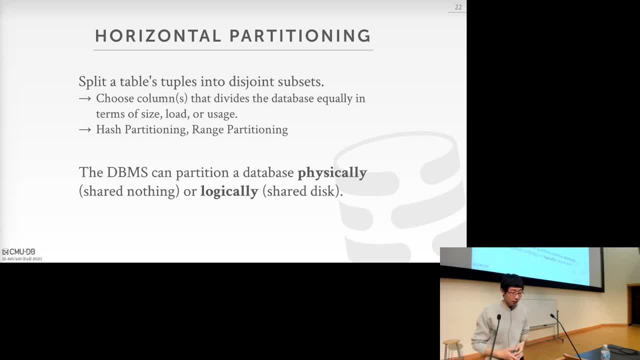 And there are many intelligent decisions you can do with this- horizontal partitioning. And then the two common approach would be called hash partitioning and then range partitioning, which I will give some specific examples in the next few slides. And then, lastly, one thing to note here is that 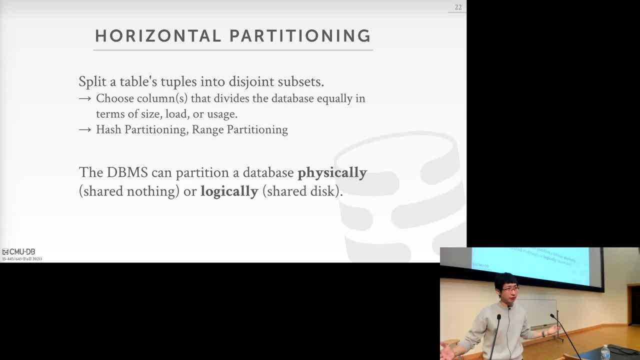 when the database system partition the data horizontally, it doesn't necessarily mean that the different partition have to be on different machines. So I mean one scenario would be a physical partition would be a very common in the shared nothing system where you indeed actually for different partition. 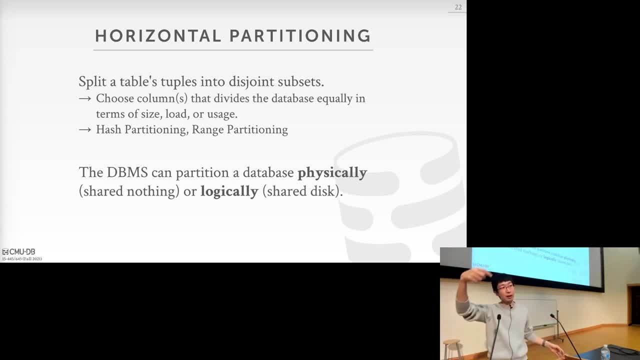 they're going to be on different machines attached to different local memory compute as a storage. Then there could be a logical partition as well, right? Typically seeing a scenario where you have a shared disk system even though you can partition the data right? 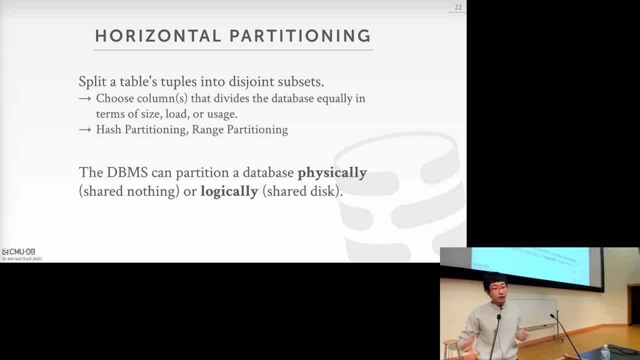 In different portions or chunks, but then they could be all the partitions would be, reside on this big pool of storage space, right, You know? shared disk scenario behind this network, And then they could be on the same machine, could be on the different machine. 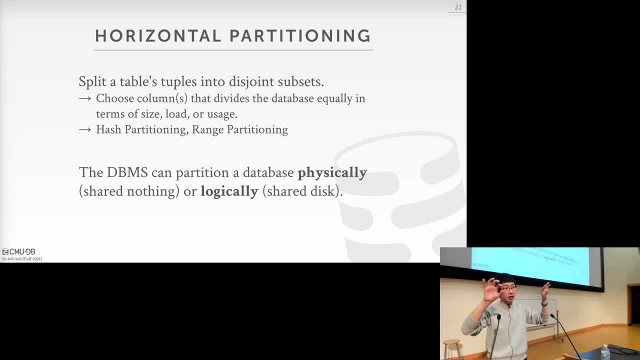 depending on how this shared disk architecture of this shared disk space is going to manage that. But then what you can do is that for different compute node right They can be responsible for handling the queries directed to different shards. But then in this case there's a sharding or the partitioning. 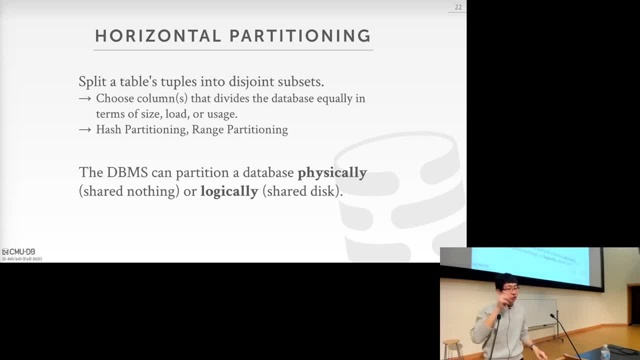 it would actually be logical right. So only like, at a logical level, which computer node should be responsible for the queries against which part of data. The data themselves could be on the same node or same physical node or different physical node, It doesn't really matter. 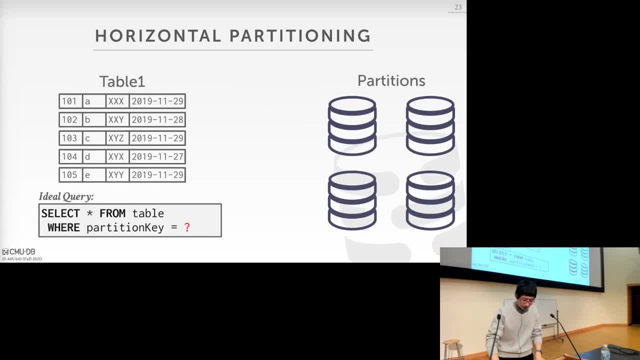 All right, make sense, Okay, nice. So let me give you an example of this horizontal partition right. Say: here I have this table right With the four attributes And the first thing you need to do is that you have to choose a partition key right. 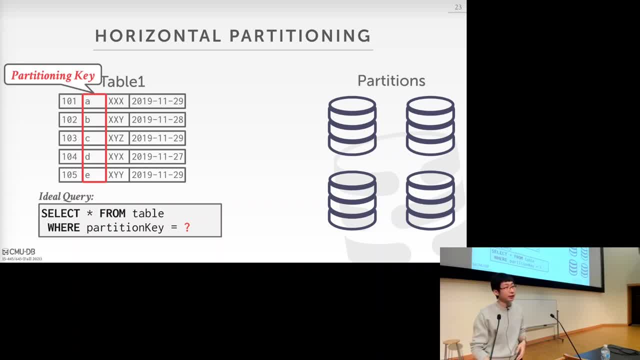 Like, for example, here we choose the second attribute of this partitioning key And then one simple strategy like I mentioned here would be one simple strategy you can use would be hash partitioning right. So in this case you would just- I mean, 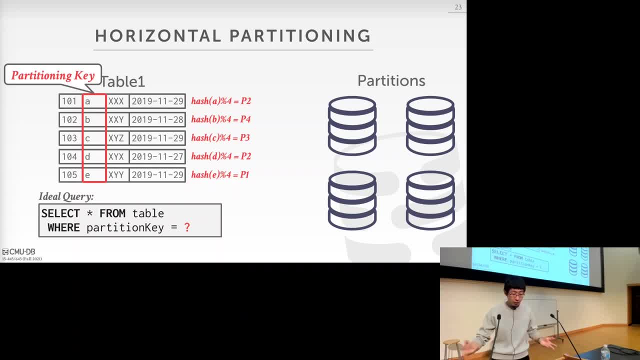 apply a hash function or all these values. And then I mean one simple thing you could do is just to mod the hash value by the number of partitions or shards that your database system has right, In this case we have a four system. 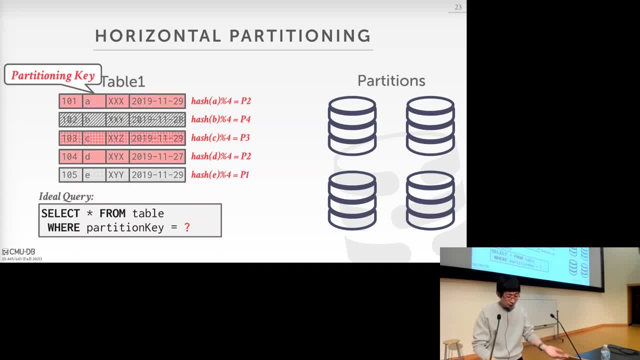 And then, after a mod, the number four, you can have different- I mean assignments of these different partitions right As illustrated here, And then, assuming that you have a query that have a where clause and it contains this partition key right. 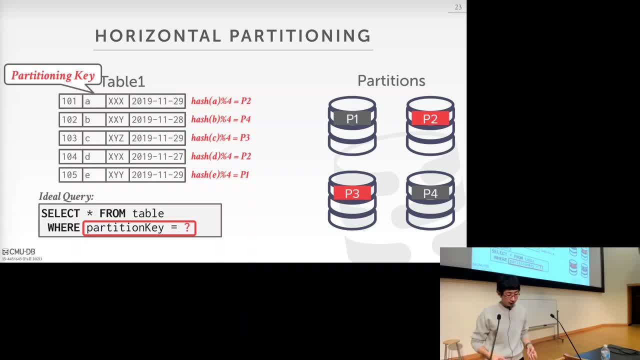 Then you can just hash the value in this where, clause, And then I mean again mod, by this total number of partitions or shards, And then you can locate the corresponding machine right, So you can. that's how you find where the data is. 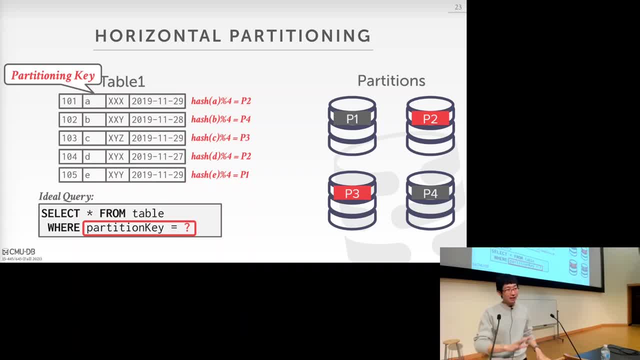 in this horizontal partitioning And, of course, as you can probably tell already, in this horizontal partitioning it's very, very important to choose which your partition key is right, Because if you have a sharding or partitioning, I mean distribution. that where many of your queries. 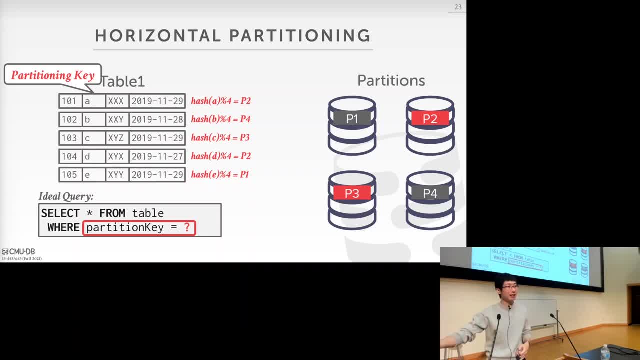 don't really have an attribute in your where clause contains the sharding key, then what you have to do is that you have to broadcast those queries- right? Don't have this partition key in where clause- to all the shards to find out where your query is. 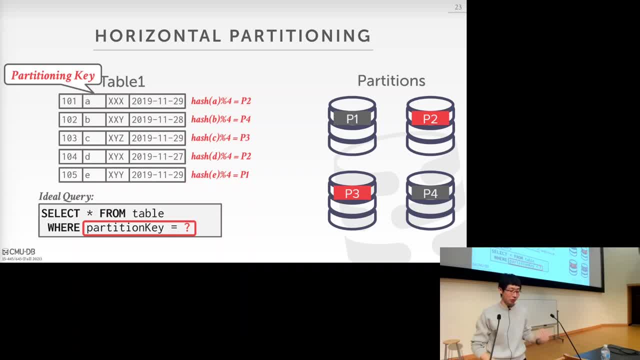 Sorry where your data is, And that could be potentially expensive, right? So this choice is very, very important, all right. So another challenge we may encounter in this simple- at least a simple- hash partitioning scheme is that what if say, right now again: 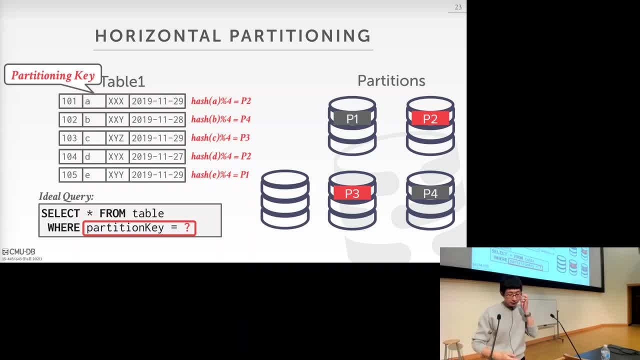 independent of whether I'm doing a shared nothing or shared disk right. Actually, in this example here I'm illustrating more a shared disk- sorry, shared nothing scenario. But one challenge here is that what if I want to add a new machine right? 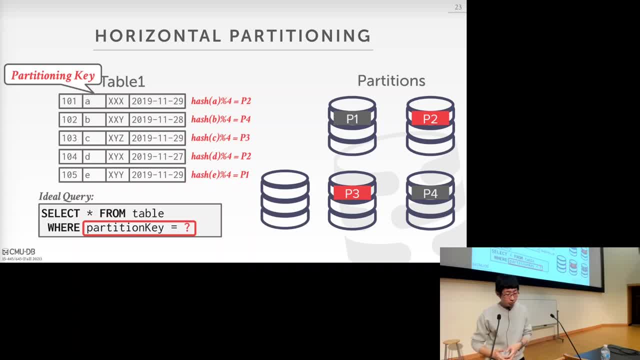 And then right now, the number of shards or partitions will actually be five. Then in this case, pretty much, I mean most of the values, I mean after this hash, and multiplied by this number of partitions, the partition assignment, most of this assignment. 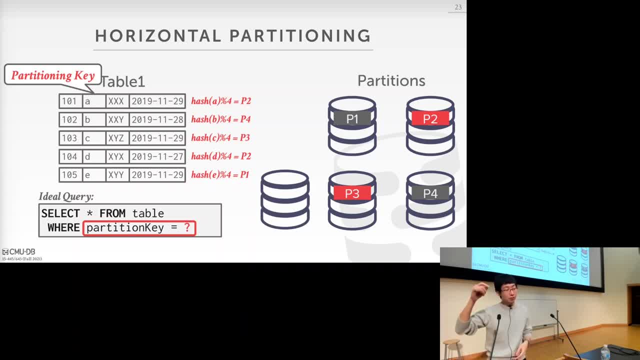 will actually change, right, And in this case, unless this simple scenario I mentioned earlier, where you have some sort of like a range-based assignment of a different number of records on different machines- Now, if you change or if you add this new node, 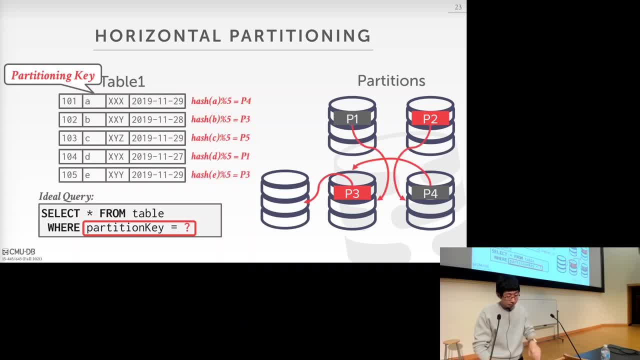 and change your equation on assign the shards, then potentially- I mean lots of things would change, And then you have to move data all around your entire cluster, right, And then put back the location, put back the position of the data to the correct location. 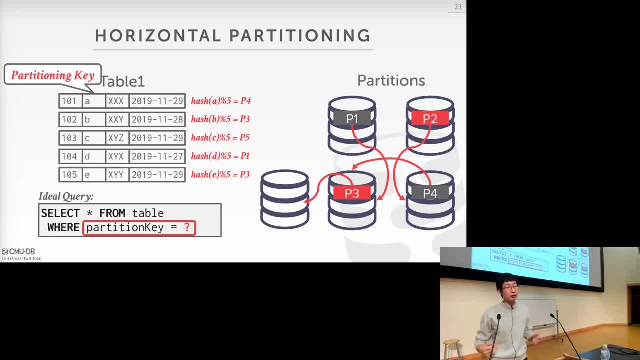 And this potentially be very, very expensive and also very, very difficult to coordinate as well. right, So that would be a challenge happening in this case. Again, like I mentioned here, it's but the choice of partitioning, which partitioning algorithm you use. 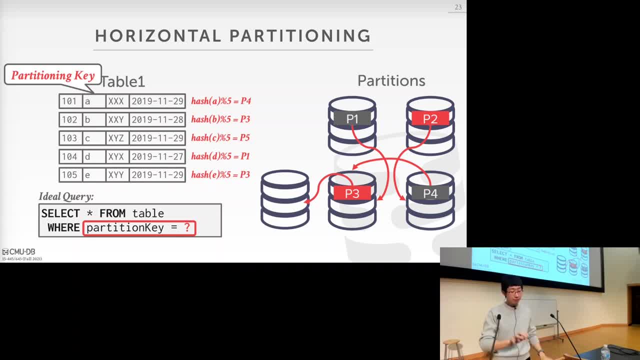 will actually be independent of whether you use shared nothing or shared disk. But, that said, this problem would actually be bigger when you have a shared nothing architecture, right, Because in shared nothing architecture, every node will have a specific portion of the data. 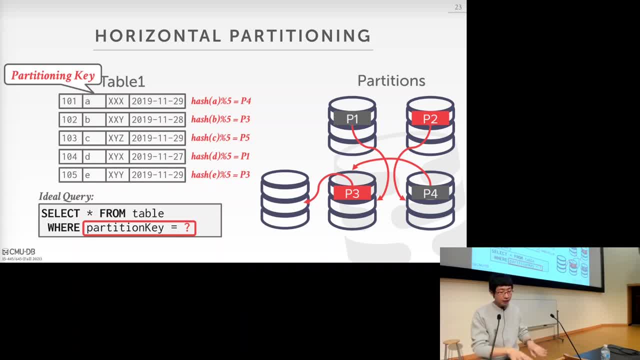 attached to it that need to be responsible for right. So there will be more of a challenge, more kind of moving around how to deal with in that architecture, In the shared disk architecture then, because everything is managed by this shared disk layer. 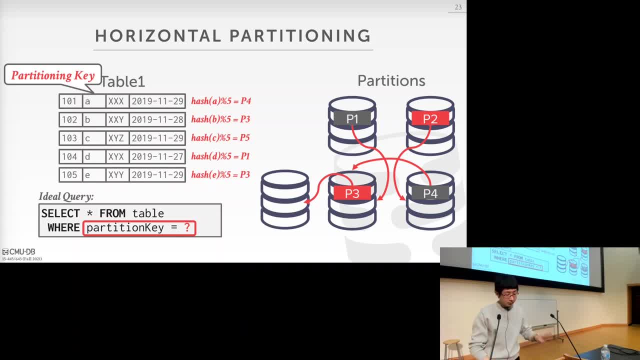 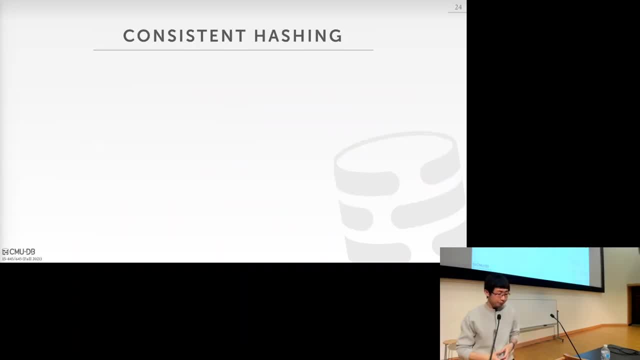 below the network layer, things could be a little bit easier. But again, similar problem you still have to deal with. All right, But potentially the mechanism would be a little bit simpler. So the approach we address this problem will actually be a very interesting idea. personally, I think 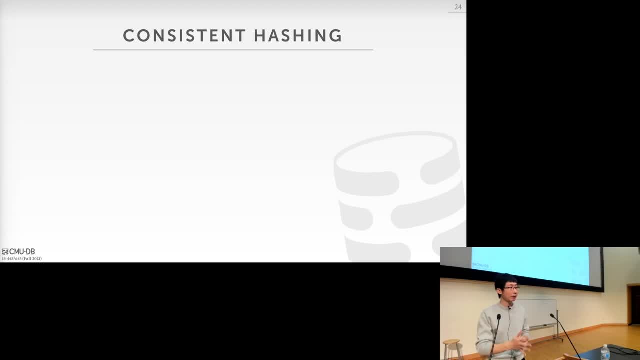 called consistency hashing right. So some of you may actually have heard of this right. So some of you may actually have heard of this right. So some of you may actually have heard of this idea of consistent hashing in some of your other. 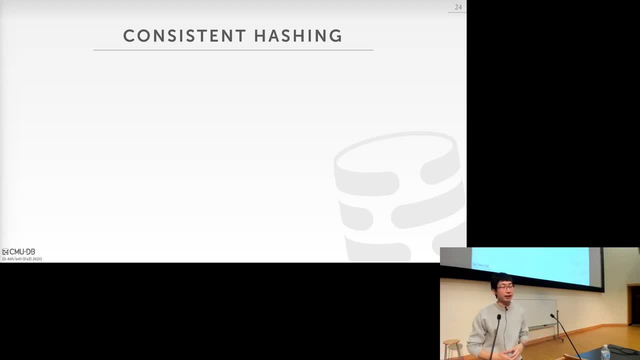 either distributed system class or other like cloud computing classes. right, It's actually a very interesting idea, came out from MIT in early 2000s, right? So what it can do is that it will actually allow you to do incremental additions or removals of the nodes. 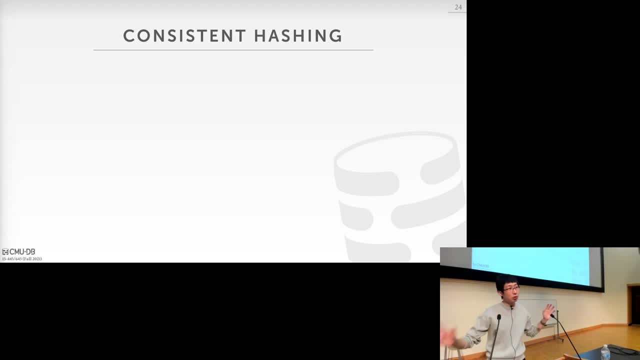 or machines in your cluster without actually having to move all the data around right, Destroy the assignments of everything. So the let me use really, this is really high level idea, right? The idea is that instead of having this function, that mode, the hash value by the number of nodes, 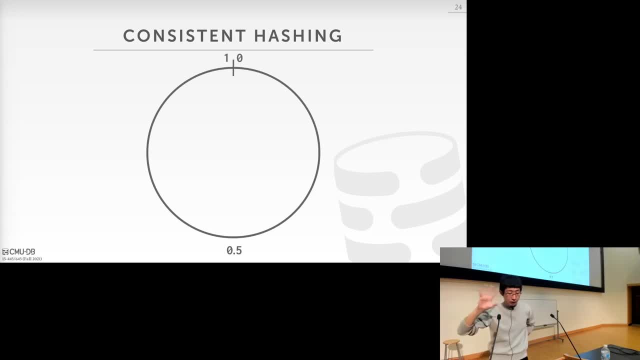 what consistency hashing is that you would actually have a, mentally would have a ring That would either map all the hash values to right And this ring would be between zero to one right. I mean, look at this username here. 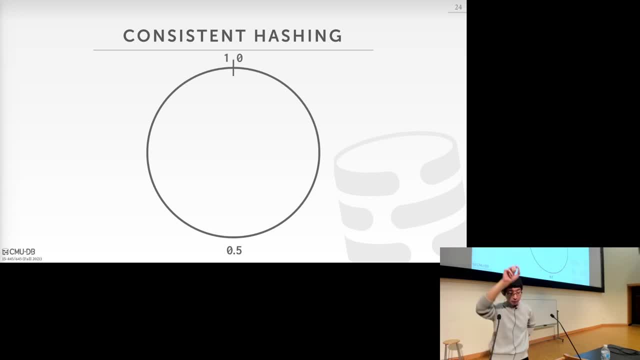 And you think about that. we have a ring of values From the top zero and one right, And then a clock- Yeah, this is a clock, wise- and then zero, zero point five at bottom, and to one right, and then for each partition. 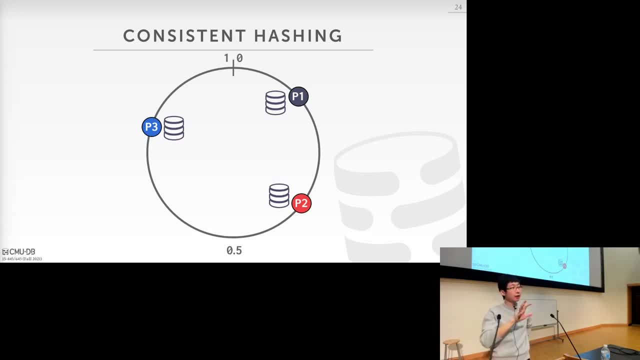 It will be actually be responsible for the hash value in a specific range in this ring Right and say we have these three locations that represent the- I mean kind of the range, that these three different partitions that it needs to be responsible for, and that this would be the. 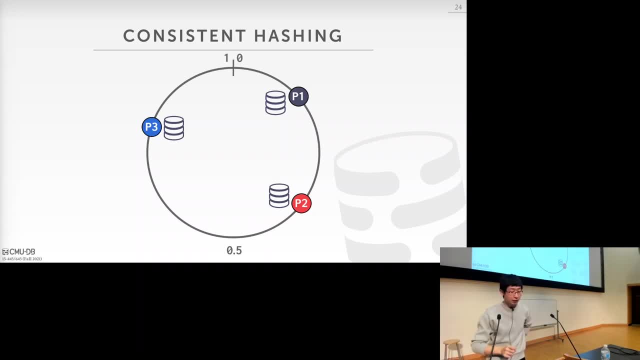 end of boundaries, of the Locations or the range that these different partitions would be responsible for. so every time we have a key that we need to hash Right, try to figure out what which partition it belongs to you actually. first, again, to hash this value between zero and one. 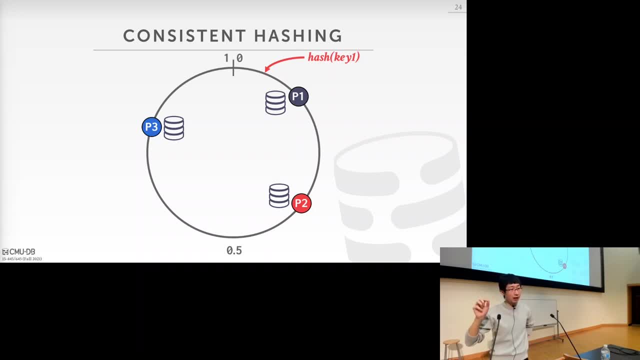 Right, no matter how many nodes you have, you always hash this value between zero and one, and then you will just Round up this decimal value to the closest partition that that related To this, to this value of this hash key. right, in this case, after hash this key one. 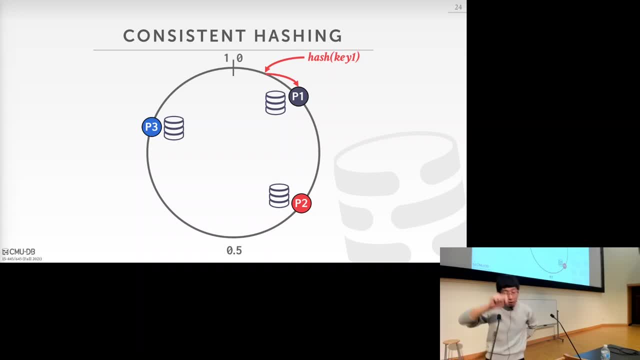 It lands, I mean somewhere at the top, and then after you round up this value, I mean this would be assigned to the partition one, because that's the first partition encounter. and similarly, assume that you have another key that would hash to a different location in this ring, and then you are round up and assigned to partition three. and then how to 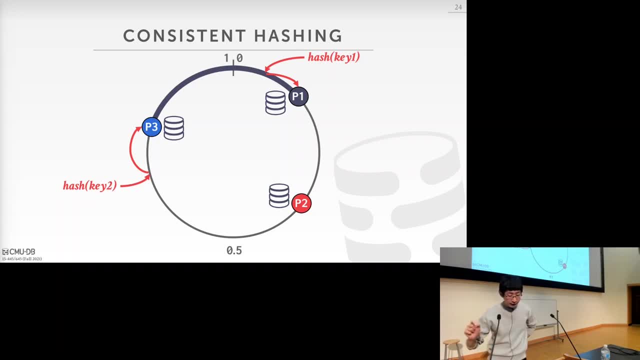 Decide and, as you read here, What this does is that essentially For this, a blue region, as I draw here right, if a key up after hashing land to this blue region, Then this key would be belong to this first partition, partition one, and similarly for all the keys. 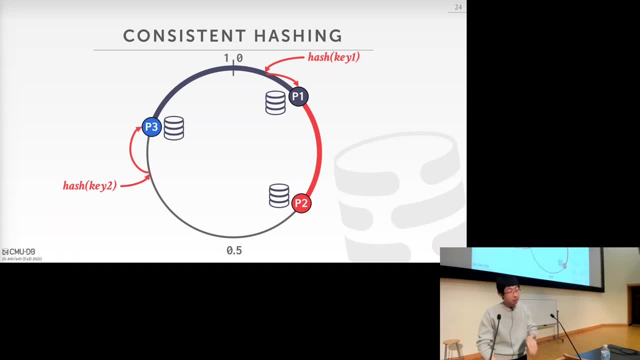 That becomes our land in this region after hashing. It'll be a belong to partition two. and similarly, for all the rings, a photo for all the keys land in this region. You'll be belong to partition three, right? So so what's good, right? 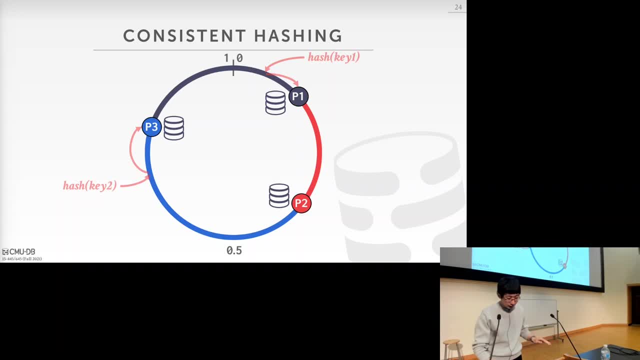 Make sense. So what's interesting here Is that what if now I want to add a new node, right, So before I need? in the old scenario where I'm all the number of nodes, I mean after I hash the key, and then I after add a new node, everything could change. 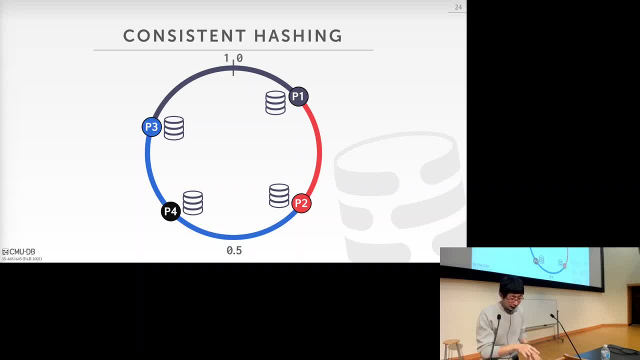 I have to move everything around now after noon, after I add a new node in this consistent hashing scenario. I just, I mean, pick a new location in this ring and typically you would pick a location that has the largest Right and then but a handle over Which is a peek, a new location for this node. 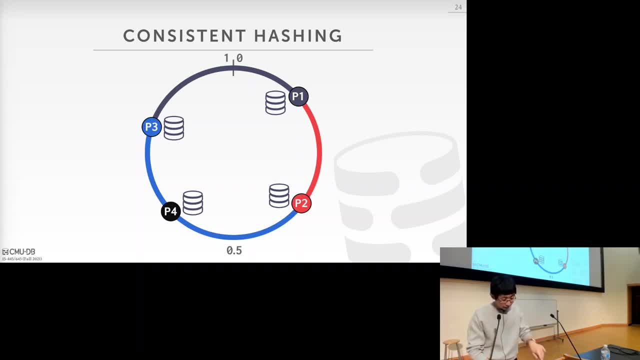 And then what you need to do is that, after you assign this location for the node, This node would be responsible for everything before that node. I'm up, I'm up until for them, But here, this before. people will be responsible for everything before and apart on tlp tool in this range, right? 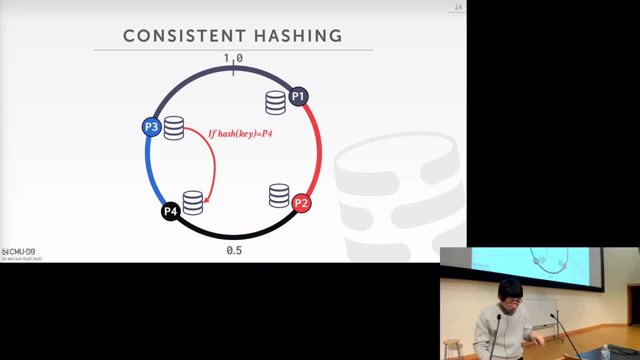 so what do we need to do? is that you only need to move this data, so you only need to go to this node, P 3- right, because originally all the data here belongs to P3, right, So you only need to go through P3 and then read every single record and compute their hash value. 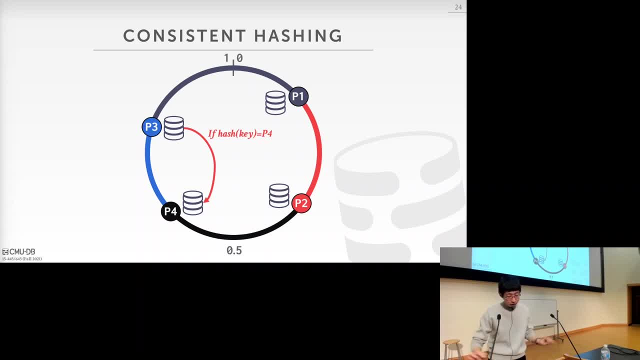 and then if the new hash value land in the region between P2 and P4, then you just move that data around instead of touching many other nodes and move everything around right. So in this case this would actually very localize the movement after you add a new node And similarly. 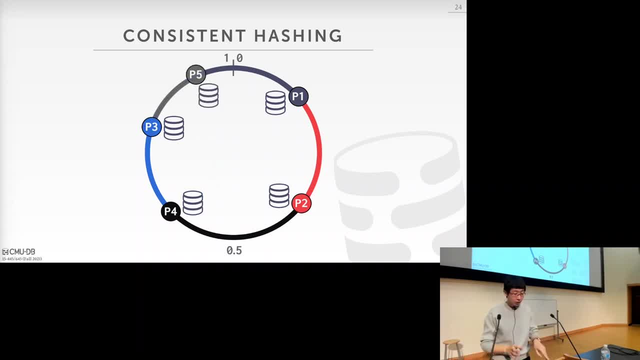 right. say, here you add a new node, node 5, and then you would just only look at the original data reside on node 1 and then move that portion of data land to the new region, belong to P5, to the new node. And similarly, if you add a node 6 here, 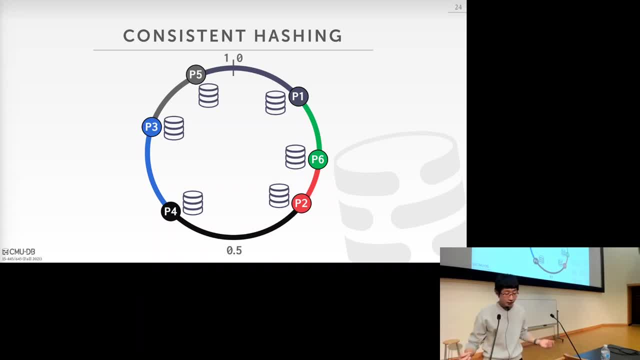 you could do it that way right. So with this consistent hashing, even though you are keep adding node, but you can always look at a region that is like the biggest on the ring and trying to move data from the current node that has the potentially the most number of records to the new node and localize the movement that way right. 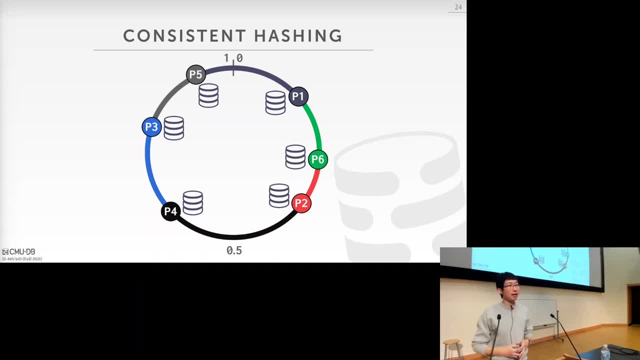 That would be actually be much simpler and much more efficient than moving all the data around. when you just simply mod the number of nodes in your cluster, That make sense, Okay, nice, nice. So one additional problem- if real I want to talk a little bit here- is that 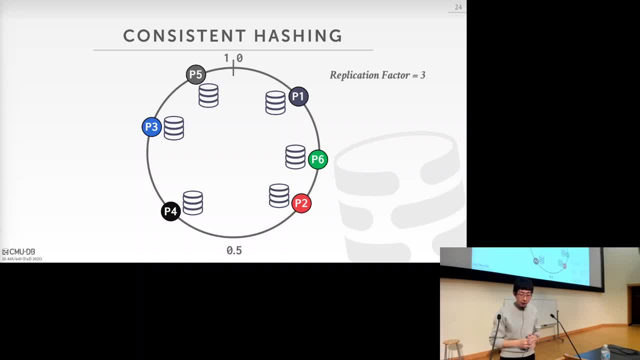 we'll get to the details in the next class when we talk about concurrency control. but the additional interesting property with this consistent hashing is that in distributed database system world, oftentimes you will actually be replicating your data as well. right, Because I mean now you have the luxury of 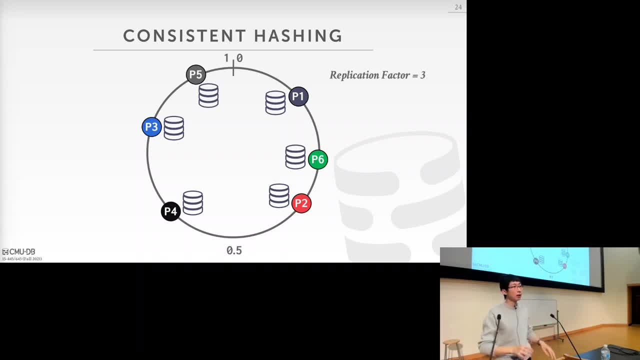 putting data on different machines in different data centers, different regions, oftentimes right. In most cases, users will actually choose to replicate a particular partition of the data to several different nodes so that if one node down, you have the copy of data immediately available on our 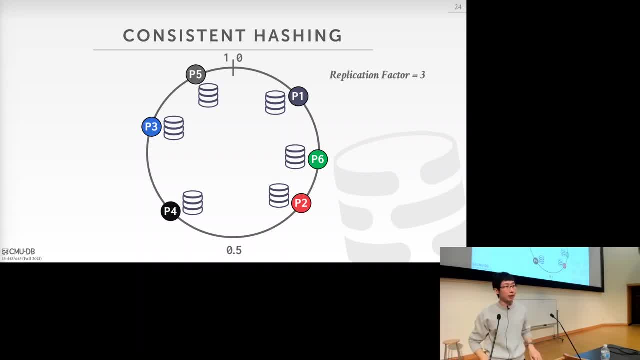 nodes so that you can read that from the other copies as well. right, So in this consistent hashing scenario or algorithm, it's very easy to handle that as well. Say you have, we want to have a replication factor of three. then in this consistent hashing, for example, your data land in p1, then 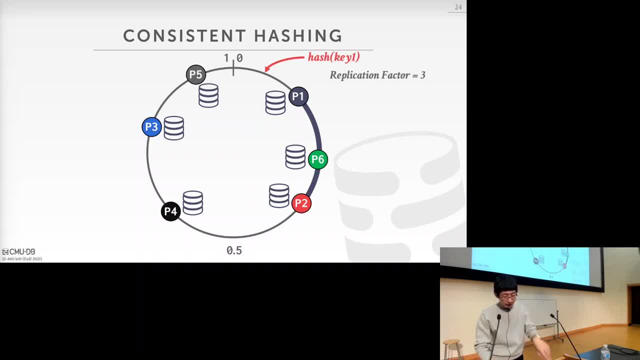 right, for example here: right, if your data land in p1, then besides just looking at the data immediately after the roundup, you can actually copy the data in these three different locations right next to p1,. right, It will be your p1, p2, p6, and p2, and then you can copy this. 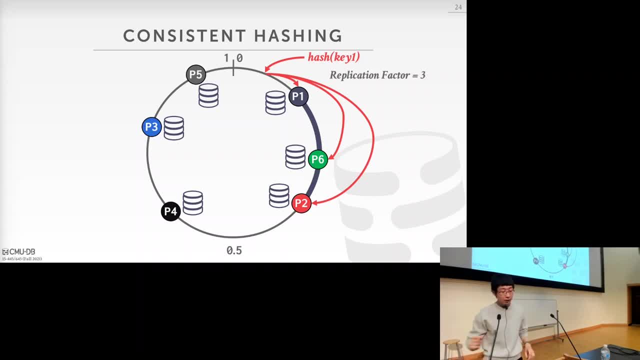 data with the key 1 to these three different consecutive locations on this ring and then, every time the query arrives, you can choose to read this data from one of the copies. okay, So that's what I mean. if one node goes down, then you can also know read data from other copies. 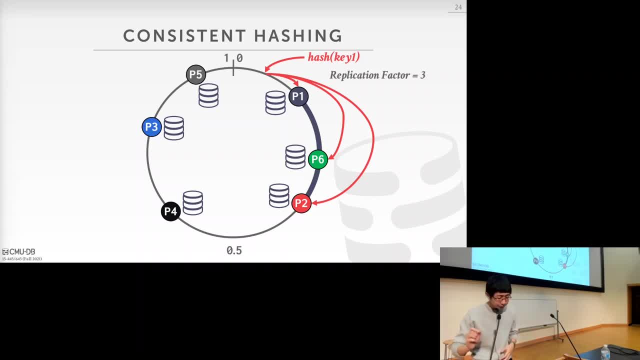 So this will actually be very convenient to handle that case as well. And here I actually want to give you guys a heads up about a consistency issue that also involved in this replication scenario. Again, we'll talk about more details later, but then remember, 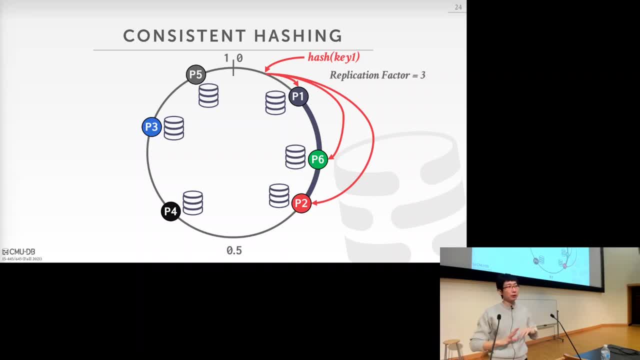 I think it's like last week or two weeks before. when we talk about the ACID property, right, We talk about this consistency property. At that time, I said that the property of consistency would actually matter a bit more in a distributed scenario than a single node scenario, right? 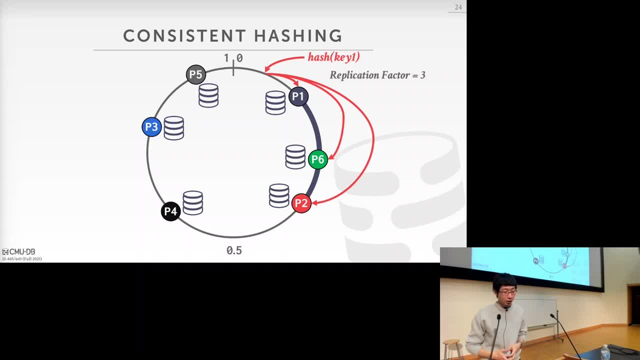 So in this case exactly- I mean, it's like examples of that consistency issue. See, here I have three replications that all have the copy of this data right- Then every time if I want to update this key right, then I have actually two different choices here, right? 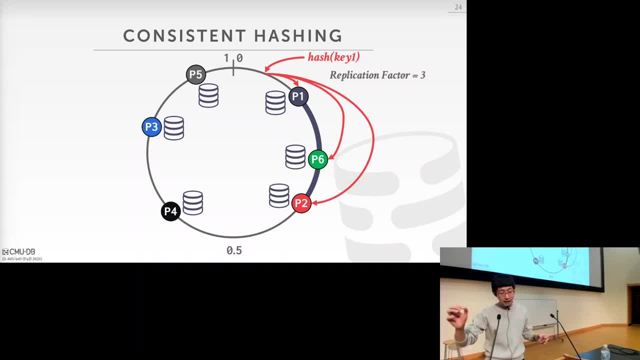 The first choice would be that I broadcast this update for all those three different locations- p1,, p6, and p2, and then I wait until all the three partitions to come back and say that hey, I successfully write this record to my partition. You wait for everything to finish and then you come back to the client, right? 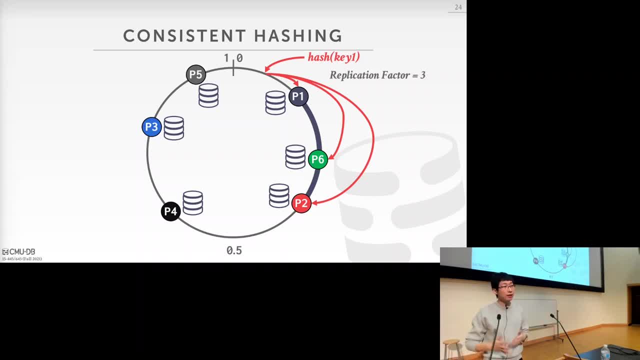 Tell the client that your query has committed, Then obviously this would be very consistent. So actually in a consistency terminology this would be called a strong consistency. But then obviously the problem is that before you only need to write one partition. 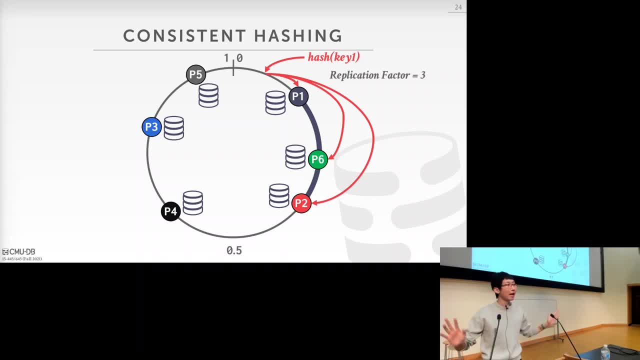 but now you need to write to a three different partition and you have to wait for everything to finish right. If there's a straggler somehow, there's a network delay happening on one partition, or the disk has just had a slow write on one partition, then your whole query or transaction would be stalled, right. 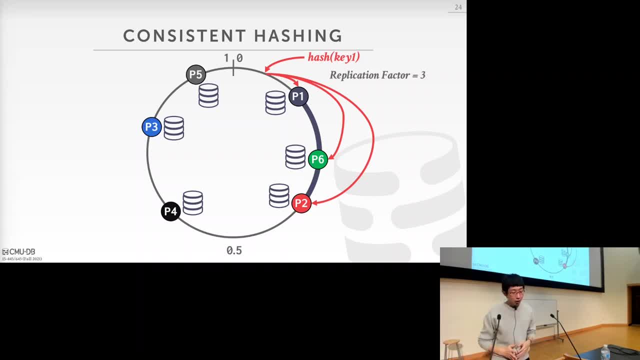 So there could be a little bit of performance issue. And then another choice would actually be that every time you want to write- let's say to this key 1,, you can still issue writes to all the three partitions, but then you only respond to your client when the first partition returns right. 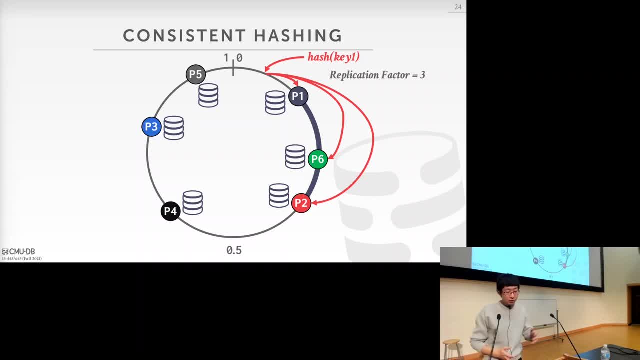 Say the partition 1 is very fast, then you just tell your client you have already successfully finished the partition, finished this query. as long as p1 returns right, Say I have committed, Then I mean, you're just assuming that at some point 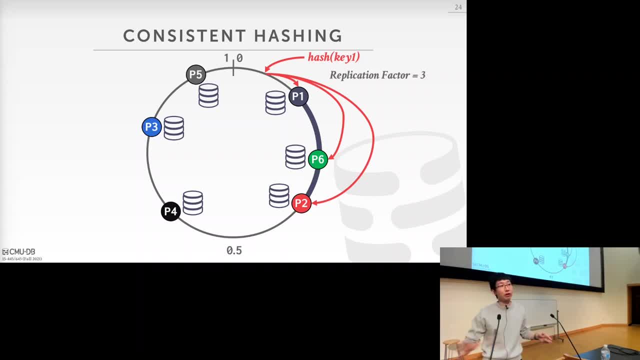 this writes to p6, and p2 will finish right and reflect the correct value. So this would actually be called eventual consistency. It would actually be a much weaker consistency level, as you can imagine, than the strong consistency that I've mentioned in the first example. 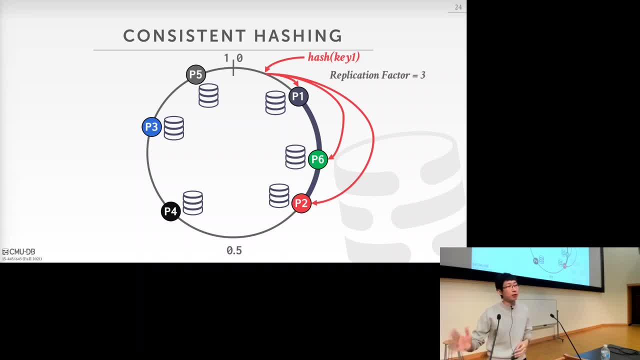 But then of course this is potentially faster, but then this would have the issue of you know, but then of course this is potentially faster, but then this would have the issue of you know, before the writes on p6 and p2 finish, then the value of p2 and p6 could be outdated, right? 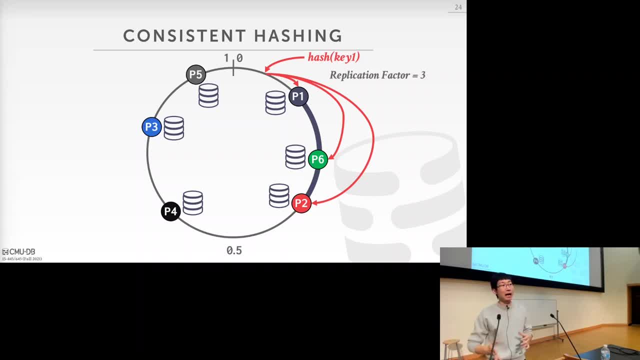 before the writes on p6 and p2 finish, then the value of p2 and p6 could be outdated, right? So some transactions, if they are reading a value from p1, it would read a new value. If they read a value from p2 and p6, would be an old value, right? 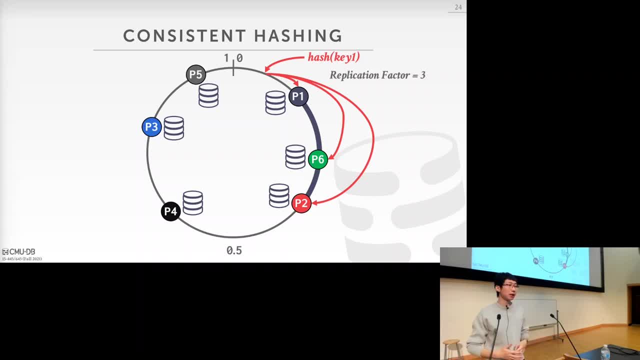 So it's not exactly consistent. So, depending on application right, depending on how fast or how strict your application requires the transaction semantics is, you may choose either strong or eventual consistency. you may choose either strong or eventual consistency. eventual consistency. 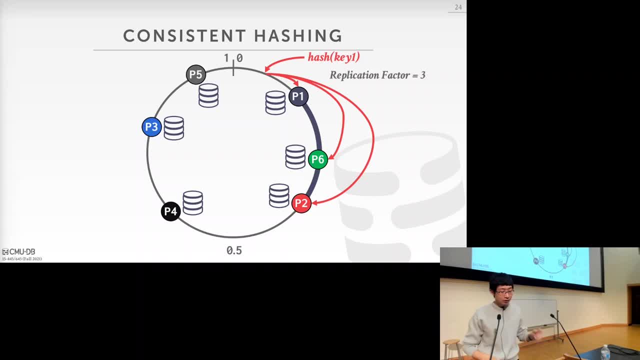 Again, we'll talk about congruency control in distribution scenario later and just give you a heads up related to this acid property that I mentioned earlier. And also this consistency issue is actually not specific to consistent hashing. If you use normal hashing, if you use range partitioning, 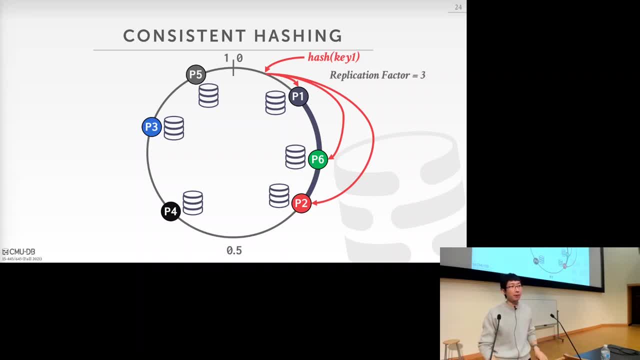 you will also be dealing with this consistency issue as well. All right, So just an example for that. So, like I mentioned this, consistently hashing is actually a very good way to handle a partitioning problem in distributed database, And there are also many systems that are using this. 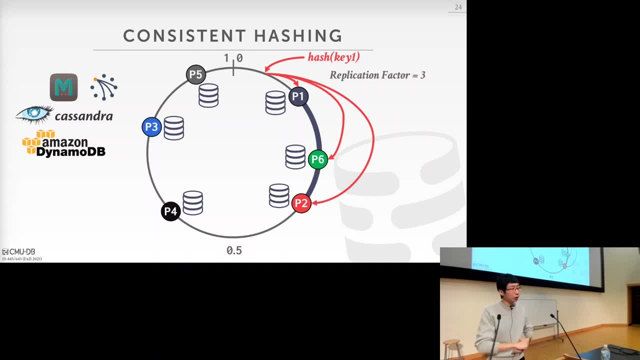 For example, the Amazon DynamoDB, I think is actually the first notable system that used this, and they have a paper on that. And then later on, there's this system called Cassandra came from Facebook. also used consistent hashing to handle their distributed database. 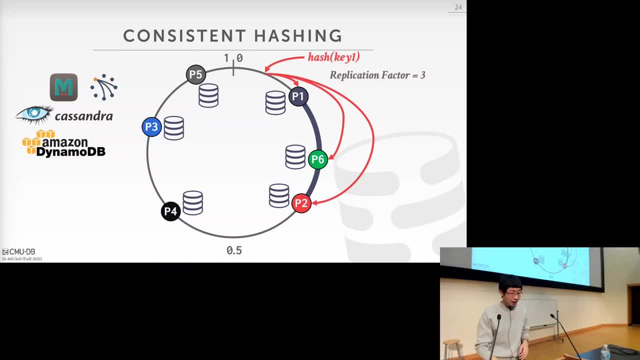 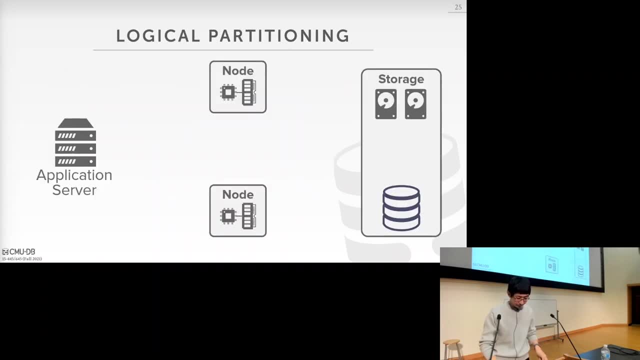 And also there's other newer startup- actually I forgot the name of them, but there are also other newer startups also use this approach as well. All right, So we talk about this consistent hashing. Now I want to give you a few examples. 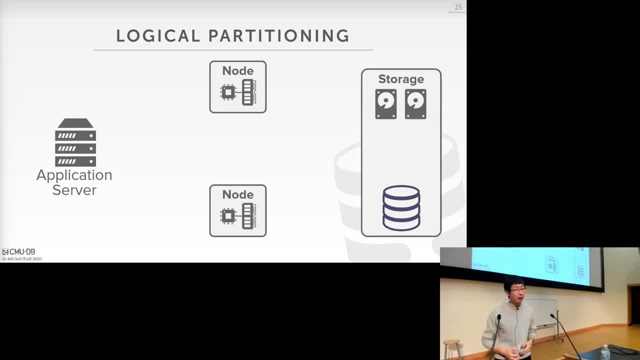 of this logical and physical partitioning. Like I mentioned earlier, just by partitioning the data, it doesn't necessarily mean that the data has to be on different machines, right? Especially in a logical partitioning scenario which would be very common in the shared nothing, sorry, 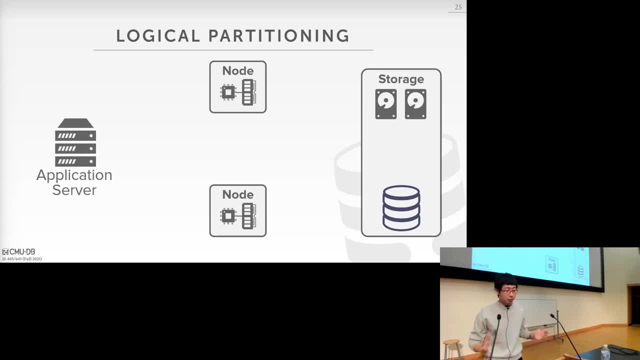 very common in the shared disk scenario. different nodes could just be responsible for handling the queries of different partition, but all the data could be all in this shared disk space, right? So here, for example, I have a shared disk architecture. See that this shared storage space has four records. 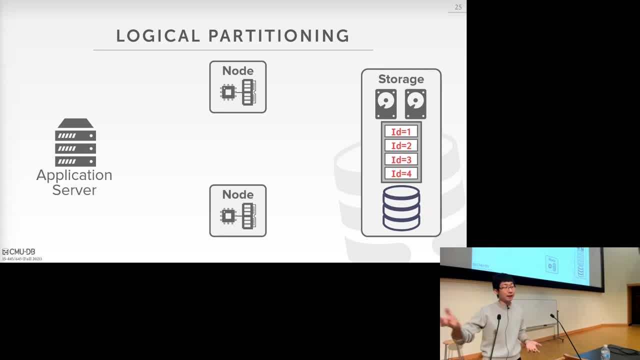 one, two, three, four, and because it's like a managed, for example, managed by Amazon S3 in this shared architecture, I don't really care which machine each of these records is on right, So what I do care is that for different nodes, 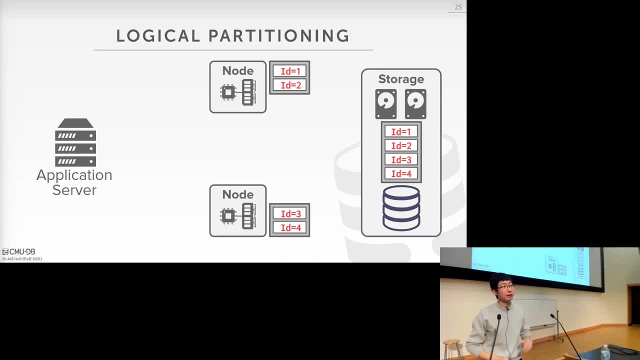 they are going to be responsible, for example, for different partition of data right. So here, for example, in node one, it will be responsible for ID one and two, and then if the application server sends a query to access tuple with ID one, it will go to node one right. 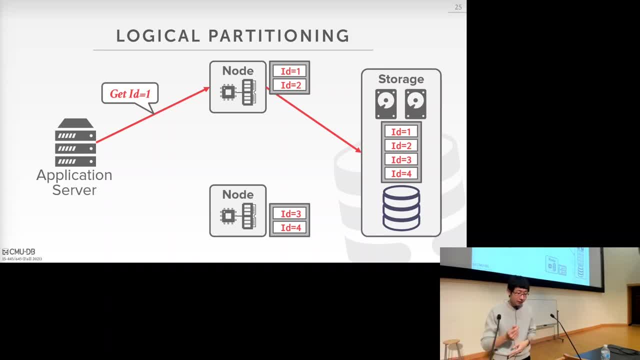 And then it will just go to this shared disk space to get this record with ID one from this unified interface. Similarly, if a node want to get access to ID equals to three, it will go to the second node and get access there, right? 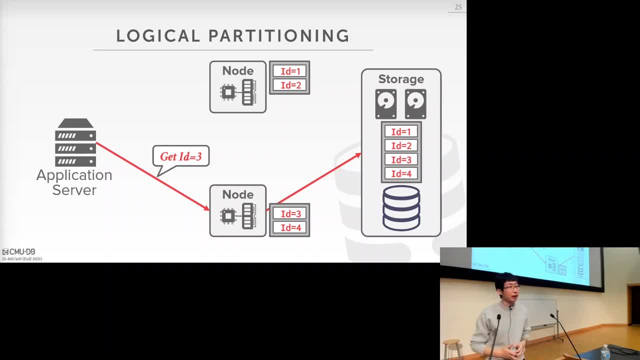 Again, different nodes. I mean it will be better for load balancing reason right. It will also be better for the consistency handling when the different nodes are responsible for different specific records. but at the end of the day everything will go to this shared space. 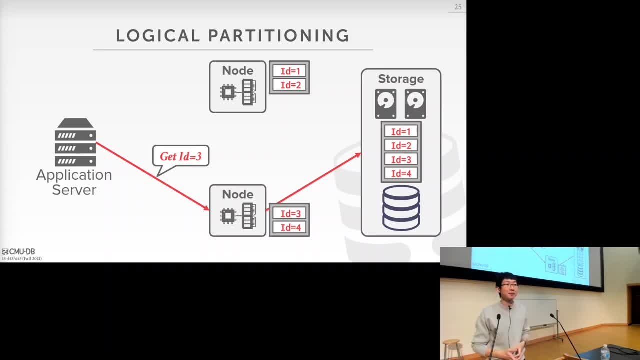 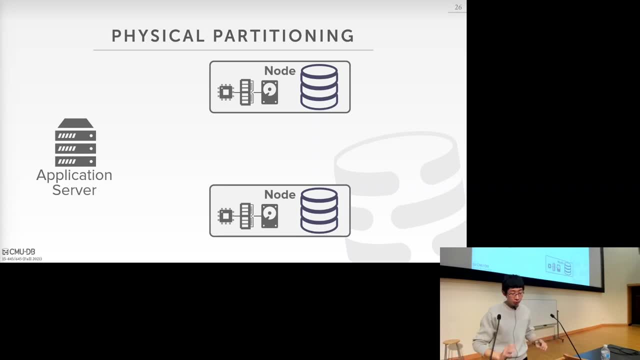 which may or may not put records on the same disk, Make sense. Okay, Then the different example right on the country of that would be physical partitioning right. That would be more common in the shared nothing scenario where you actually would have. 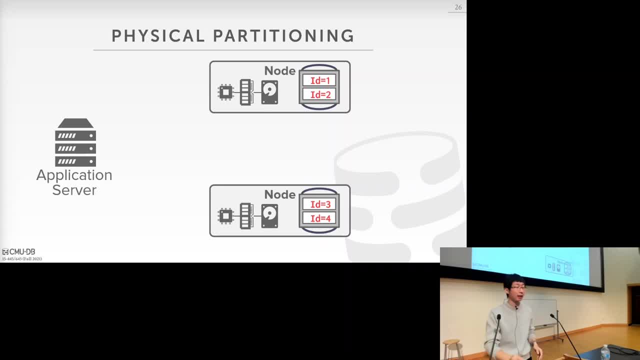 it would be directly locating data on the specific disk right Local to a specific node right, See here. for example, the first node can have a high ID one and two. the second node can have ID three and four right. 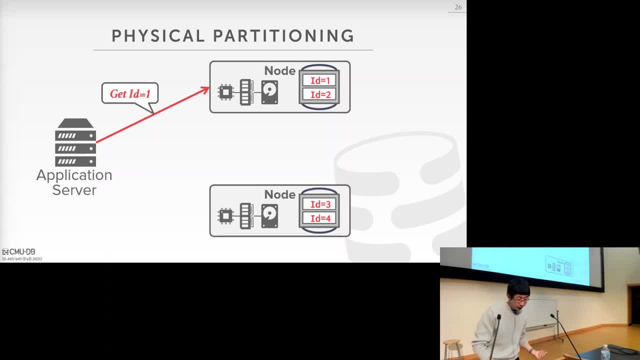 And this case again similar to, I mean the other example. if you have a request that want ID equals to one, want tuple with ID equals to one, you go to the first node. and then you have a query or request that want ID equals to three, you will go to the second node. 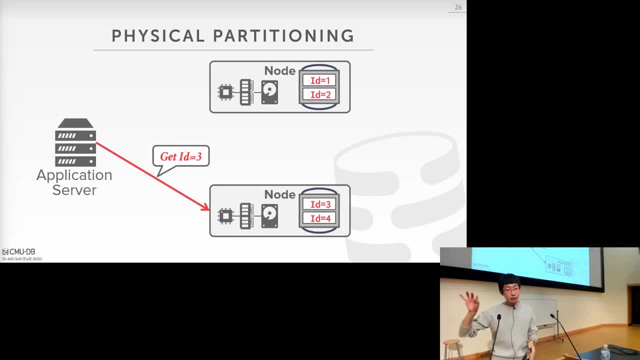 right, And in this case you actually go to the specific node and access the record local to the first node right locally on a local disk. I mean on that machine right, Which I mean again if a transaction only access. 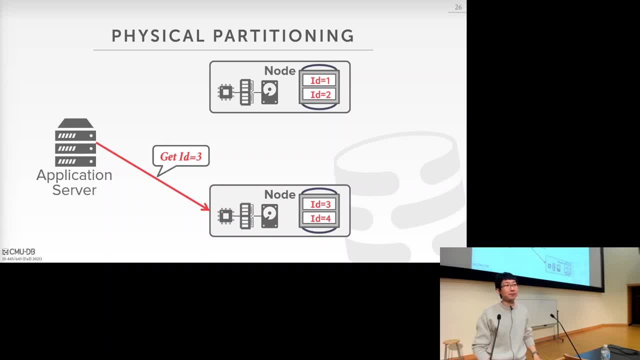 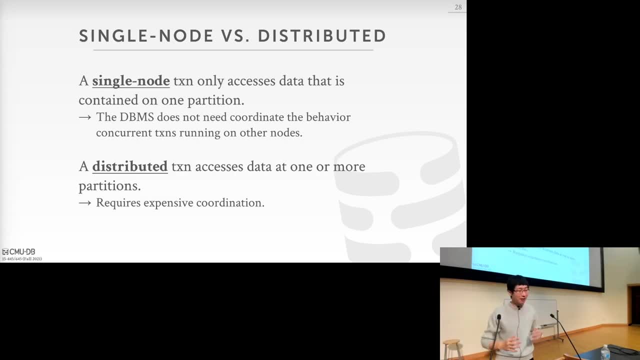 that record would potentially be faster. All right, Okay, So that's that, but that's when. all the example. probably one thing: you have noticed that in all the examples I showed earlier, all the transactions only access data on a single node. 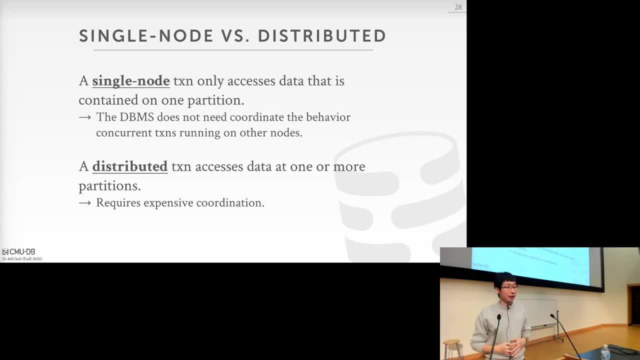 right and, like I mentioned, in that case maybe a shared nothing architecture would potentially be better because everything is local right. But then, but for those kind of transactions they will be called a single node transaction right Essentially means that all the data, a transaction. 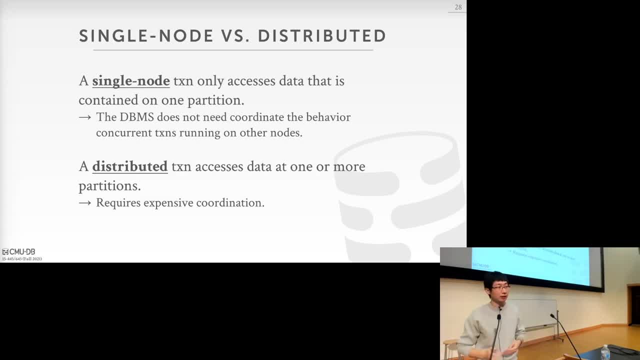 needs to read or currently needs to read will be accessing to a disk locally to that node. okay, But then in practice often cases- right, you, it's not that ideal right- Sometimes you just have to read the data that is not on your specific partition, right. 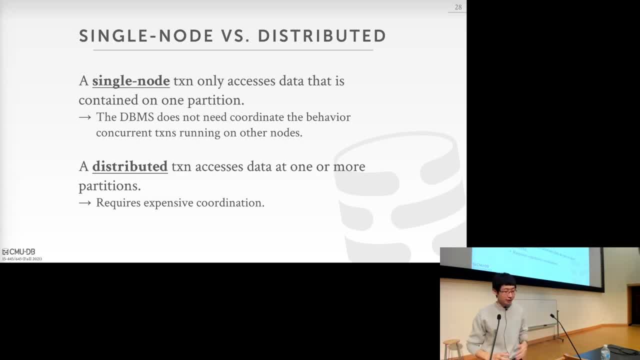 That scenario would be called a distributed transaction. And then in that scenario, when a transaction- I mean a query by itself- needs to, either would be like one single query or multiple query, doesn't really matter right. But when a transaction needs to access data, 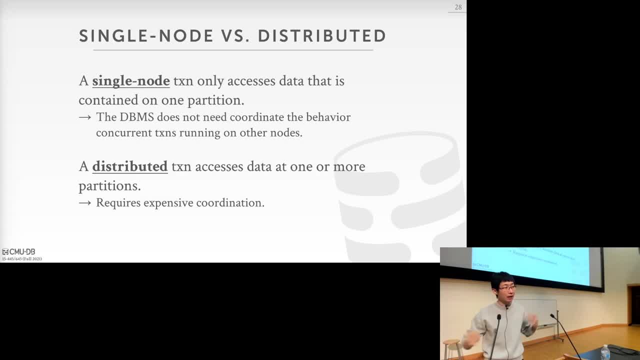 across different partitions or different nodes in your cluster, then this would actually be a very, very expensive and require expensive coordination. Okay, And that's what we are going to talk about next, about this coordination of distributed transaction. Again, I mean how? 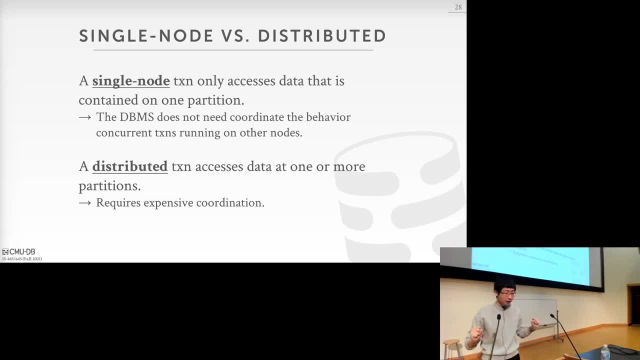 kind of what we think about this is that if all the transactions would be single node, then the distributed database would actually be very easy. right, because all you need to do is that you partition the data on different machines and figure out which data is on which machine. 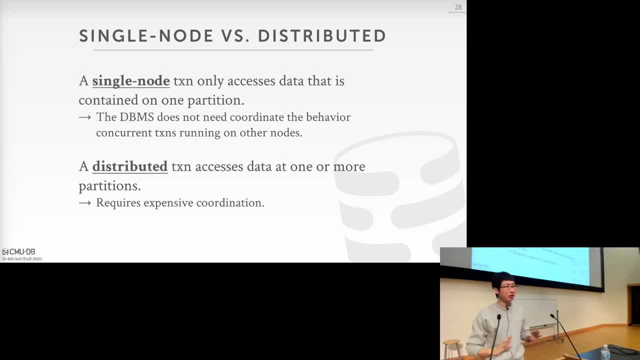 then you will be done right. So if you only have a single node transaction, things would be very easy. So what would be challenging with distributed database would exactly be this distributed transaction, when you actually need to access data on different machines and lots of coordination needs to happen. all right, 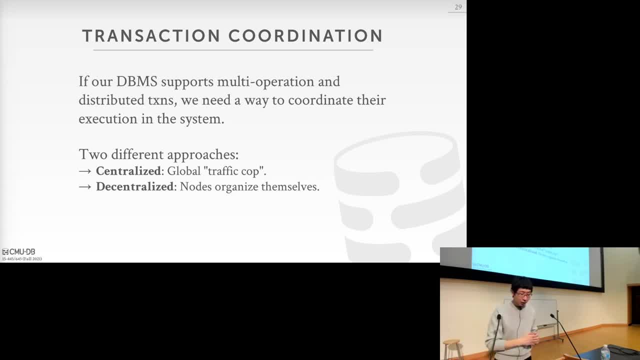 Okay, So at high level there would actually be two different approaches to handle these distributed transactions, right? So one would be called a centralized approach- Essentially you can think of that- just a centralized, similar to the Mongo architecture I mentioned earlier, right? 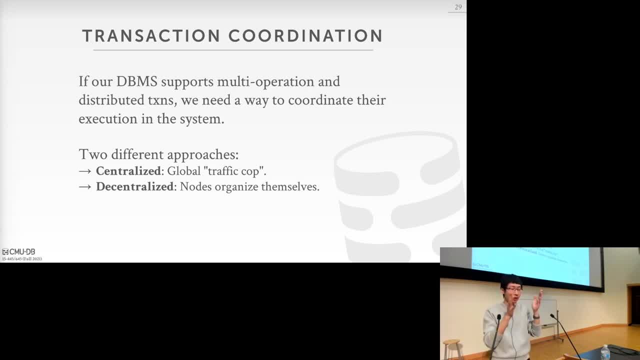 There would be like a central config server handling the I mean that have information about location of data. Here the centralized approach, you have a global I mean server or a traffic corp that will actually know the status of all the transactions. 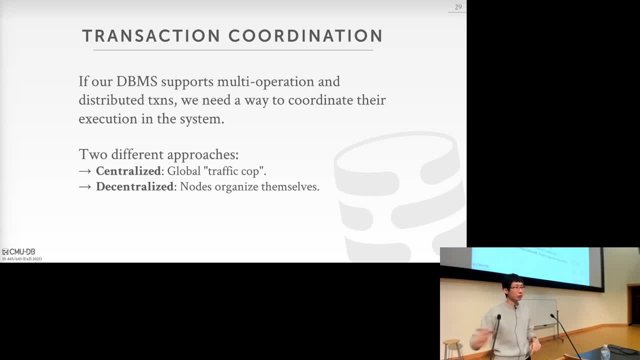 and which transaction is accessing which data, on which node, which transaction locks which, et cetera, and then do all coordination and law and then resolving all the concurrent sequential issues and then, every time the transaction was to commit the centralized node or traffic corp. 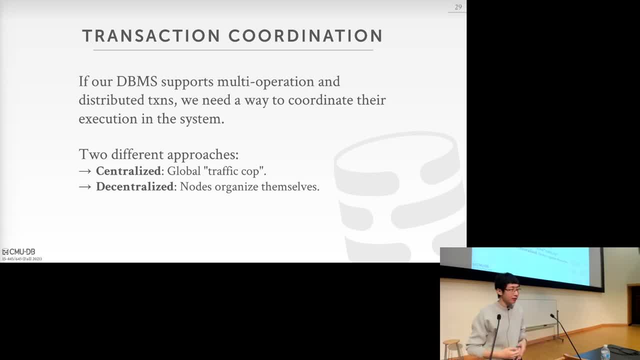 needs to make the decision. Alright, Then I mean kind of obvious. the country approach will be called the decentralized approach, right Where different nodes actually just organizes themselves. So every node will actually be responsible for coordinating whether a transaction should be committing or not. 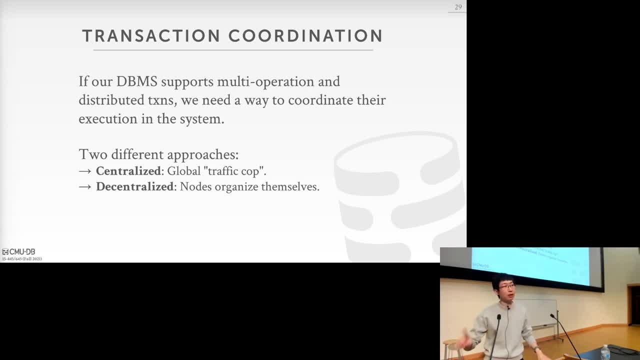 but, at the end of the day, right, even though it's decentralized, one specific node needs to be responsible for a specific transaction that it should commit, or not, right? It's just besides a kind of like a heterogeneous, centralized approach. every node would has the ability. 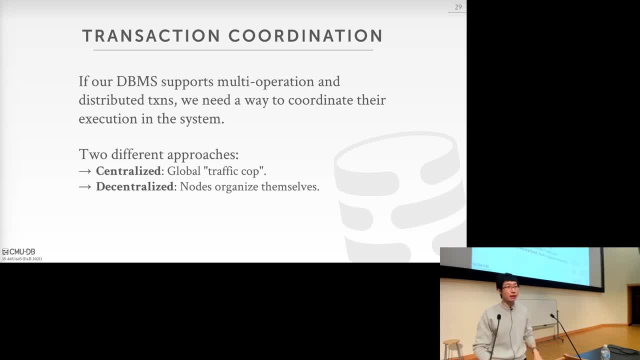 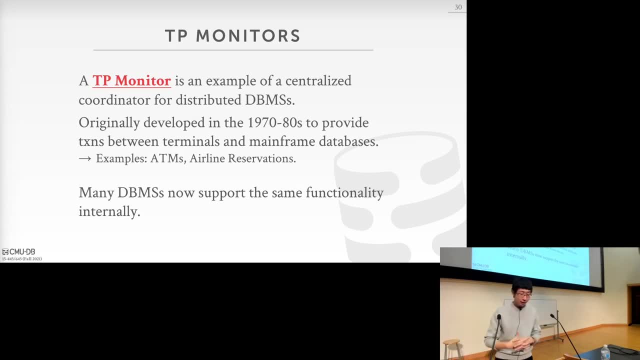 to decide which transaction commit or not, right? That would be called decentralized approach, right? So the very first centralized approach example of this will be something called the TP monitors. actually dates way back to 70s or 90s, right? 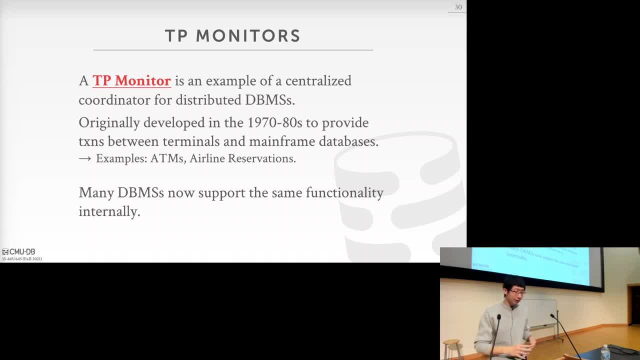 I think at that time it's called a telecom monitor, but nowadays people actually refer to them as a transaction processing monitor, And actually at that time there's even no like mature implementation of distributed database system yet, right So? but I mean there are many use cases. 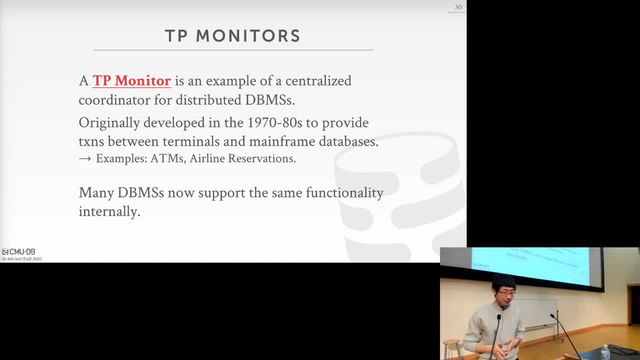 that people need distributed functionality of distributed database. So what people do at that time is that many people, for example, for ATMs or airline reservations- right, you have a different machines or different- sorry, different- databases that are holding all the records. 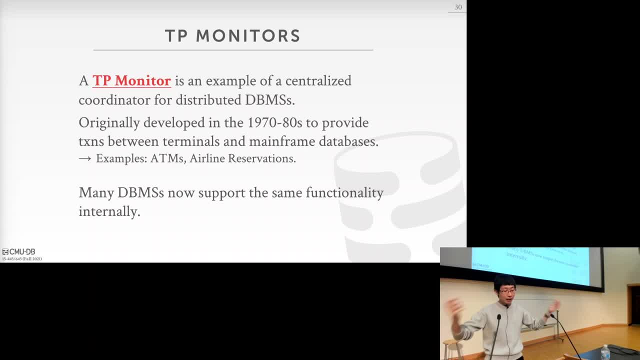 or the tickets- right, airline tickets- but then you have different clients want to access them at the same time. you actually have sort of a middleware, if you will right. I mean sits between that coordinate the execution of these different transactions. 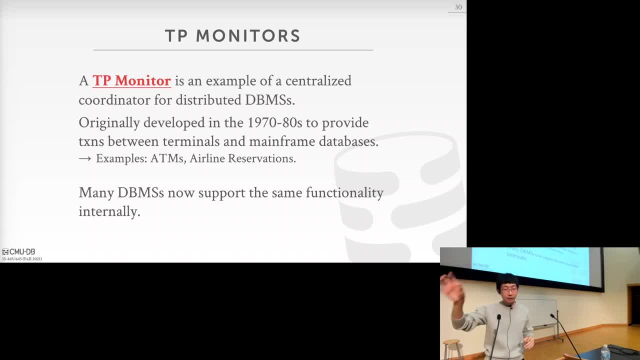 to different database servers. right Again, for each database server it has its own concurrency control algorithm. right, To make sure that access to that specific database is ACID. right, it's like protected by a concurrency control algorithm, But then for different clients that may access records. 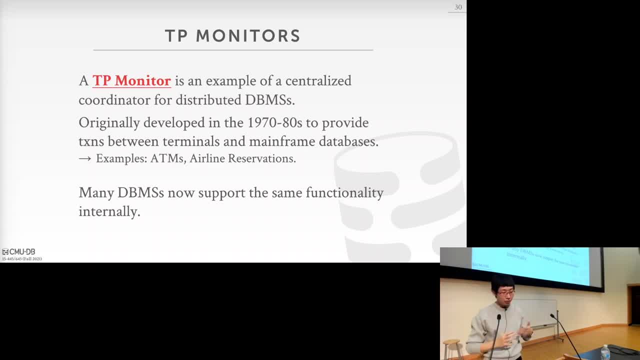 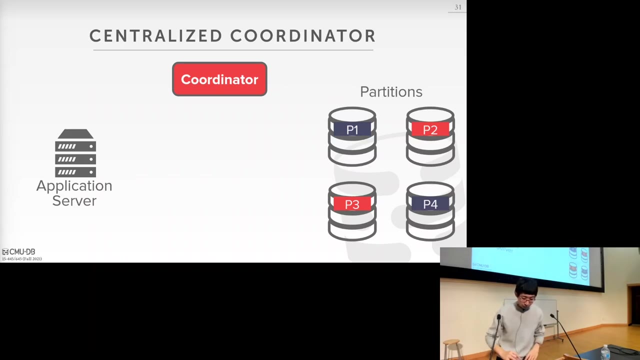 to different databases right located potentially on different machines. they need to go to this centralized transaction processing monitor and to resolve which record is on which, which transaction needs to be locked and then how to handle all the conflicts correctly, right? So I'll give you an example for this right. 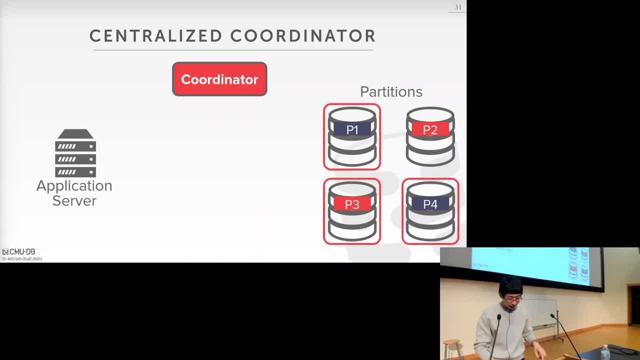 Say I have an application server here, right. And then when the application server needs to access the data, say it needs to access data on these three different partitions, right, it actually needs to send this centralized coordinator that, hey, this query needs to access this data. 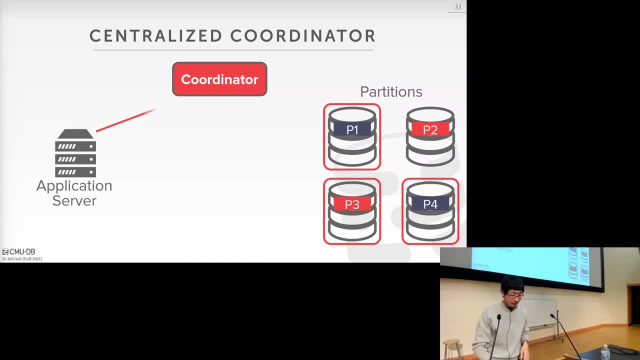 on three different partitions on this cluster of databases, right, and then what this coordinator will do is that this coordinator will actually need to lock. well, it'll have a lock table and it'll need to put a lock on these three different partitions of data. right. 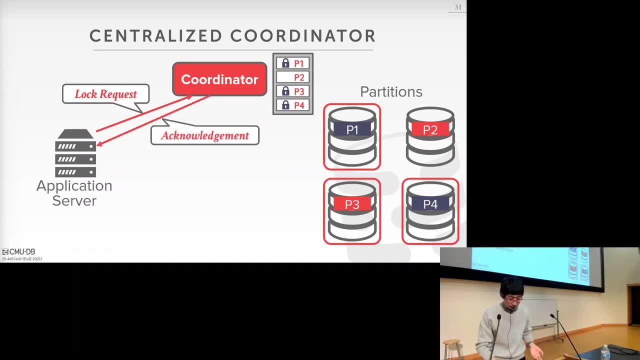 And then only after that- this I mean it can send back the acknowledgement to the client and then client can go ahead and modify the content, or read and write the content of these three different partitions And in the meantime, depending on whether you are holding. 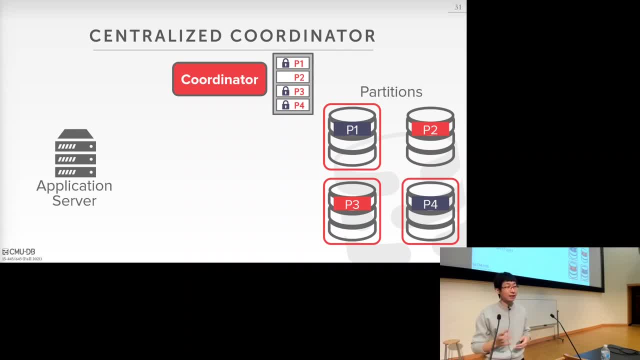 read lock or write lock. other transactions may not be able to access data on these different partitions. Again, this is like in your system, right? If you do this inside the distributed database system, it could be finer grain at the table level. 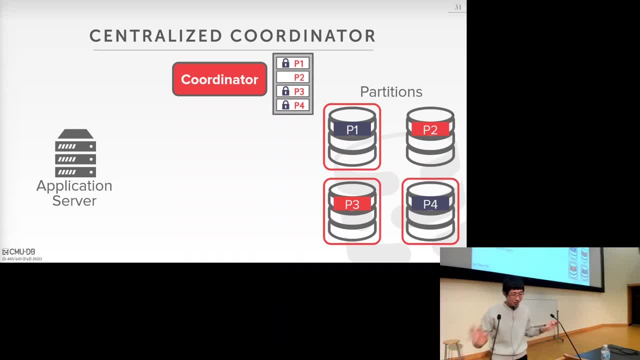 table level, et cetera. But then back into the old days. right with this centralized controller, it would be at partition level. You had to lock the whole thing right And then you can- yeah, you can- access all these different records. 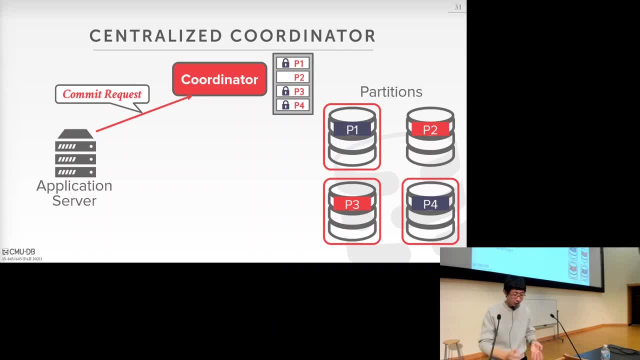 So now see that this transaction or the application finished this query and then wants to commit right. So what do you need to do? It actually needs to go to every single of these, these like machines or partitions. right To ask the machine. hey. 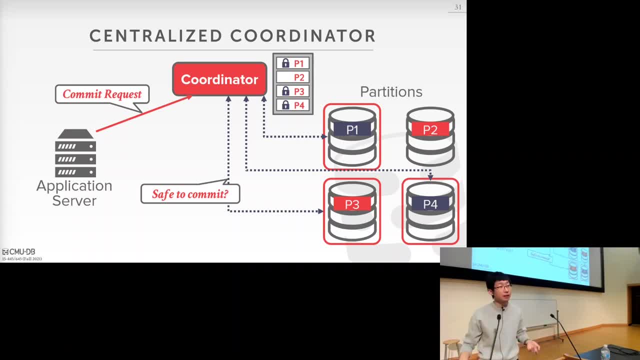 have you finished all your operation? Have you finished all the writes? Am I ready to commit right now? right, And if every transaction was ready to commit, then it comes back to this coordinator, sends the acknowledgement and saying that hey, I can safely commit. 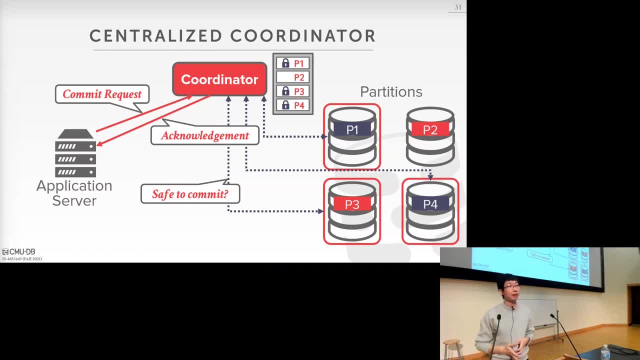 and then I can now release all the logs in my log table. Right, that's how to handle that. this, like in the first implementation, very original idea. And then actually there are systems still be using something similar, similar to that, right. 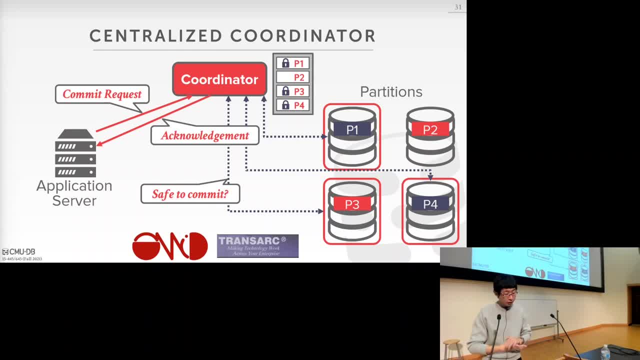 There's actually one, a startup called Transoc, that actually came from CMU, right, Build some sort of a transaction monitor in this fashion And actually again came out very early, but still be used in many systems, right? And then Oracle also has a version of this. 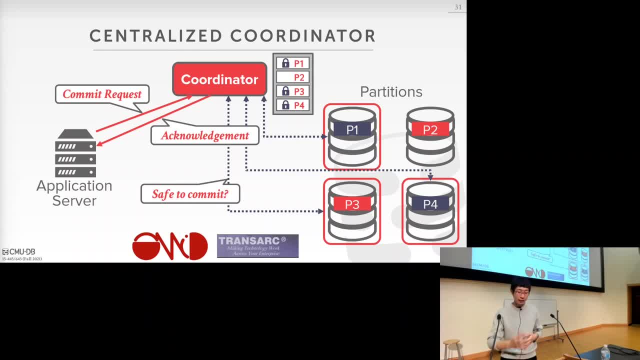 Oracle has also been doing database business for a long time, right, He also has a version of this called Taxido, And there are also this other company called Omid. that is like doing this kind of service, right, But then this kind of like early implementation. 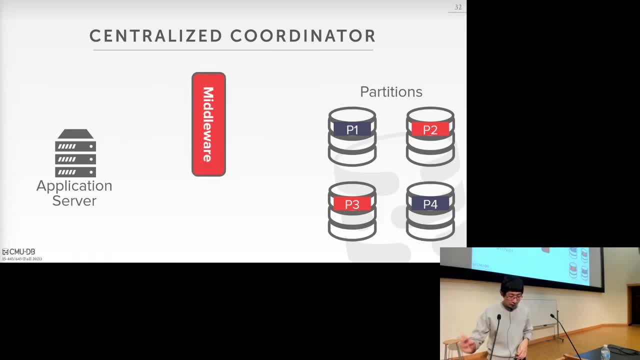 of these distributed transactions. And then what happened a little bit later is that, instead of just a simple coordinator, where- because in the coordinator, like I mentioned this early, this application server actually need to send the log request to the coordinator to log different partitions, right. 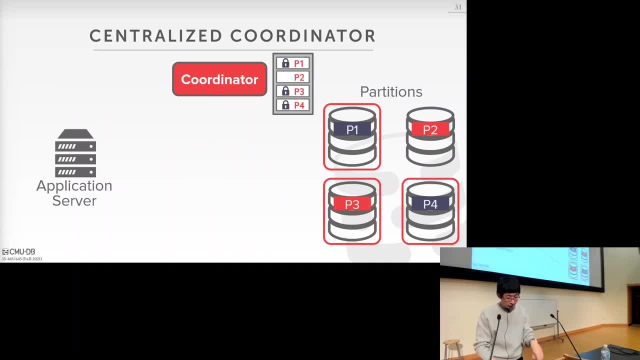 And then when the log finishes, the application server needs to send other like individual request to the partitions right To get all the data back right. This is, like this, very limited. I mean there will still be lots of involvement. 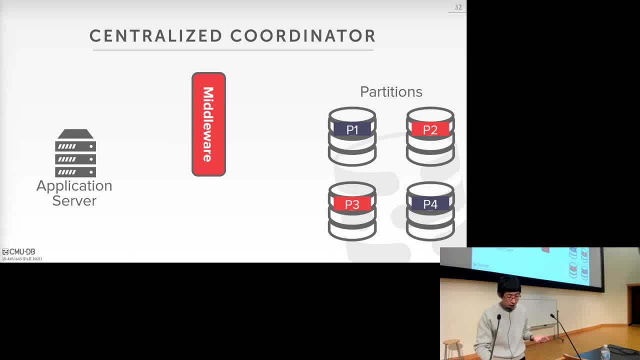 with the application server as well, right? So we later optimization or extension of this approach is that you actually build a middleware that will hide all of those logics, right? So this would actually be used more common in many of the newer systems as well, right? 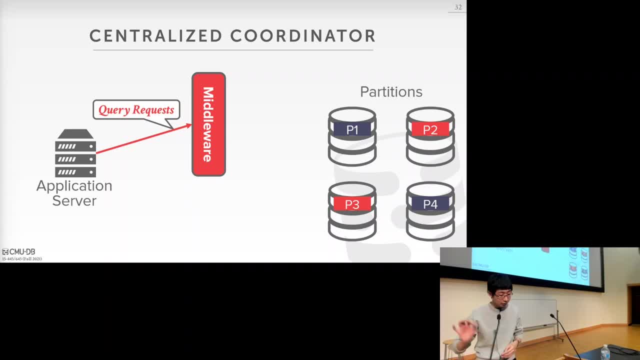 So essentially in this case, when the application server sends the request- I mean distributed database- it doesn't need to know which data is on which machine. it doesn't send log requests, and then it doesn't send individual requests to different server or partitions either, right? 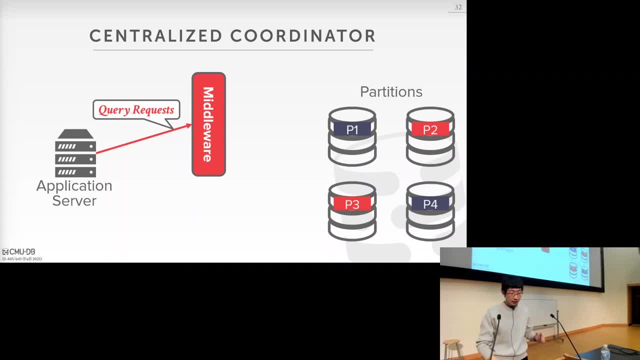 It just sends a single request, just as a single node database, and then inside this middleware it actually maintains all the information of which data is on which partition, etc. And also this middleware is going to be responsible to send log requests or maintain log request. 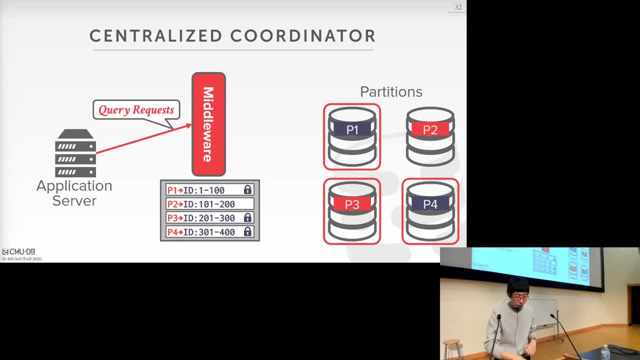 on different partitions, right, And say, in this case again, it needs to log these three different partitions and then this middleware will put this log in its log table, But then there's nothing that this application server needs to do anymore, right? 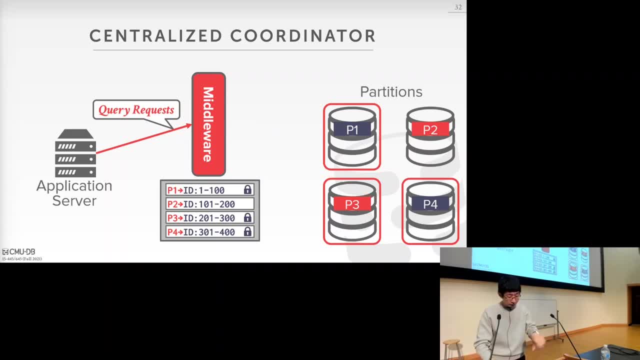 The middleware hides all the details. And after that the middleware will do all the read and update on the application's behalf, right, And then after that, when the application sends the commit request, similarly the middleware will ask, hey, whether each of these partition would be safe to commit. 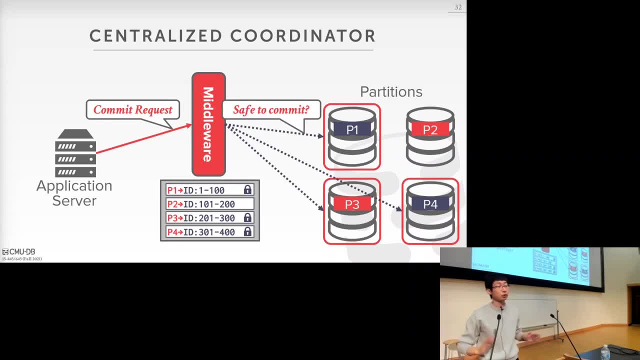 and if yes, it comes back and then commit the transaction right. So this will be kind of like an optimized version right of the original transaction processing monitor approach that would hide many of the details And this, actually this approach will be more common right used in many of the newer systems. 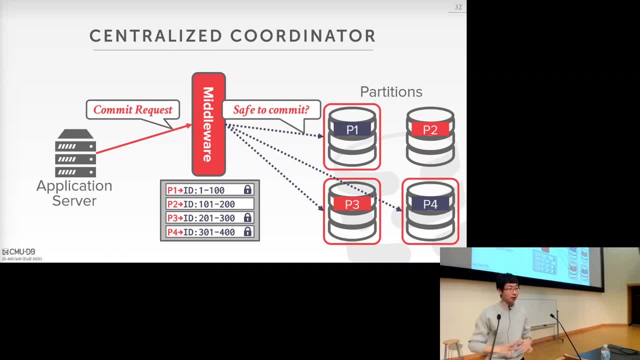 The biggest example of this is like Facebook actually has the largest MySQL cluster on the world that they manage using this approach. So each MySQL would actually just be a normal single node database system we talked about earlier in this class, but then they build this: 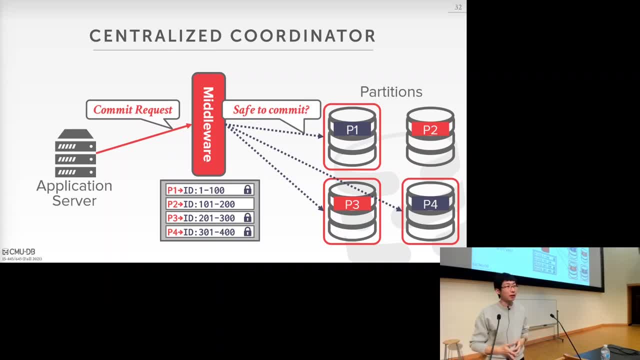 uh, uh, like a function, like a complex middleware that will hide all the details for their MySQL cluster, right? That's actually the largest thing in the world. And then YouTube also has a version of this, also built on MySQL, called Vertease, right? 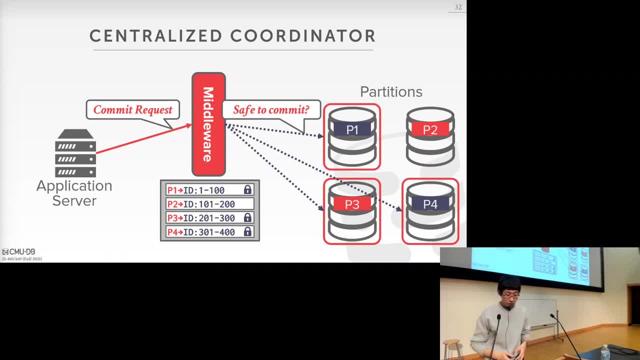 That's also, I mean, used as a middleware approach, And then also Google also- at least Google used to have a version of MySQL service- also use this approach as well. All right, make sense, Cool. So the next approach will be: uh. 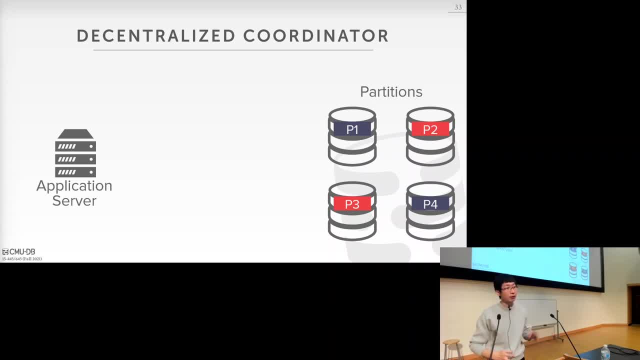 I mean, as I used it here, would be a decentralized coordinator, right, Because that would be, uh, each node would have the ability to commit a transaction. So again, like the similar user here, when a application server sends a begin request, 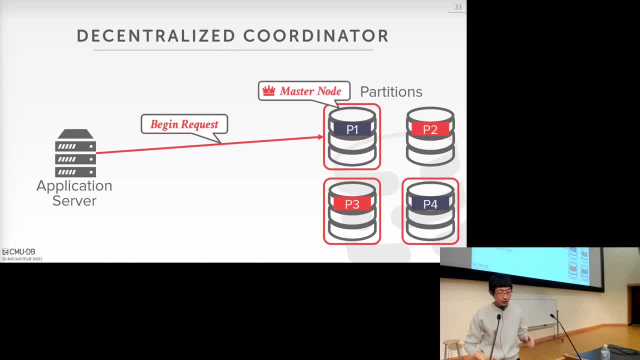 it will actually find a master node for the specific transaction. In this case it could be P1, right, But it also could be P3 and P4, depending on your load balancing right, depending on your routing mechanism, et cetera. 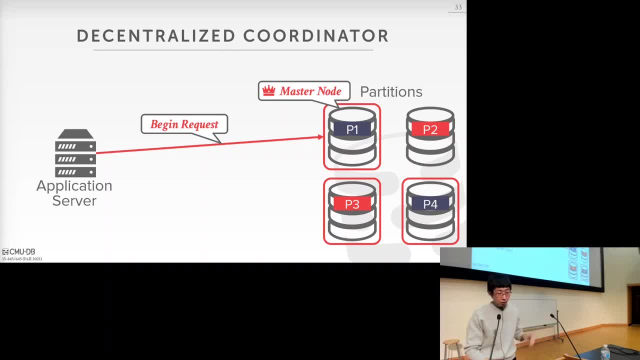 but it's just a peak one master node right And then this master node will be responsible for for all the coordinations of this uh specific transaction right. And then of course this transaction can pick, can have user requests to other nodes, uh P4,, P3, et cetera. 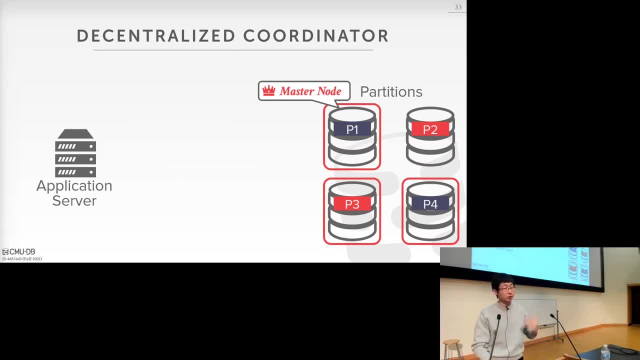 But then this master node would be responsible for recording all those information which, um which partitions this transaction accessed, and then whether it's conflicting with others or not, And then when the transaction wants to commit, this master node would similarly right. 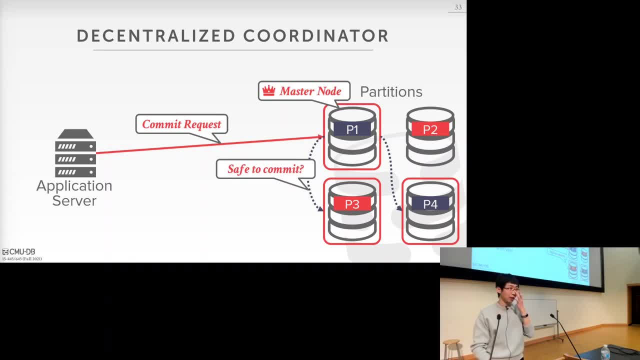 issuing this request relative to commit et cetera, and then get back to the uh, to the client server. But then, just in this case, every node in the cluster would have the ability to handle and commit transactions And of course you also need to co- to do coordination between different nodes now as well, right, 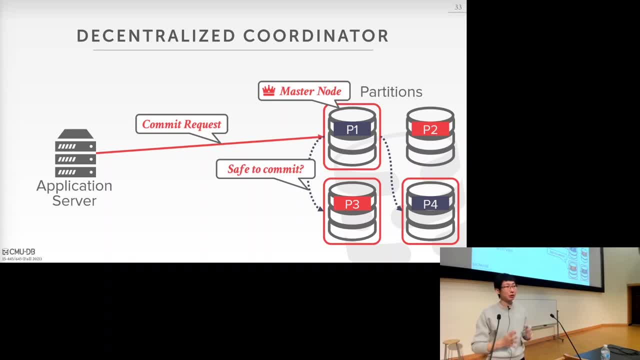 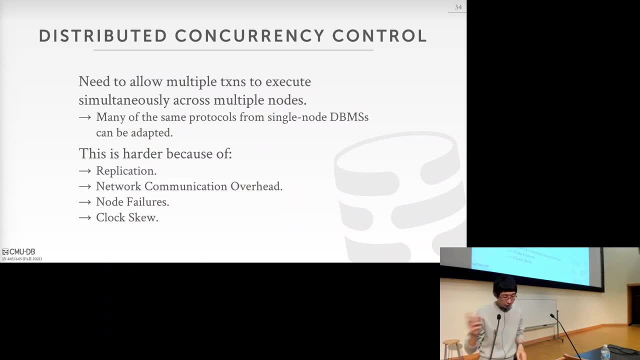 Because when every node can commit, then I mean things can conflict and you have to do coordination, which I'll get to get to next class, all right. So I would just uh, I would have uh like two or three more slides. 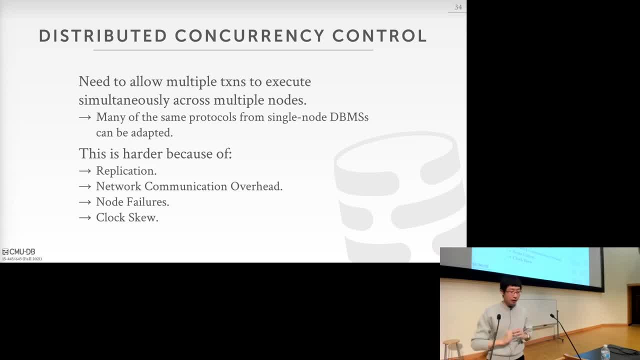 give you just a little bit of small heads up about the distributed concurrency control that we are- we are going to talk about in the next class, right. So, uh, at high level, right, when we are trying to uh control the concurrency of distributed transaction. 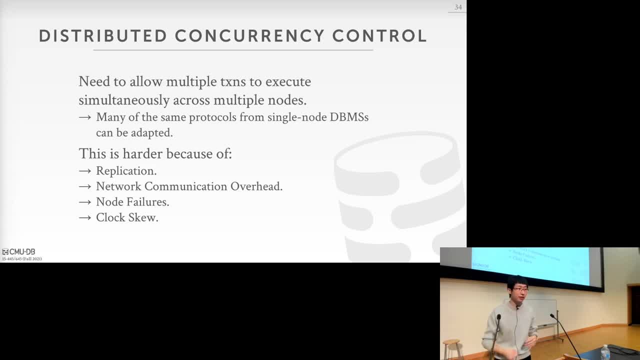 many of the ideas right we used when we talk about a single node transaction will actually be still be up, be able to apply right Either a timestamp ordering, concurrency control, two-phase logging, et cetera. we will actually be applying many of the uh similar mechanisms. 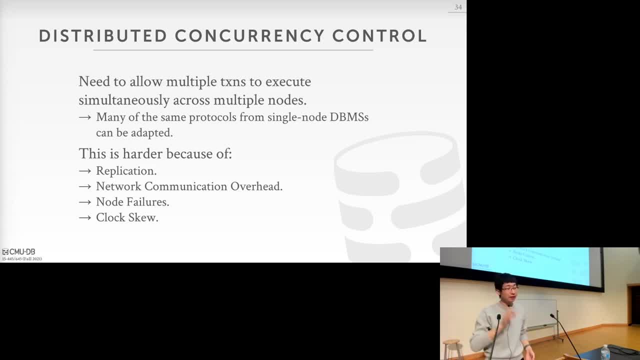 But instead, which is but uh, beyond what those uh mechanism. what we need to do here is that we need some additional steps right To handle the case where, hey, there's the data on a different machine. 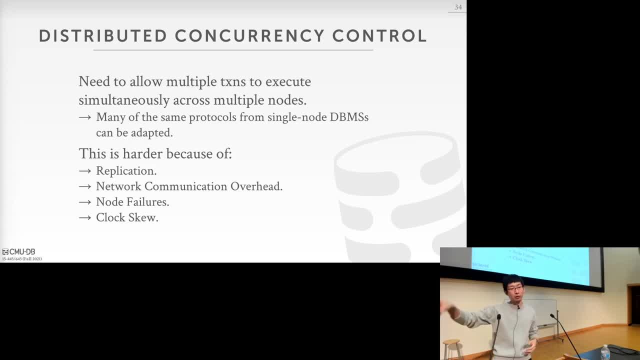 you may put in. you do put a log on a different machine and then sometimes, after you acquire a log on that machine, that machine go down. what do you need to do when the node comes back As as, what if, like, there are different skills? uh, on the log. 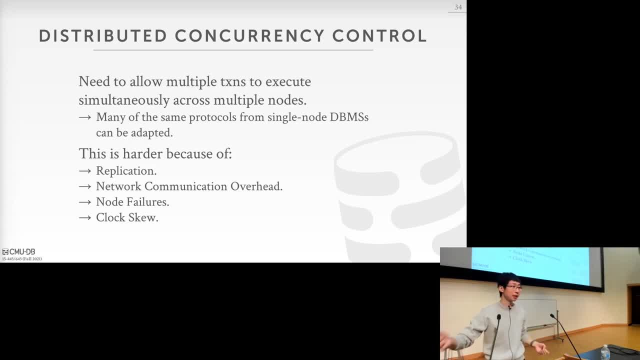 there are skills on the different logs on different machines. for example, if you're using a timestamp ordering, concurrency control- right Again. two-phase logging- uh, optimistic concurrency control, all those things will still apply, it's just there are additional steps and additional scenarios. 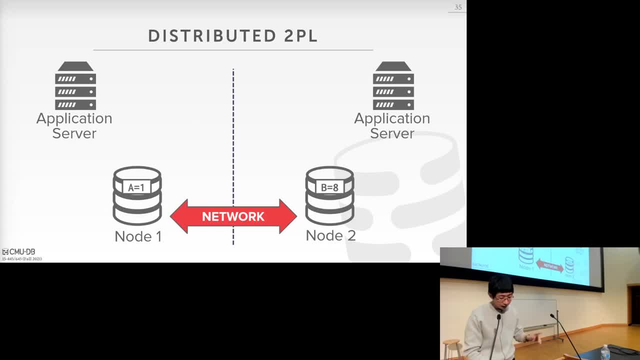 that we need to uh handle in a distributed scenario. right, In a simple example here: right, Like, just like- I think this is the last example in this class- Say, I have uh, just uh, two applications, right? 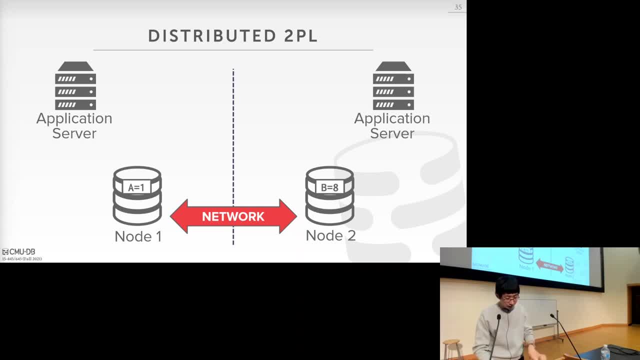 Oh sorry, two application servers, right, And then we have two nodes and then connected by the network. Say this like: uh: one application wants to read record A on this first node, the other, uh application, wants to read uh. 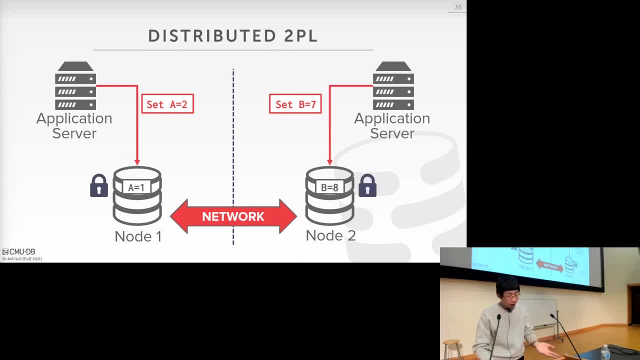 record B on the second node. so far, so good. right, And they, they can log the uh corresponding node or log the uh specific record on the corresponding node. But now what if that uh, we, we encounter a common like a deadlock scenario, right? 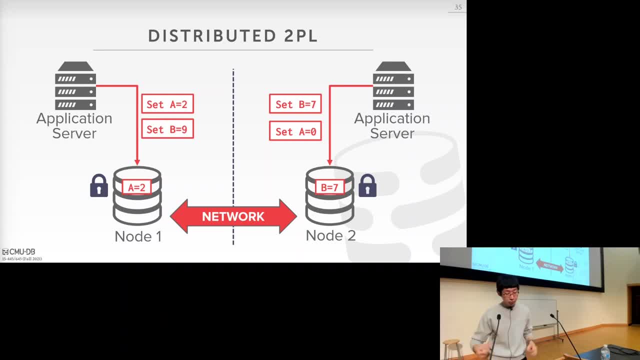 Say, the first application needs to read uh B, the second application needs to read A, right, Then I mean we have a deadlock. we know how to resolve that in a in a single-node scenario, right? Essentially, we are going to construct this waterfall graph. 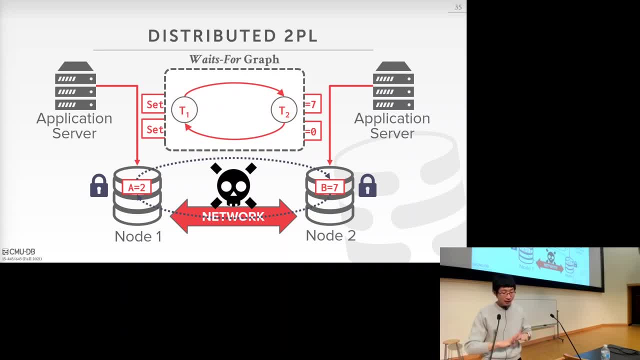 and then break things up. right, I mean, it seems easy. but then in a distributed scenario, right C scenario- we need to consider things like: hey, these different logs may own different machines, right Then how do we coordinate different logs? 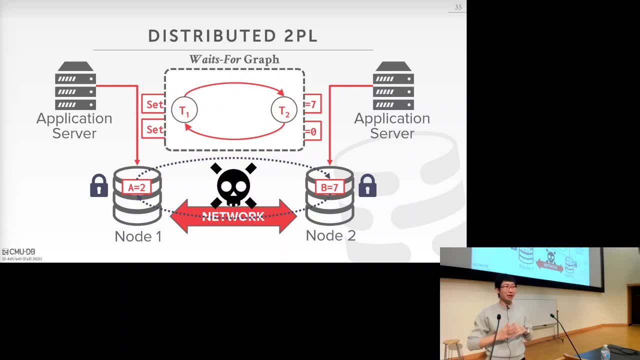 And then also there's maybe network delay on these different machines, right, So network communication may be costly. We don't want to send uh messages and back and forth very frequently- And lastly, uh when one node go down.